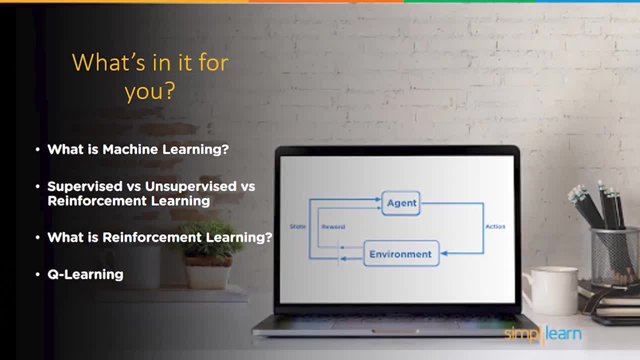 the sub-branches of machine learning which are supervised, unsupervised and reinforcement learning. Following this, we will delve into what is reinforcement learning and finally, we will look at Q-learning, a type of reinforcement learning. But before we begin, don't forget: 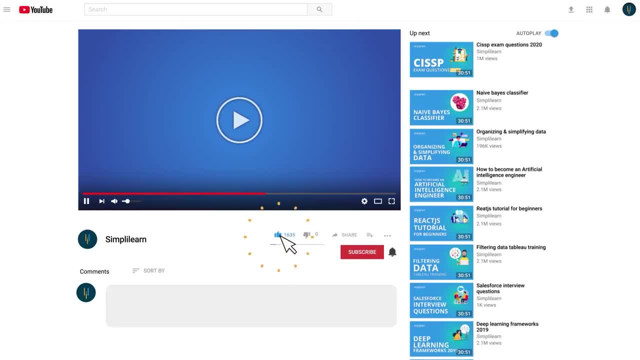 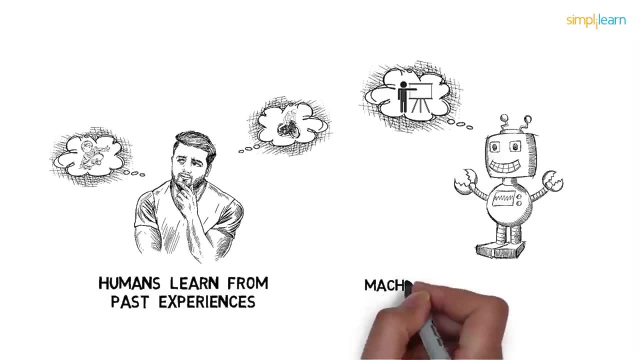 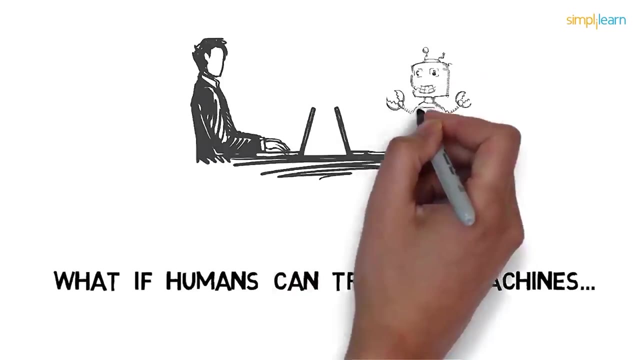 to like this video and subscribe to the YouTube channel and hit the bell icon to never miss an update. We know humans learn from their past experiences and machines follow instructions given by humans. But what if humans can train the machines to learn from their past data and do what? 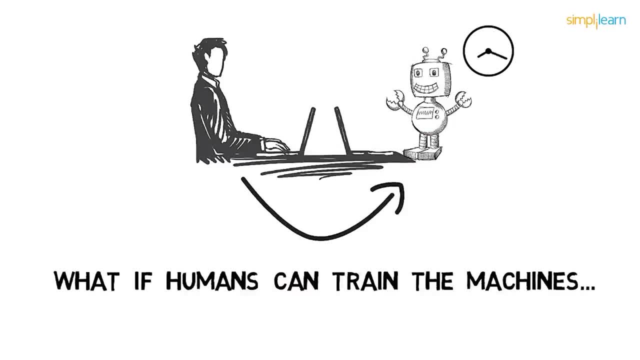 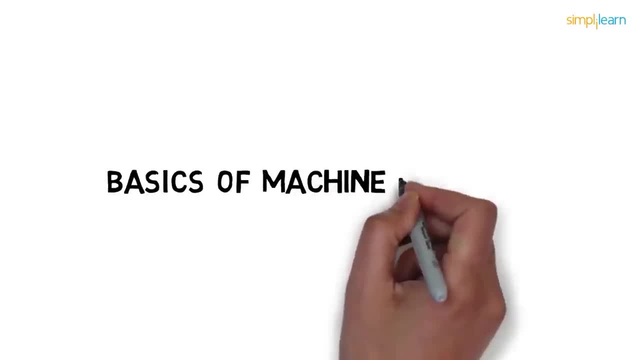 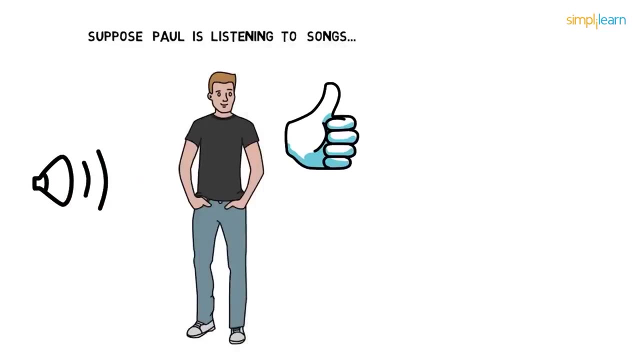 humans can do, and much faster. Well, that's called machine learning. But it's a lot more than just learning. It's also about understanding and reasoning. So today we will learn about the basics of machine learning. So that's Paul. He loves listening to new songs. He either likes them or dislikes them. 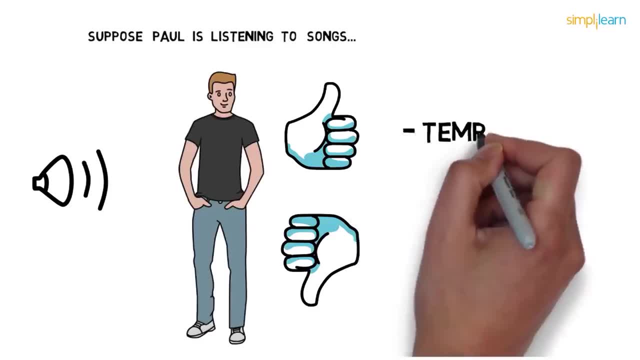 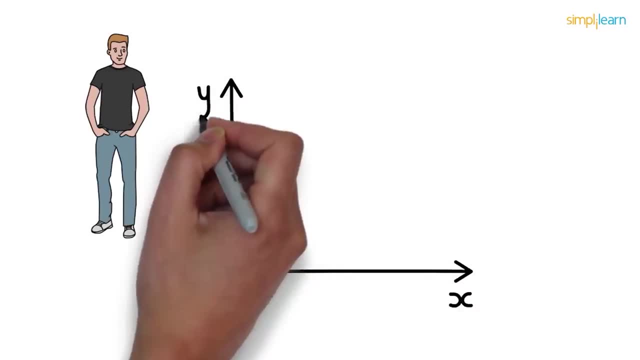 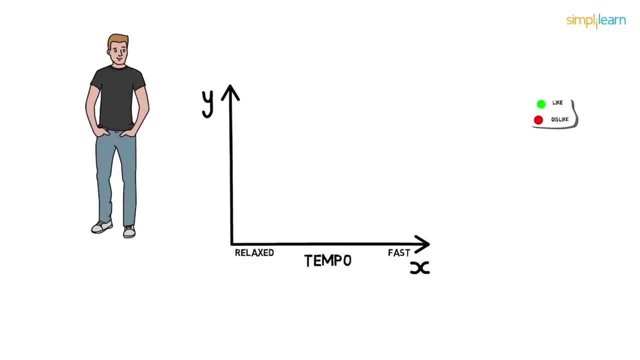 Paul decides this on the basis of the song's tempo, genre, intensity. For simplicity, let's just use tempo and intensity for now. So here, tempo is on the x-axis, ranging from relax to fast, whereas intensity is on the y-axis, ranging from light. 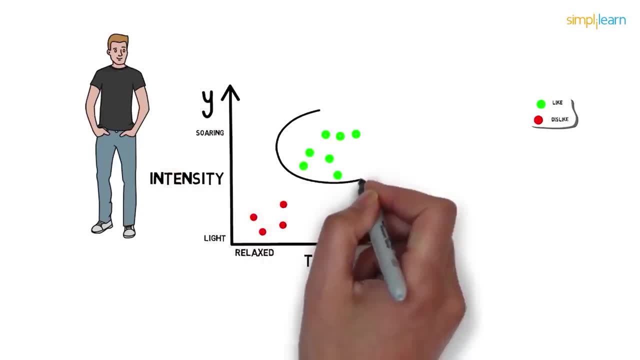 to soaring. We see that Paul likes the song with fast tempo and soaring intensity, while he dislikes the song with relax tempo and light intensity. So now we know Paul's choices. Let's say Paul listens to a new song. Let's name it as song A. Song A has fast tempo and a soaring intensity. 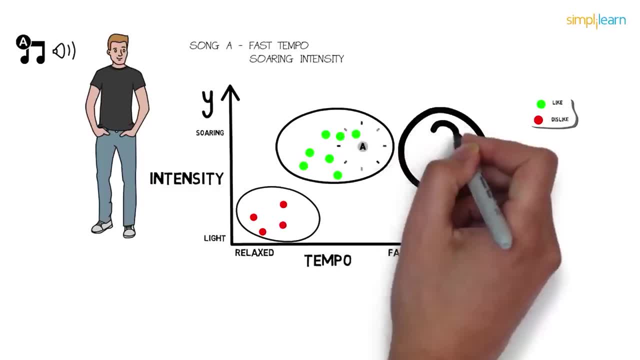 So it lies somewhere here. Looking at the data, can you guess whether Paul will like the song or not? Correct, So Paul likes this song. By looking at Paul's past choices, we were able to classify the unknown song very easily, Right? 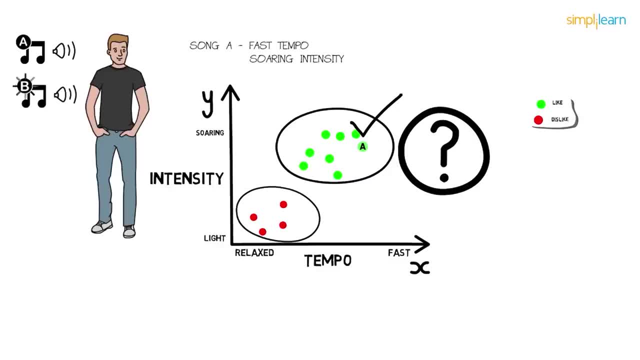 Let's say now Paul listens to a new song, Let's label it as song B. So song B lies somewhere here. Song B has fast tempo and medium intensity, Neither relaxed nor fast, neither light nor soaring. Now can you guess whether Paul likes it or not? Not able to guess whether Paul 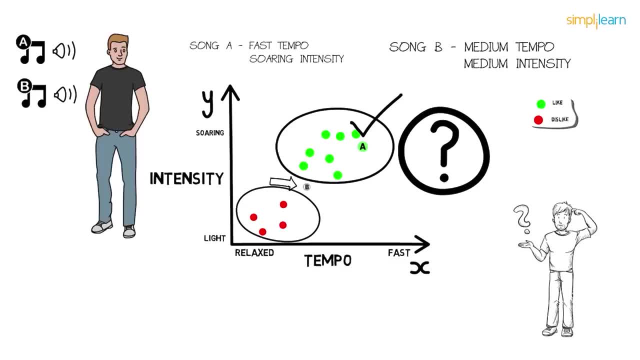 will like it or dislike it. Are the choices unclear? Correct? We could easily classify song A, But when the choice became complicated, as in the case of song B, yes, and that's where machine learning comes in. Let's see how. 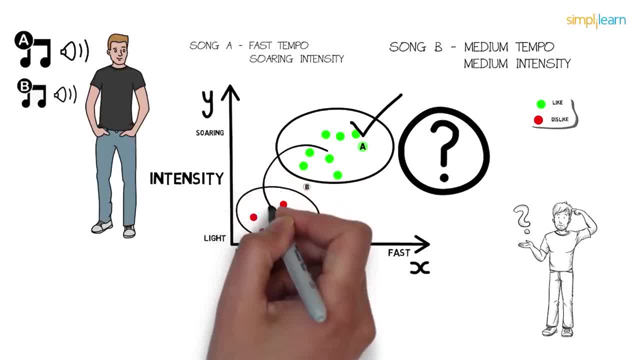 In the same example for song B. if we draw a circle around song B, we see that there are four words for learning- Like, Whereas one word for dislike. If we go for the majority words, we can say that Paul will definitely like the song. That's all. This was a basic machine learning. 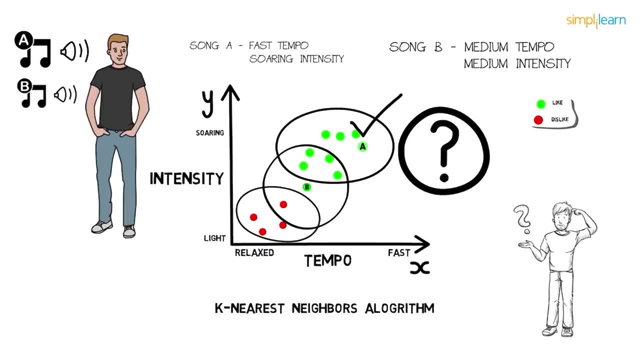 algorithm. also, It's called k-nearest neighbors. So this is just a small example in one of the many machine learning algorithms. Quite easy, right, Believe me it is. But what happens when the choices become complicated, as in the case of song B? That's when machine 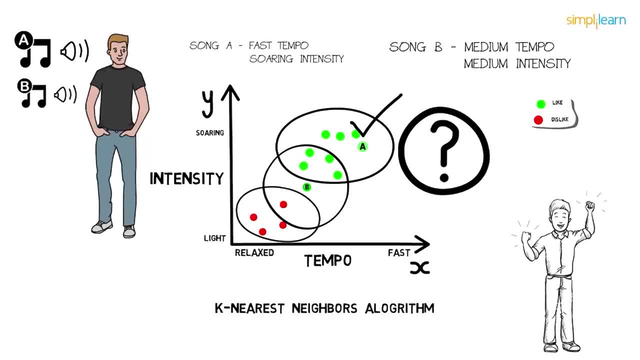 learning comes in. It learns the data, builds the prediction model and when the new data, new data point comes in, it can easily predict for it. More the data, better the model, higher will be the accuracy. There are many ways in which the machine learns. It could be either: 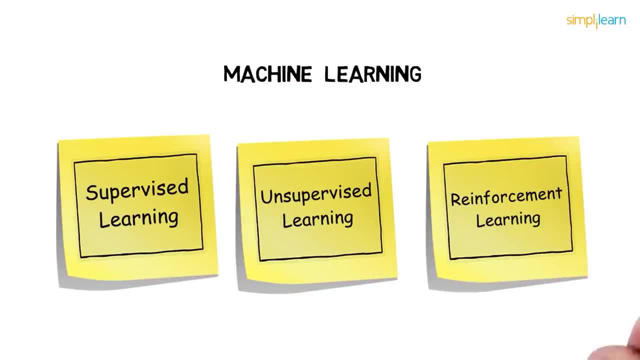 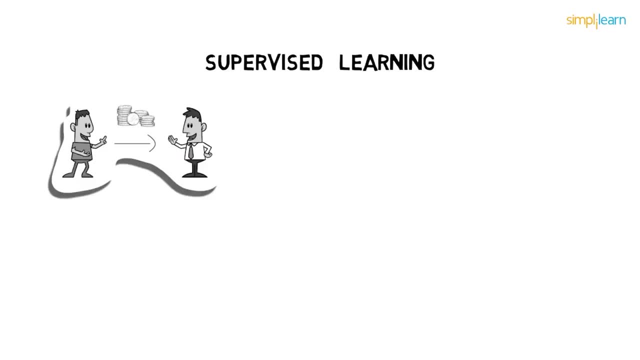 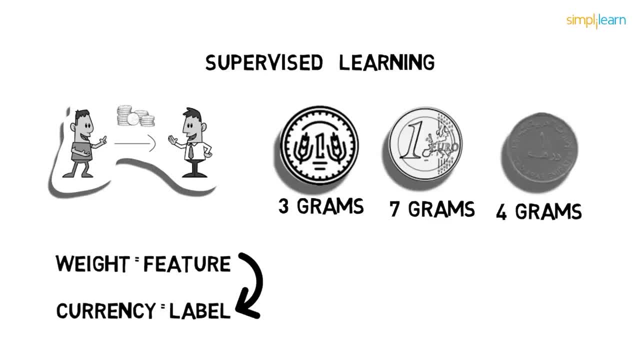 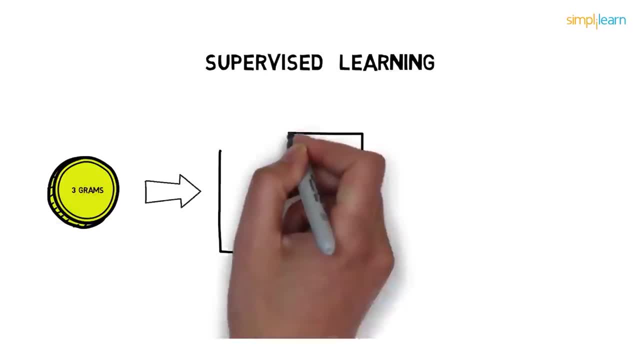 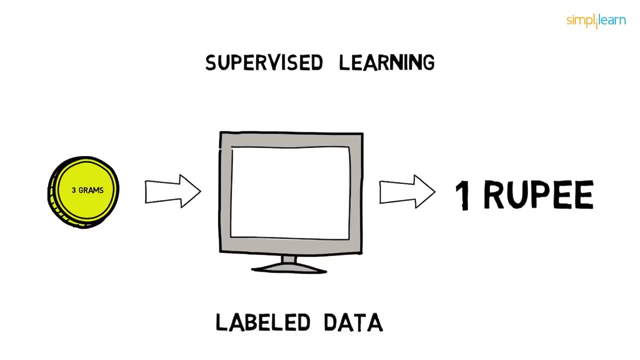 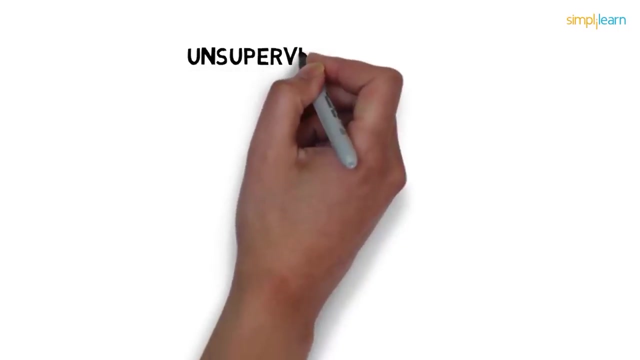 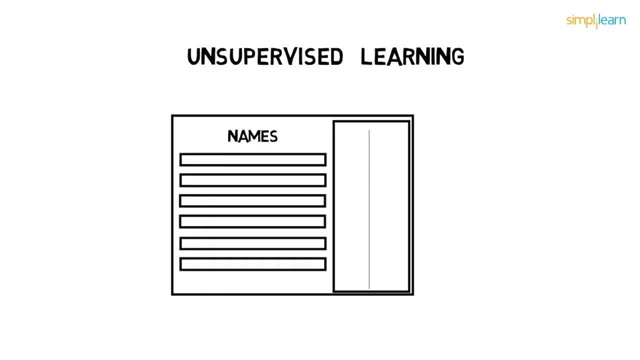 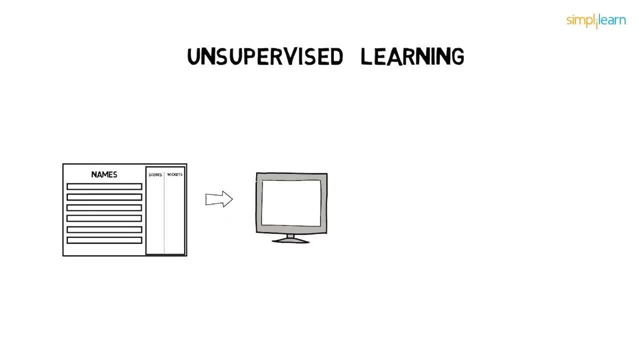 On this note, let's move to unsupervised learning and see the difference. Suppose you have a cricket data set of various players with their respective scores and the wickets taken. When we feed this data set to the machine, the machine identifies the pattern of player performance, So it plots these data on the 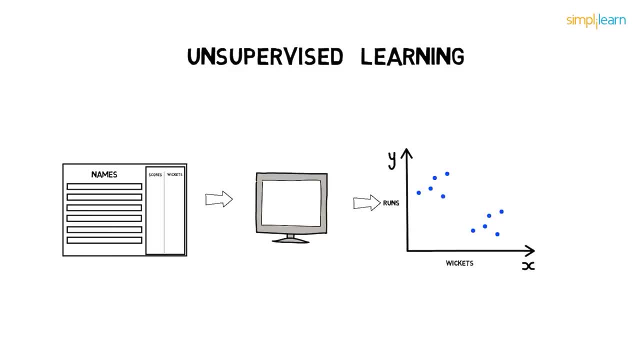 other half while runs on the y axis. While looking at the data, you can clearly see that there are two clusters. The one cluster are the players who scored high runs and took less wickets, while the other cluster is of the players who scored less runs but took many wickets. so here we interpret these two. 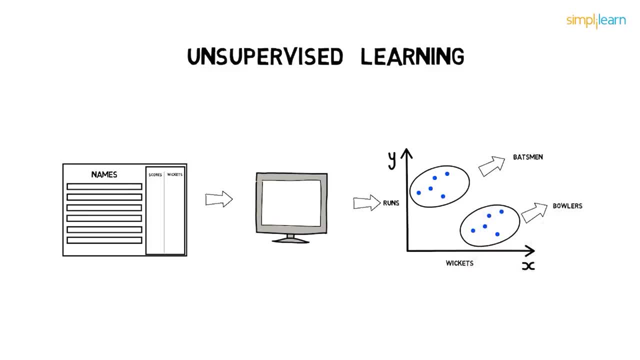 clusters as batsmen and bowlers. the important point to note here is that there were no labels of batsmen and bowlers, hence the learning with unlabeled data is unsupervised learning. so we saw supervised learning where the data was labeled and the unsupervised learning where the data was. 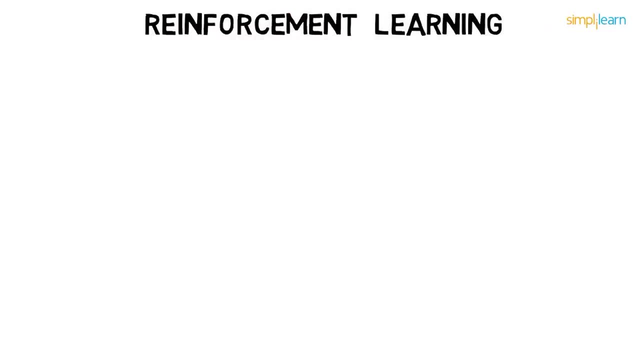 unlabeled. and then there is reinforcement learning, which is reward-based learning, or we can say that it works on the principle of feedback here. let's say you provide the system with an image of a dog and ask it to identify it. the system identifies it as a cat, so you give a negative feedback to. 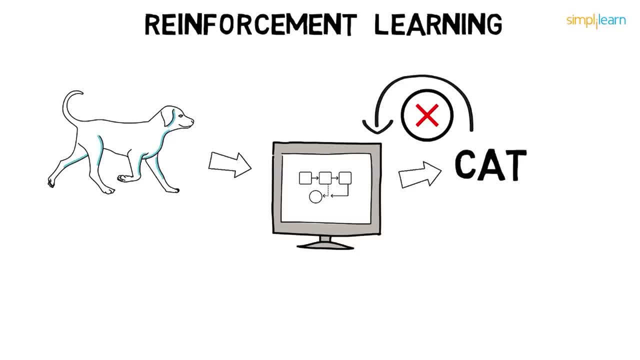 the machine saying that it's a dog's image. the machine will learn from the feedback and, finally, if it comes across any other image of a dog, it will be able to classify it correctly. that is reinforcement learning. to generalize machine learning model. let's see a flow chart. input is: 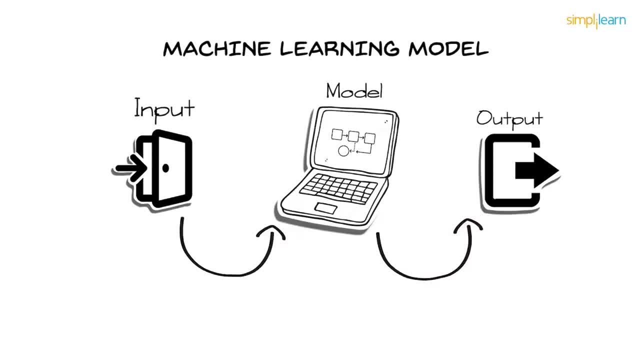 given to a machine learning model, which then gives the output according to the algorithm applied. you can see that the input is given to a machine learning model, which then gives the output according. if it's right, we take the output as a final result. else we provide feedback to the training model. 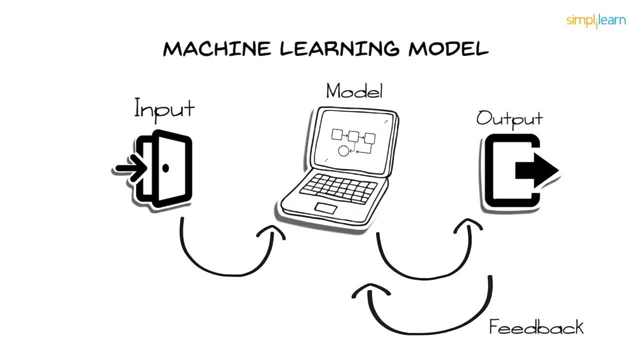 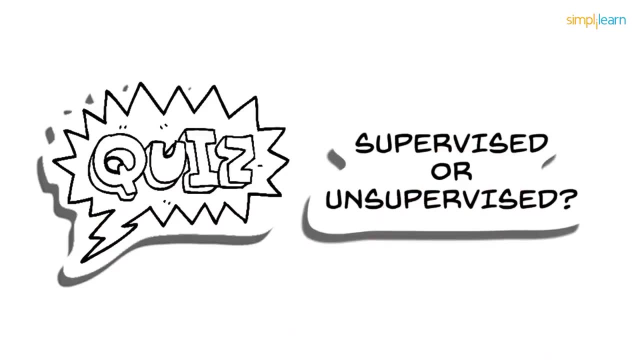 and ask it to predict until it learns. i hope you've understood supervised and unsupervised learning, so let's have a quick quiz. you have to determine whether the given scenarios uses supervised or unsupervised learning. simple, right. scenario one: facebook recognizes your friend in a 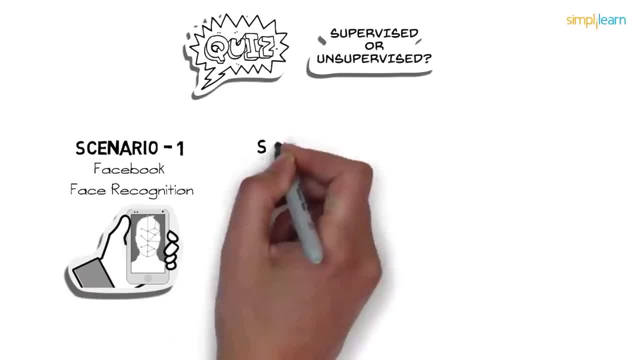 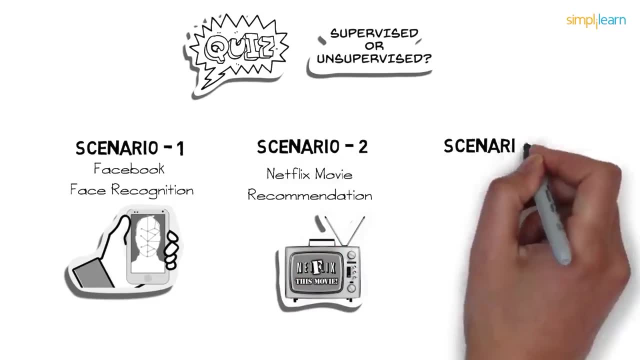 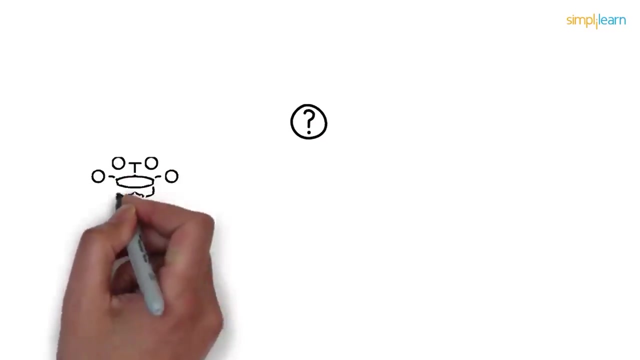 picture from an album of tagged photographs. scenario 2: netflix recommends new movies based on someone's past movie choices. scenario 3: analyzing bank data for suspicious transactions and flagging the fraud transactions. think wisely and comment below your answers. moving on, don't you sometimes wonder how is machine learning possible in today's era? well, that's because. 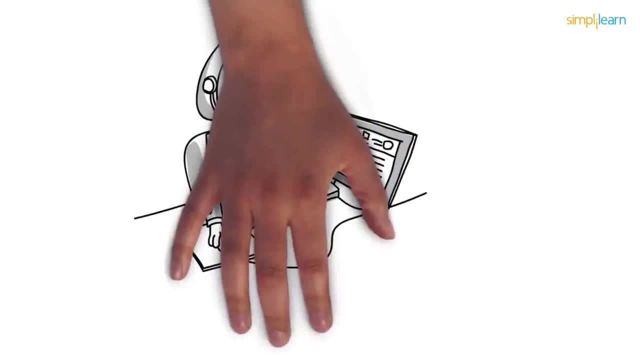 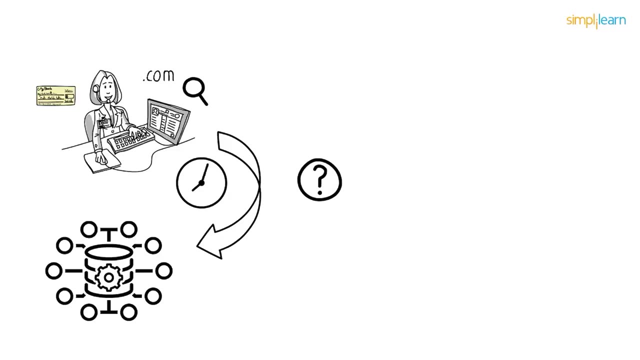 today we have humongous data available. everybody's online, either making a transaction or just surfing the internet, and that's generating a huge amount of data every minute. and that data, my friend, is the key to victory analysis. also, the memory handling capabilities of computers have largely increased, which helps them. 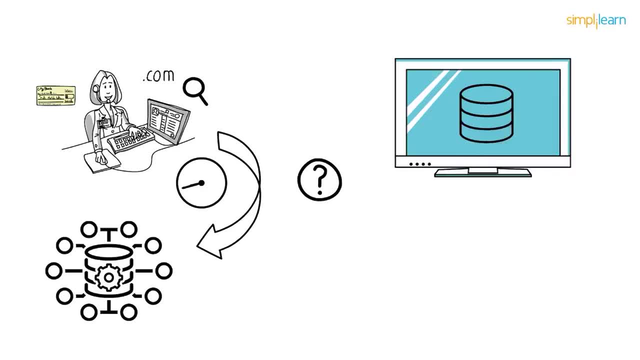 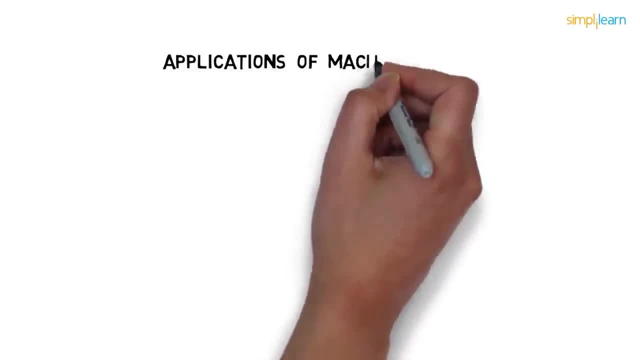 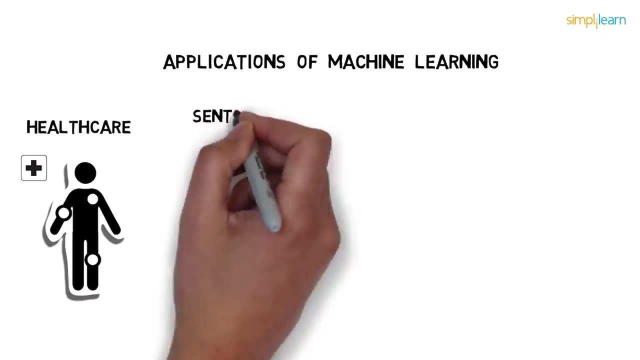 to process such a huge amount of data at hand without any delay. and, yes, computers now have great computational powers, so there are a lot of applications of machine learning out there. to name a few, machine learning is used in healthcare, where diagnostics are predicted for doctor's review. the sentiment analysis that the tech giants are doing on social media: 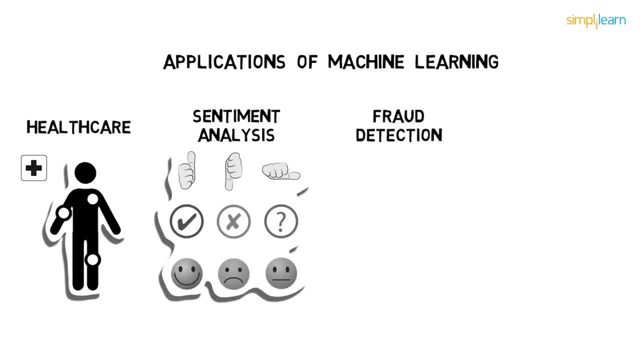 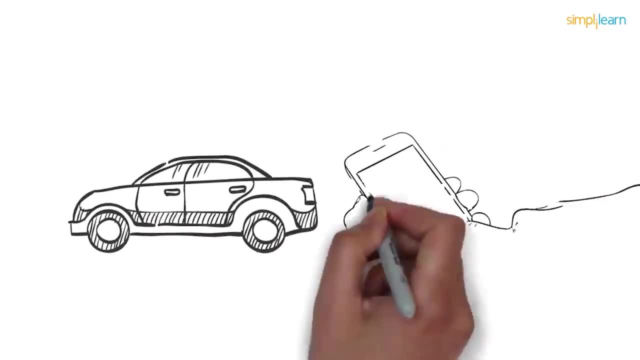 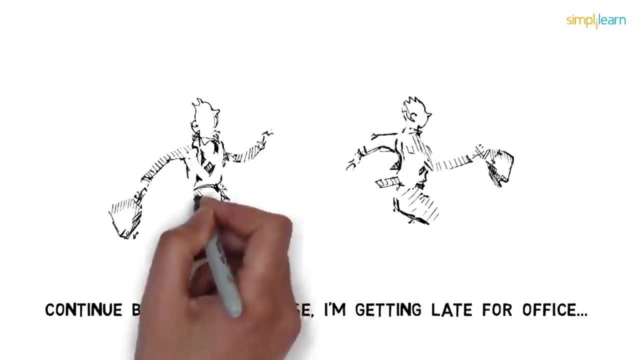 is another interesting application of machine learning: fraud detection in the finance sector and also to predict customer churn in the e-commerce sector. while booking a gap, you must have encountered surge pricing, often where it says the fare of your trip has been updated. continue booking. yes, please, i'm getting laid for office. 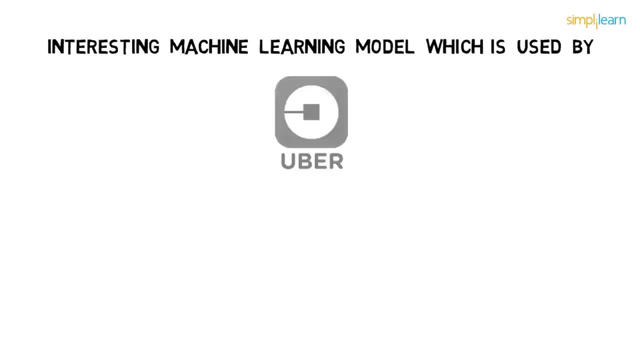 well, that's an interesting machine learning model which is used by global taxi giant, uber and others, where they have differential pricing in real time based on demand, the number of cars available, bad weather, rush hour, etc. so they use the surge pricing model model to ensure that those who need a cab can get one. also, it uses predictive. 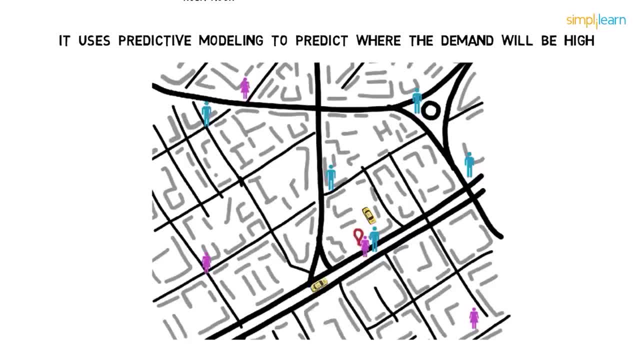 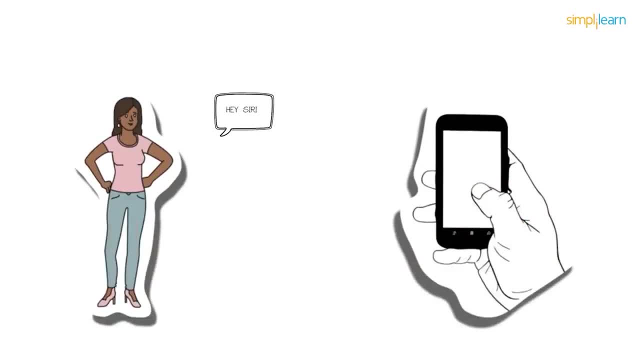 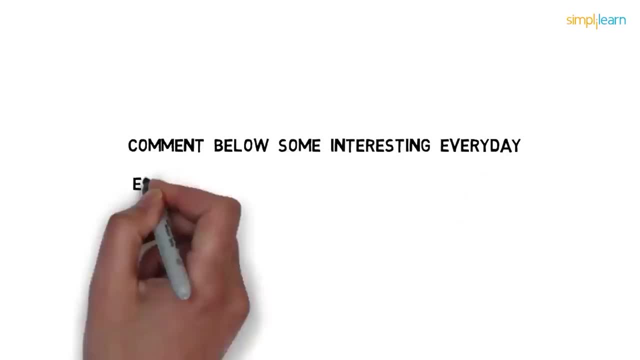 modeling to predict where the demand will be high, with a goal that drivers can take care of the demand and search pricing can be minimized. great, hey, Siri, can you remind me to book a cab at 6 pm today? okay, I'll remind you. thanks, no problem. comment below some interesting everyday examples around you. 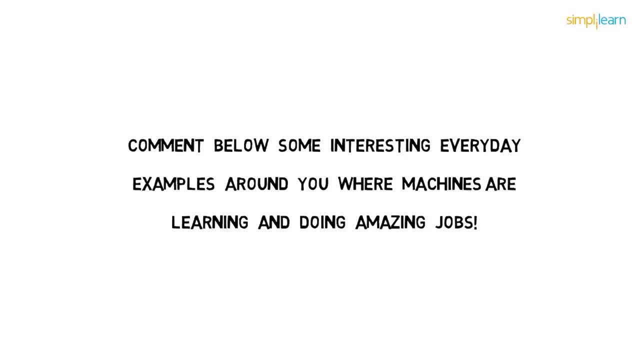 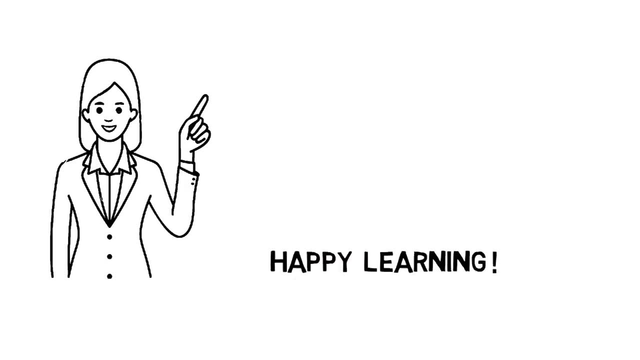 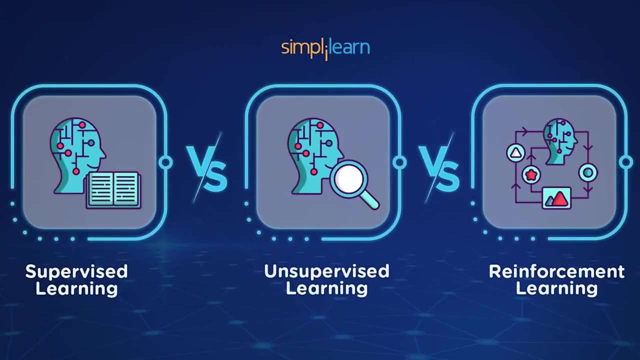 where machines are learning and doing amazing jobs. so that's all for machine learning basics today from my site. keep watching the space for more interesting videos. until then, happy learning. hello everyone, welcome to this tutorial. by simply learn in this video, you will learn about an interesting machine. 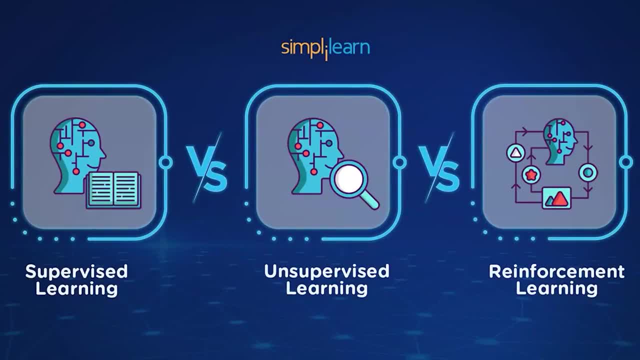 learning topic, that is, supervised versus unsupervised, versus reinforcement learning. let's discuss each of them in detail and understand when to use these algorithms, along with their applications. now, there are a number of algorithms used in the field of machine learning to solve complex problems. each of these algorithms is used to solve complex problems, such as: 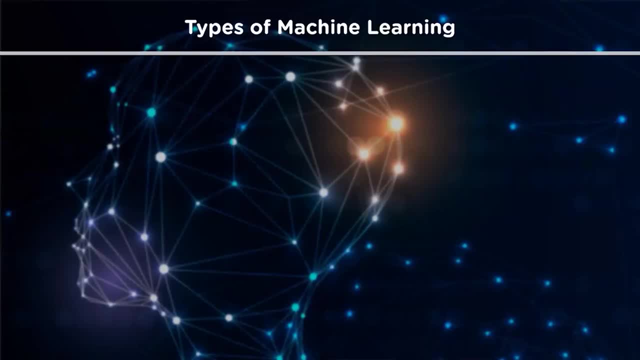 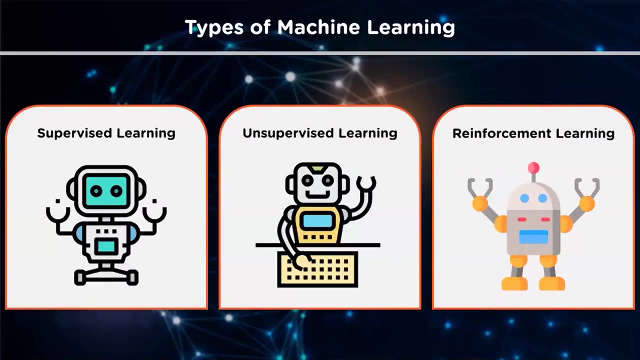 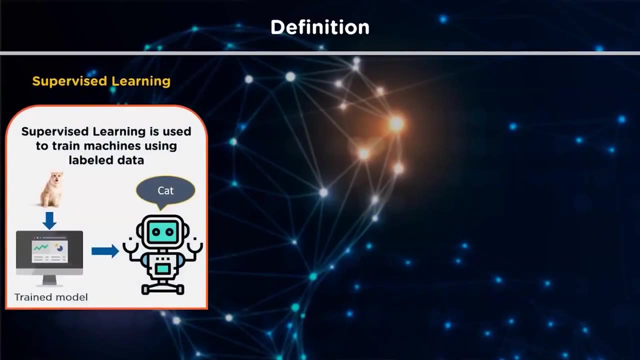 each of these algorithms can be classified into a certain category, so the different types of machine learning algorithms are supervised learning, unsupervised learning and reinforcement learning. now let's look at the definition of each of these learning techniques. supervised learning uses labeled data to train machine learning models. labeled data means that the 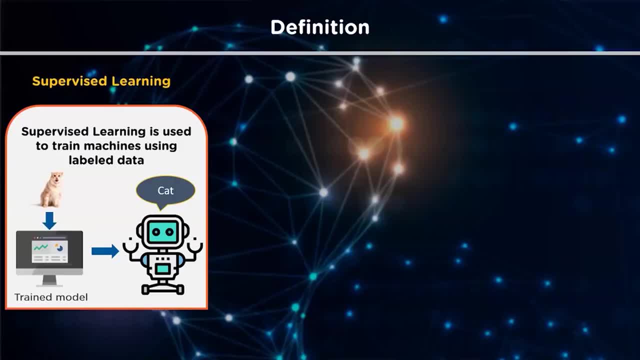 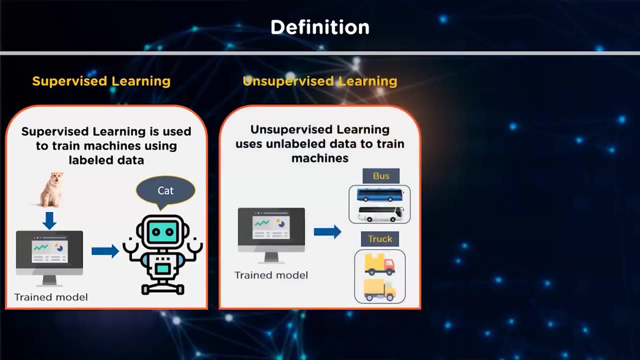 output is already known to you. the model just needs to map the inputs to the outputs. an example of supervised learning can be to train a machine- cheese interfer milestone machine- that identifies the image of an animal. below you can see, we have our trained model that identifies the picture of a cat- unsupervised learning. 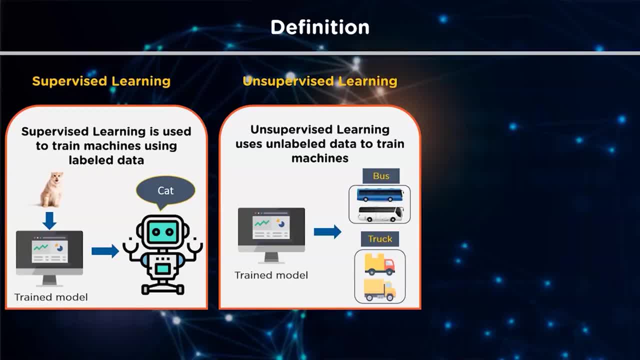 uses unlabeled data to train machines. unlabeled data means there is no fixed output variable. the model learns from the data, discovers patterns and features in the data and returns the output. here is an example of an unsupervised learning technique that uses the images of vehicles to classify if it's a bus or 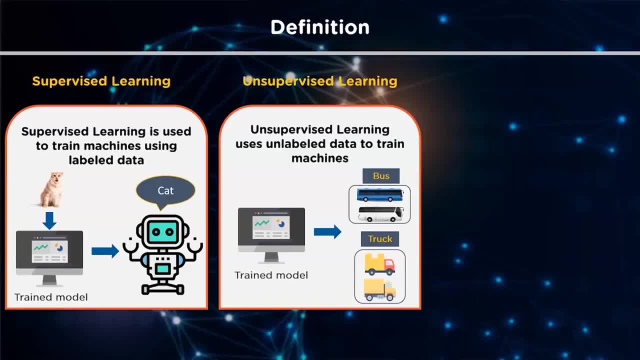 a truck. so the model learns by identifying the parts of a vehicle in the of a vehicle, such as the length and width of the vehicle, the front and rear end covers, roof hoods, the types of wheels used, etc. Based on these features, the model classifies. 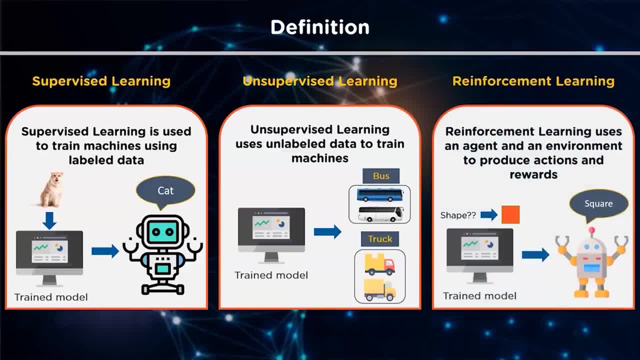 if the vehicle is a bus or a truck. Reinforcement learning trains a machine to take suitable actions and maximize reward in a particular situation. It uses an agent and an environment to produce actions and rewards. The agent has a start and an end state, but there might be different paths. 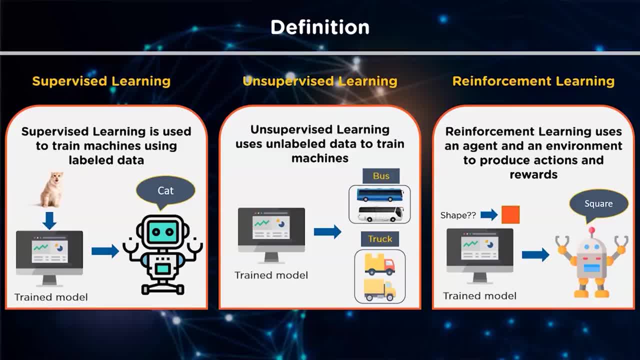 for reaching the end state like a maze. In this learning technique there is no predefined target variable. An example of reinforcement learning is to train a machine that can identify the shape of an object, given a list of different objects, such as square, triangle, rectangle. 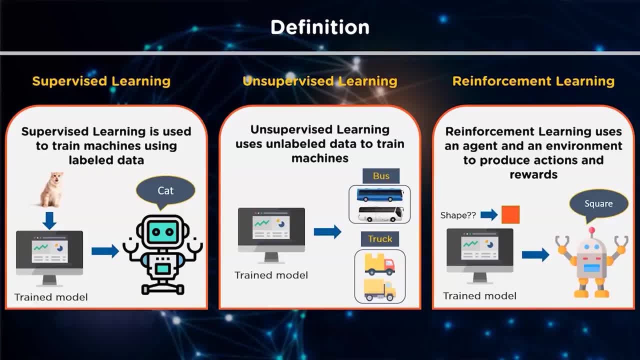 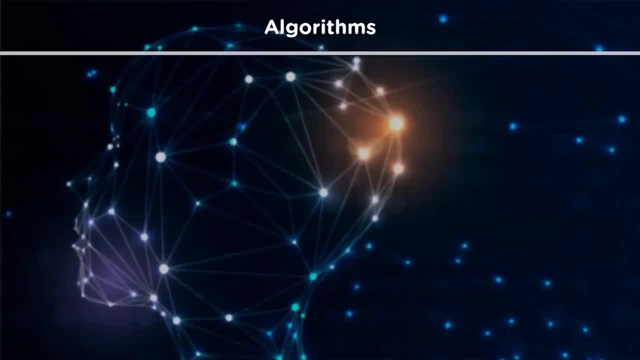 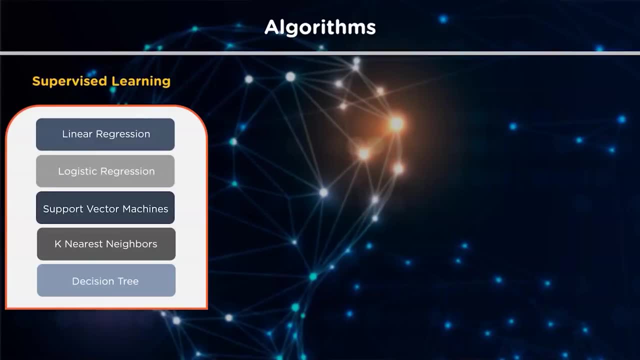 or a circle. In the example shown, the model tries to predict the shape of the object, which is a square here. Now let's look at the different machine learning algorithms that come under these learning techniques. Some of the commonly used supervised learning algorithms are: Linear regression, logistic. 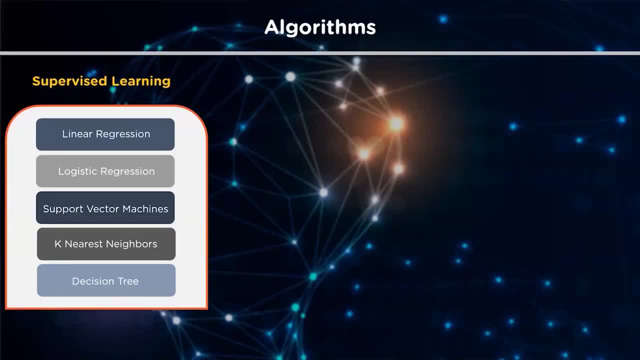 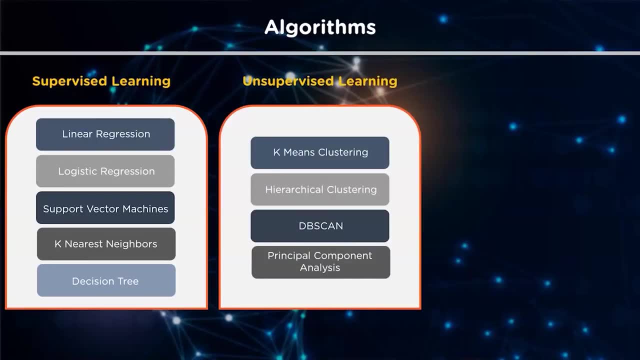 regression, support, vector machines, k-nearest neighbours, decision tree, random forest and naive Bayes. Examples of unsupervised learning algorithms are k-means clustering, hierarchical clustering, db-scan, principal component analysis and others. Choosing the right algorithm depends. 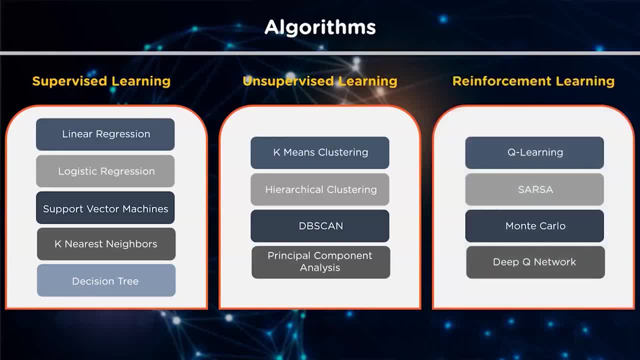 on the type of problem you are trying to solve. For example, you could choose the type of trying to solve. Some of the important reinforcement learning algorithms are Q-learning, Monte Carlo, SARSA and Deep Q-network. Now let's look at the approach in which these machine learning techniques work. 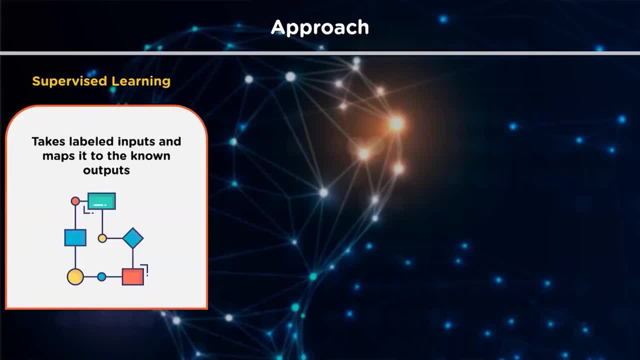 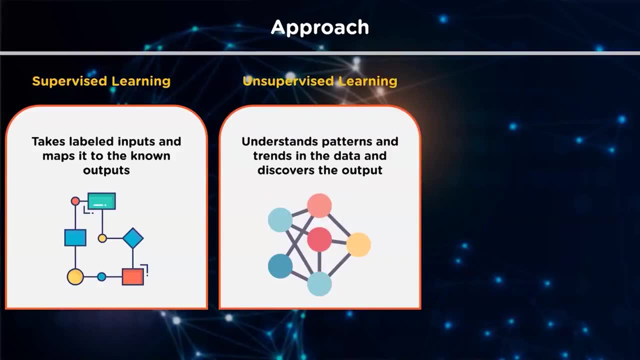 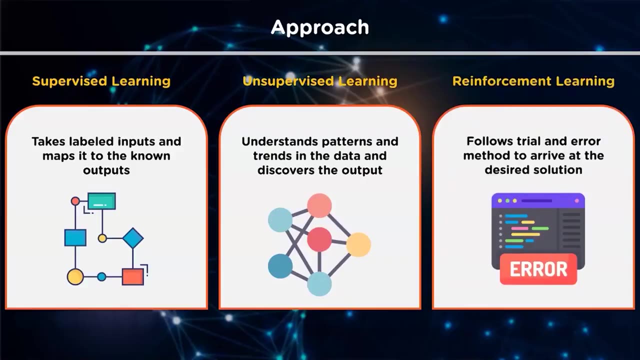 So supervised learning takes labeled inputs and maps it to known outputs, which means you already know the target variable. Unsupervised learning finds patterns and understands the trends in the data to discover the output. So the model tries to label the data based on the features of the input data, while reinforcement 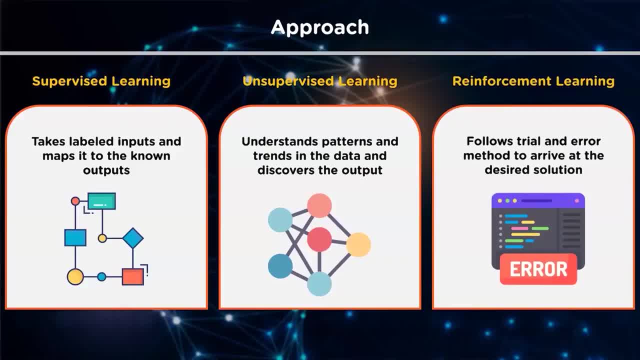 learning follows trial and error method to get the desired solution. After accomplishing a task, the agent receives an award. An example could be to train a dog to catch the ball. If the dog learns to catch a ball, you give it a reward such as a biscuit. 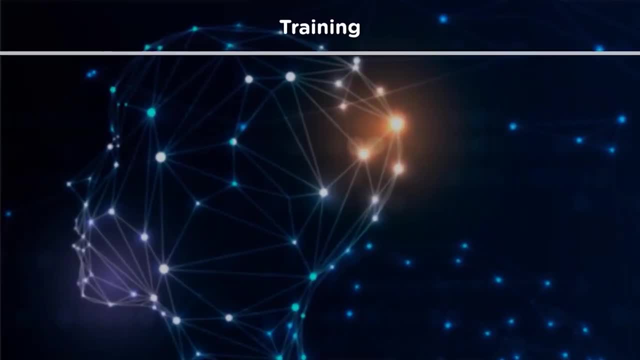 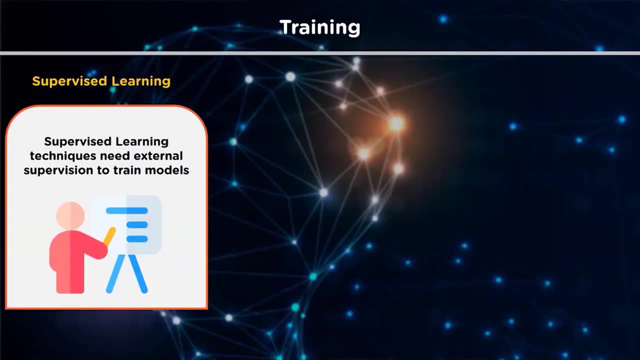 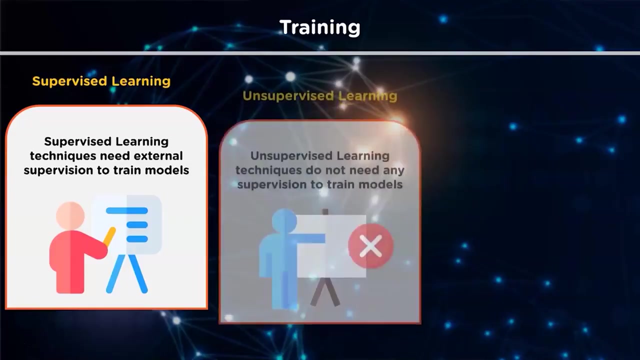 Now let's discuss the training process for each of these learning methods. So supervised learning methods need to be trained. They need external supervision to train machine learning models, and hence the name supervised. They need guidance and additional information to return the result. Unsupervised learning techniques do not need any supervision to train models. 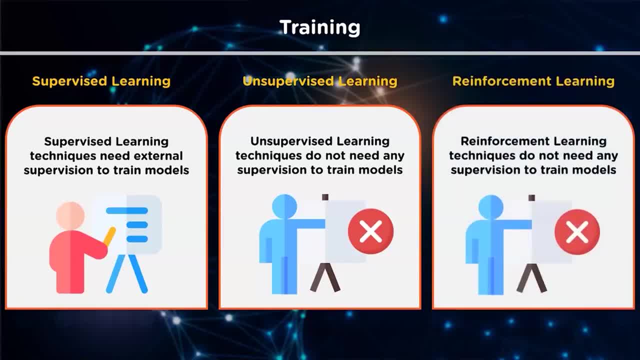 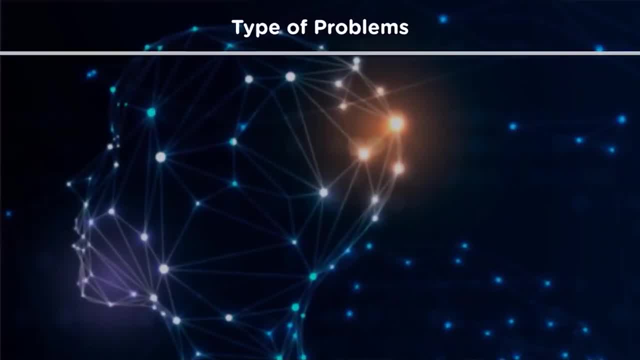 They learn on their own and predict the output. Similarly, reinforcement learning methods do not need any supervision to train machine learning models. And with that let's focus on the types of problems that can be solved using these three types of machine learning methods. 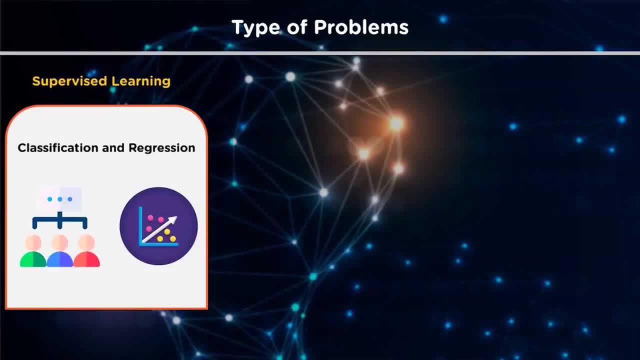 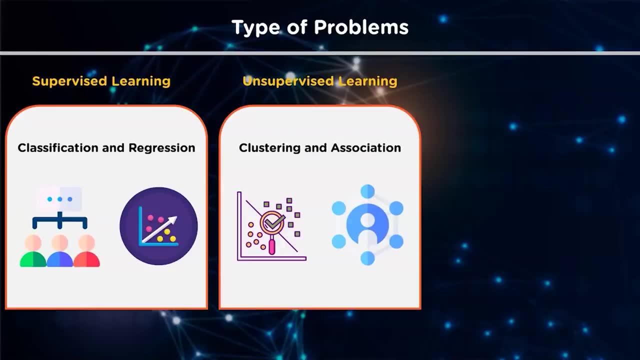 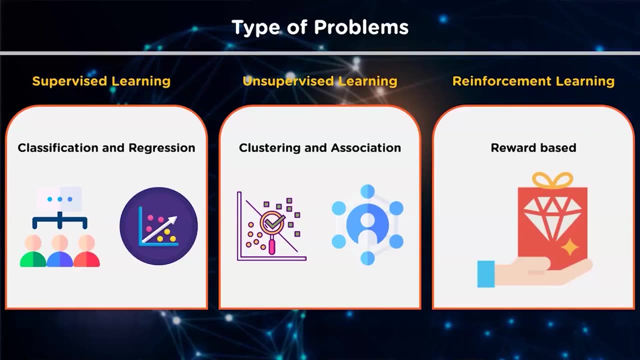 So supervised learning is generally used for classification and regression problems- We'll see the examples in the next slide- And unsupervised learning is used for clustering and association problems, While reinforcement learning is reward based. So for every task or for every step completed, there will be a reward received by the agent. 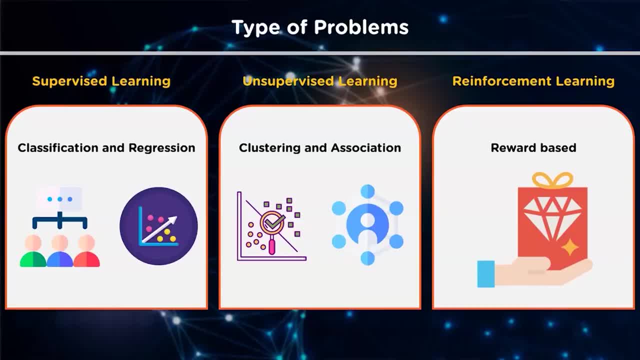 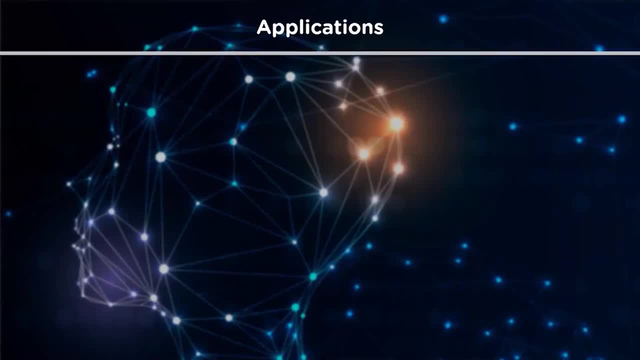 And if the task is not achieved correctly, there will be some penalty used. Now let's look at a few examples: Applications of supervised, unsupervised and reinforcement learning. As we saw earlier, supervised learning are used to solve classification and regression. 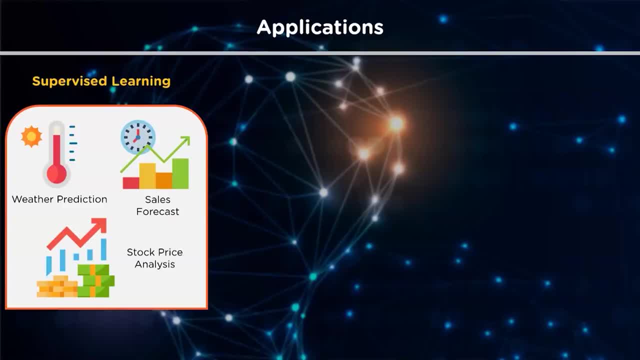 problems. For example, you can predict the weather for a particular day based on humidity, precipitation, wind speed and pressure values. You can use supervised learning algorithms to forecast sales for the next month or the next quarter for different products. Similarly, you can use it for stock price analysis or identifying if a cancer cell is. 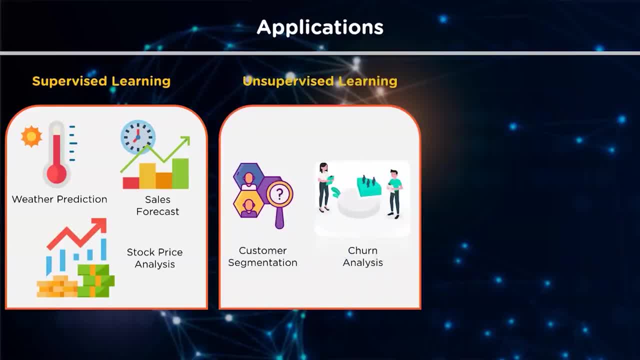 malignant or benign. Now talking about the applications of unsupervised learning, we have customer segmentation, So based on customer behavior, likes, dislikes and interests, you can segment and cluster similar customers into a group. Another example where unsupervised learning algorithms are used is customer churn analysis. 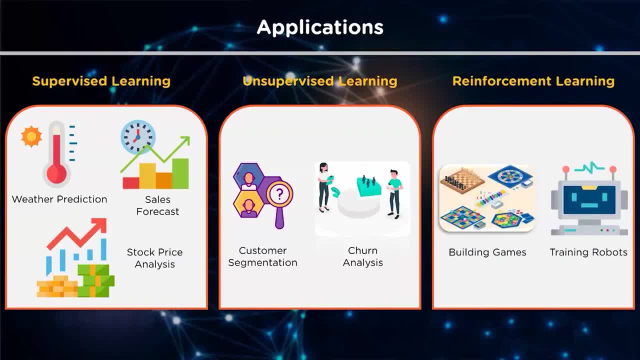 Now let's see what applications we have in reinforcement learning. So reinforcement learning algorithms are widely used in the gaming industries to build games. It is also used to train robots. It is also used to train robots. It is also used to train robots to perform human tasks. 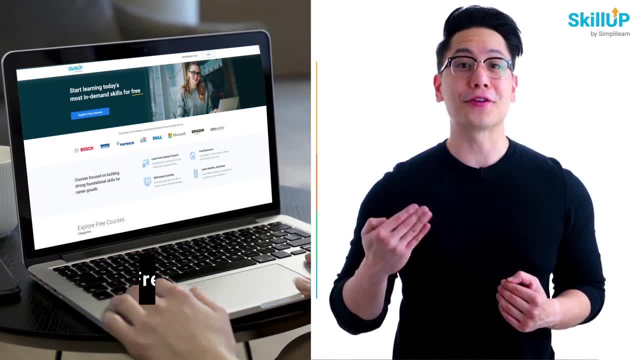 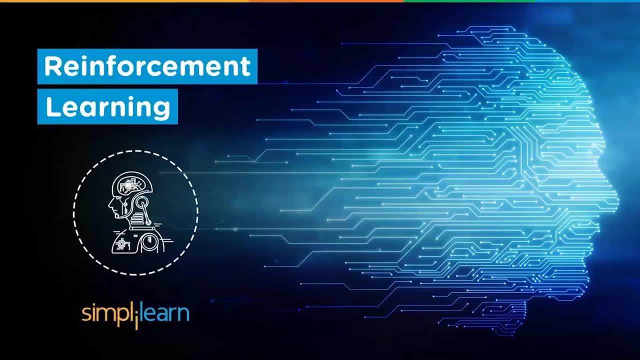 If getting your learning started is half the battle, what if you could do that for free? Visit SkillUp by SimplyLearn. Click on the link in the description to know more Reinforcement learning by SimplyLearn. My name is Richard Kirshner with the SimplyLearn team. 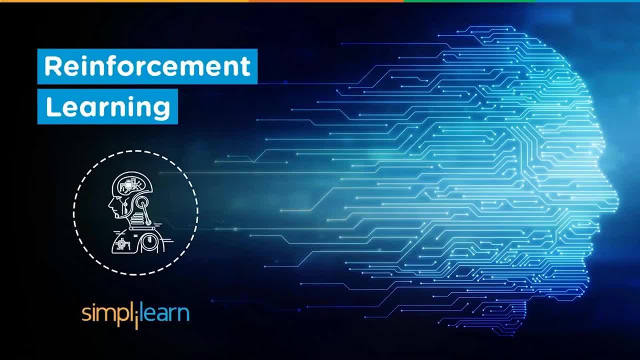 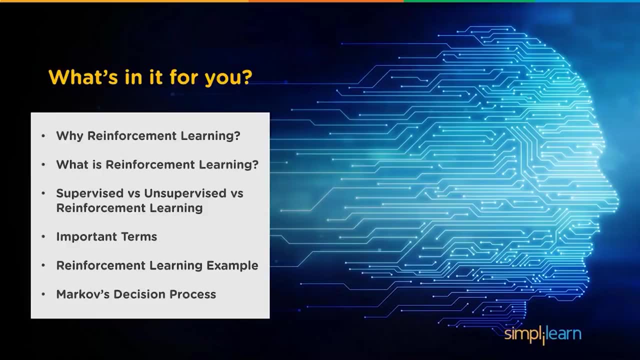 That's wwwsimplylearncom. Get certified, Get ahead. We're going to cover reinforcement learning today And what's in it for you. We'll start with why reinforcement learning. We'll look at what is reinforcement learning. We'll see what the different kinds of learning strategies are that are being used today in 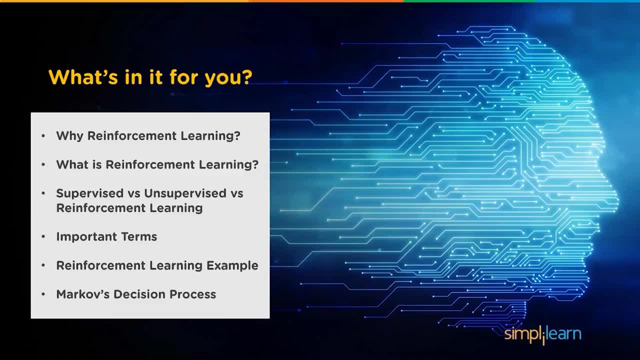 computer models under supervised versus unsupervised, versus reinforcement. We'll cover important terms specific to reinforcement learning. We'll talk about Markov's decision process And we'll take a look at a reinforcement learning example where we'll teach a tic-tac-toe how 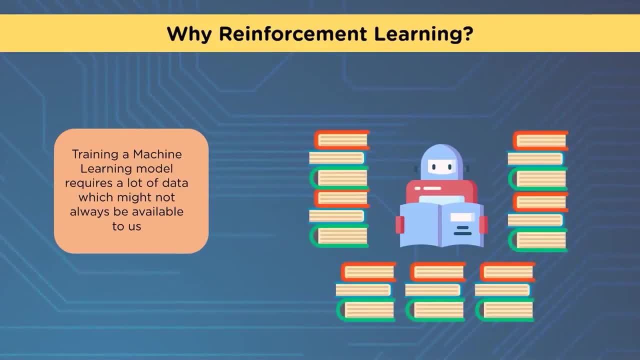 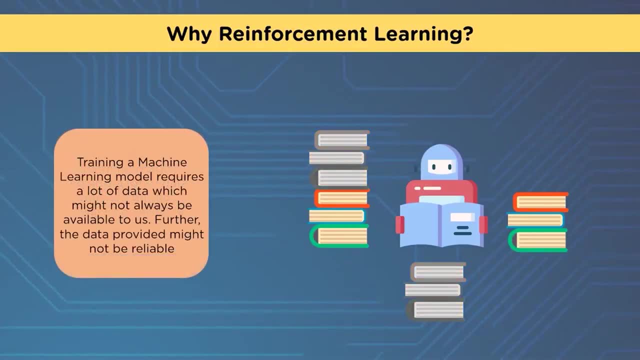 to play. Why reinforcement learning Training a machine learning model requires training. Why reinforcement learning Training a machine learning model requires a lot of data, which might not always be available to us. Why reinforcement learning? It requires a lot of data which might not always be available to us. 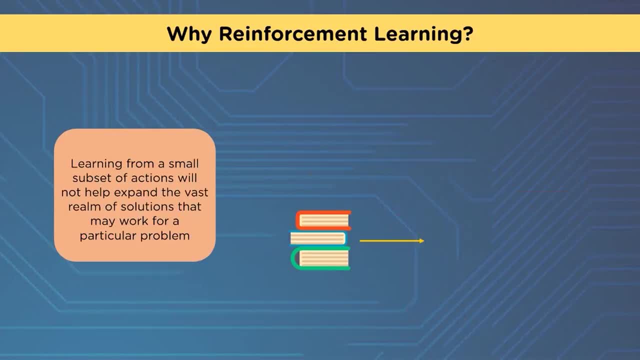 Further, the data provided might not be reliable. Learning from a small subset of actions will not help expand the vast realm of solutions that may work for a particular problem. You can see here we have the robot learning to walk, Very complicated set up when you're learning how to walk and you'll start asking questions. 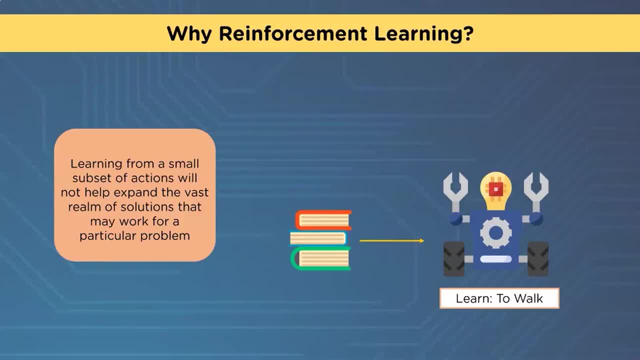 like if I'm taking one step forward and left. what happens if I pick up a 50 pound object? How does that change how a robot would walk? These things are very difficult to program because there's no actual information on it until it's actually tried out. 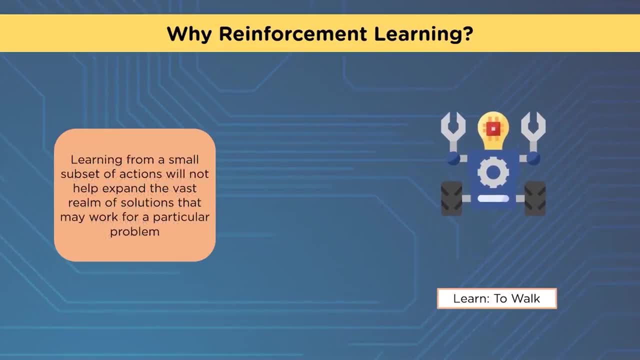 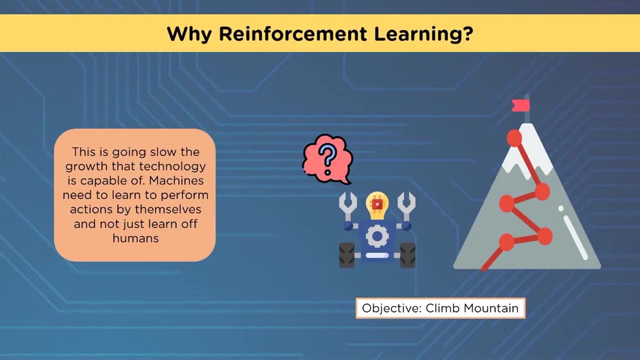 Learning from a small subset of actions will not help expand the vast realm of solutions that may work for a particular problem, And we'll see here. it learned how to walk. This is going to slow the growth that technology is capable of. Machines need to learn to perform actions by themselves and not just learn. 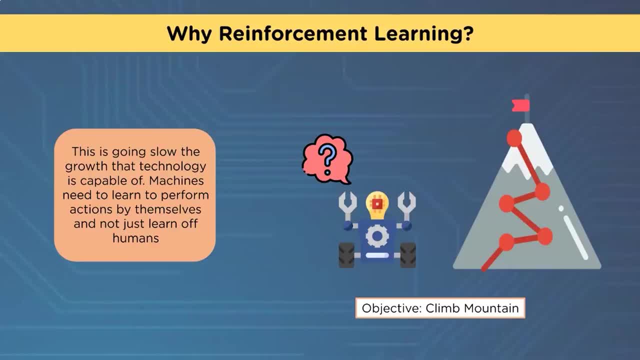 off humans And you see the objective: climb a mountain. A real interesting point here is that as human beings we can go into a very unknown environment and we can adjust for it and kind of explore and play with it. Most of the models, the 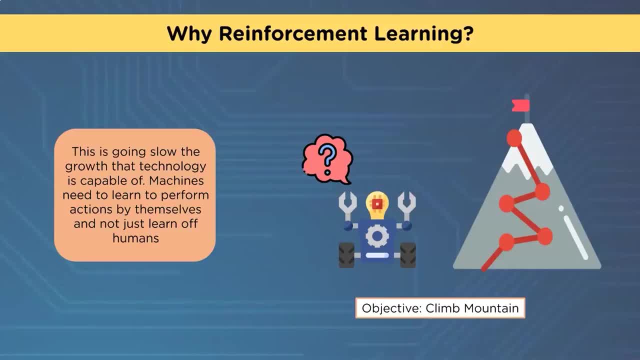 non-reinforcement models in computer machine learning aren't able to do that very well. There's a couple of them that can be used or integrated to see how it goes. This is what we're talking about with reinforcement learning. So what is? 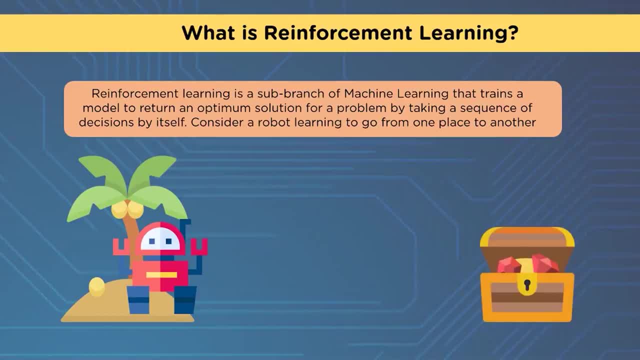 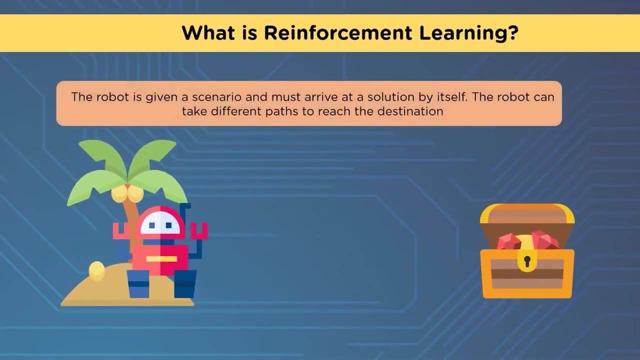 reinforcement learning. Reinforcement learning is a sub-branch of machine learning that trains the model to return an optimum solution for a problem by taking a sequence of decisions by itself. Consider a robot learning to go from one place to another. The robot is given a scenario and must arrive at a solution by 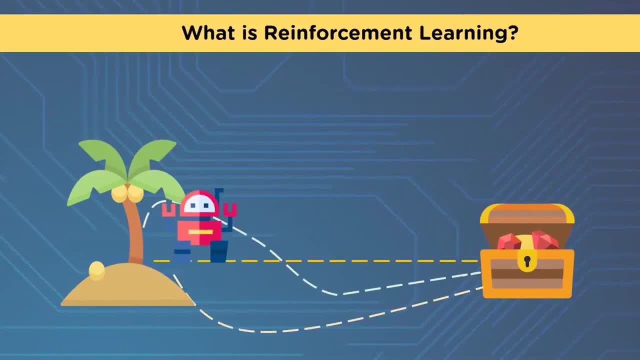 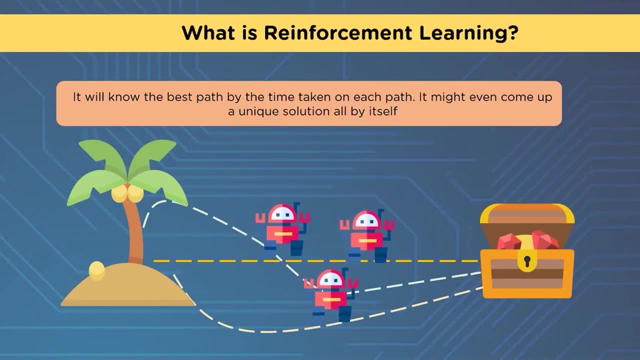 itself. The robot can take different paths to reach the destination. It will know the best path by the time it reaches the destination. It might even come up with a unique solution all by itself, And that's really important, as we're looking for unique solutions. We want the best solution, but you can't find. 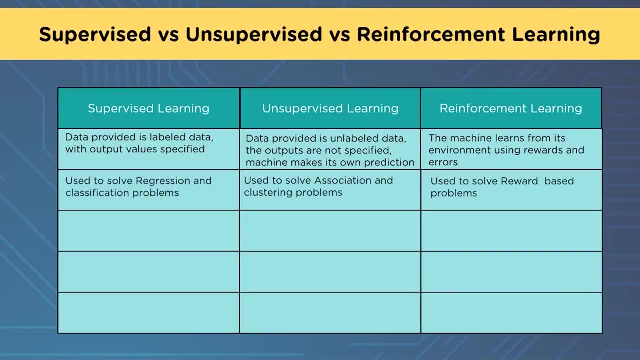 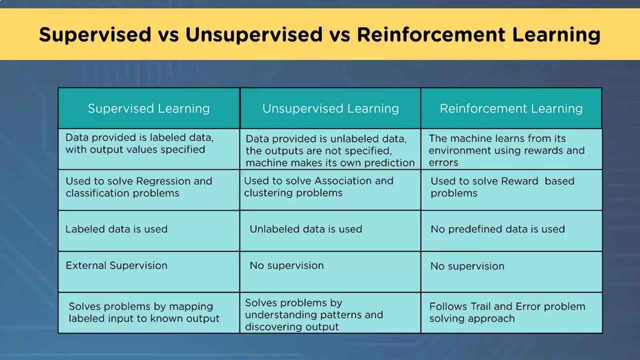 it unless you try it. So we're looking at our different systems, Our different model. We have supervised versus unsupervised versus reinforcement learning And with the supervised learning that is probably the most controlled environment. We have a lot of different supervised learning models where there's linear learning, linear 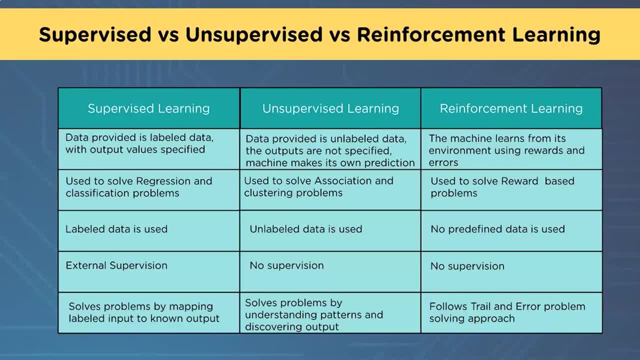 regression, neural networks- there's all kinds of things in between decision trees. the data provided is labeled data with output values specified, and this is important because we talk about supervised learning. you already know the answer for all this information. you already know the picture has a motorcycle in it, so you're supervised learning. you already know that the 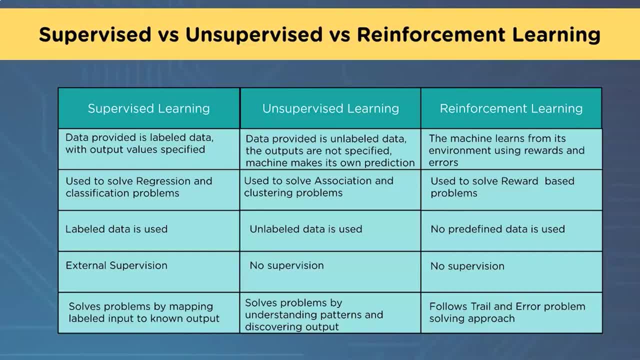 outcome for tomorrow. for you know, going back a week, you're looking at stock. you can already have like the graph of what the next day looks like. so you have an answer for it and you have labeled data which is used. you have an external supervision and solves problems by mapping labeled input to no one output. 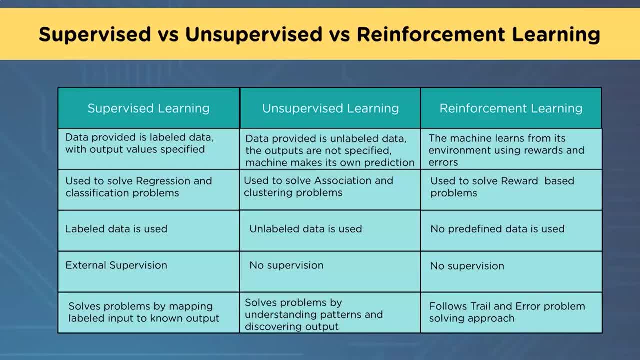 so very controlled unsupervised learning and the end to provide learning is really interesting because it's now taking part in many other models. they start with and you can actually insert an unsupervised learning model in almost either supervised or reinforcement learning as part of the system, which is 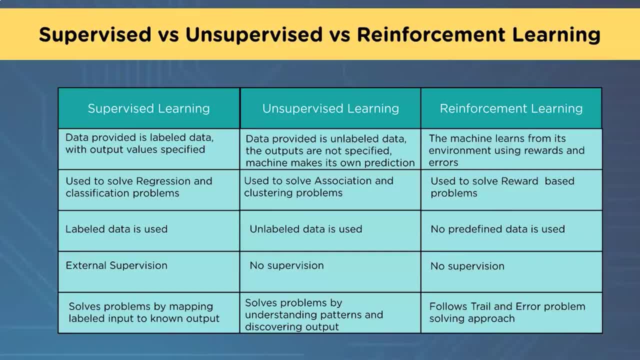 really cool. data provided is unlabeled data. the outputs are not specified. machine makes its own predictions used to solve association with clustering problems. unlabeled data is used. no supervision solves problems by understanding patterns and discovering output. so you can look at this and you can think some. 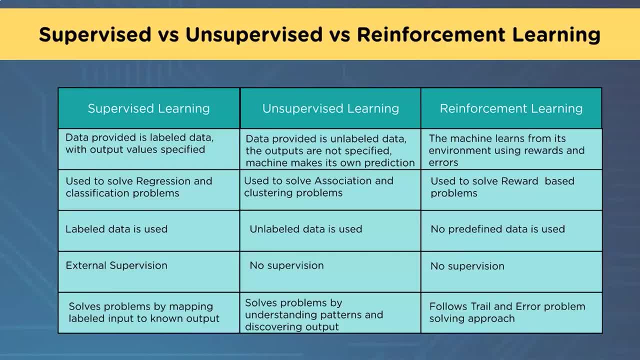 of these things go with each other. they belong together. so it's looking for what connects in different ways and there's a lot of different algorithms that look at this. when you start getting into those are some really cool images that come up of what unsupervised learning is, how it can pick out, say, the area of a donut one. 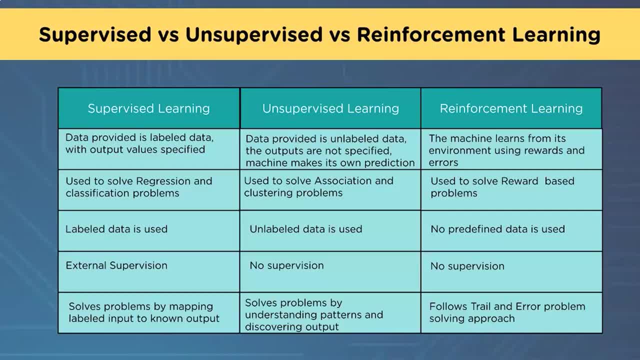 model will see the area of the donut and the other one will divide it into three sections based on this location versus what's next to it. so there's a lot of stuff that goes in with unsupervised learning, and then we're looking at reinforcement learning, probably the biggest industry in today's market in. 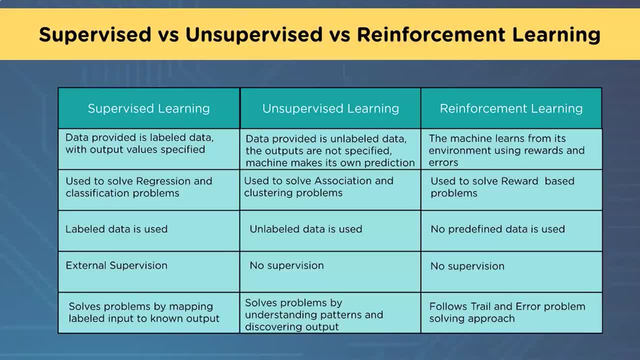 machine learning or growing market. it's very- it's very- infant-staged as far as how it works and what's going to be capable of. the machine learns from its environment using rewards and errors used to solve reward based problems. no predefined data is used, no supervision follows trail and error problem-solving. 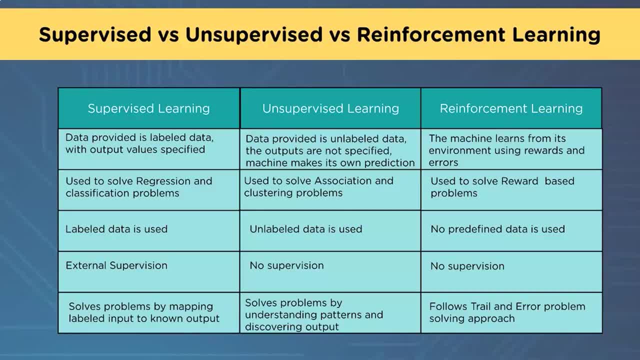 approach. so again we have a random. at first you start with a random, I try this, it works, and this is my reward. doesn't work very well, maybe, or maybe doesn't even get you where you're trying to get it to do, and then you get your reward. 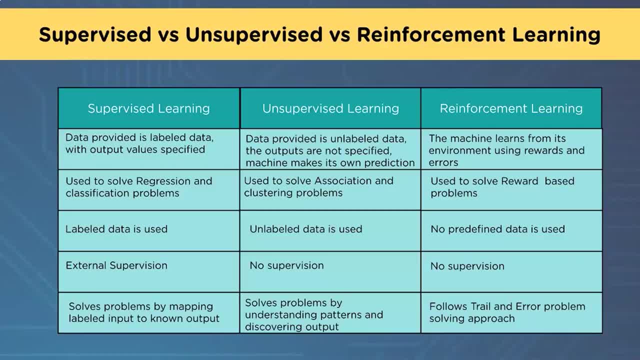 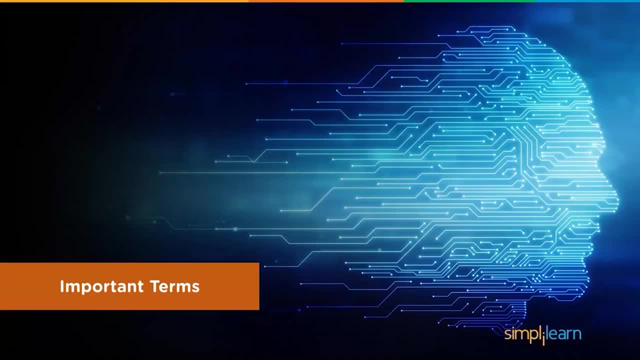 and then it looks at that and says, well, let's try something else. and it starts to play with these different things, finding the best route. so let's take a look at important terms in today's reinforcement model, and this has become pretty standardized over the last few years, so these are really good to know. 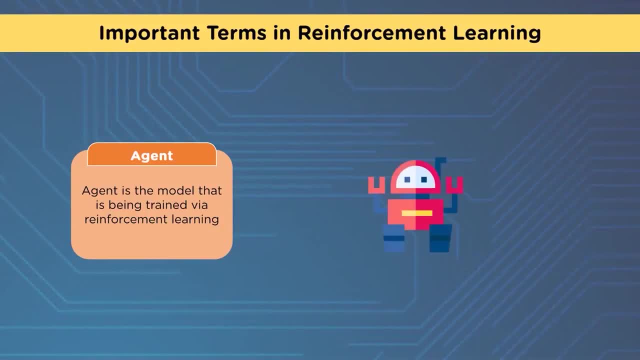 we have the agent. agent is the model that is being trained via reinforcement learning. so this is your actual entity that has, however you're doing it with, using a neural network or cue table or whatever combination thereof, this is the actual agent that you're using. this is the model and you have your environment, the training. 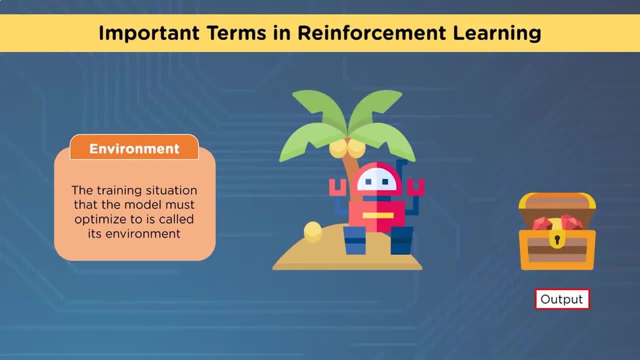 situation that the model must optimize to is called its environment, and you can see here, I guess we have a robot who's trying to get chest full of gyms or whatever, and that's the output, and then you have your action. this is all possible steps that can be taken by the model, and it picks one action and you 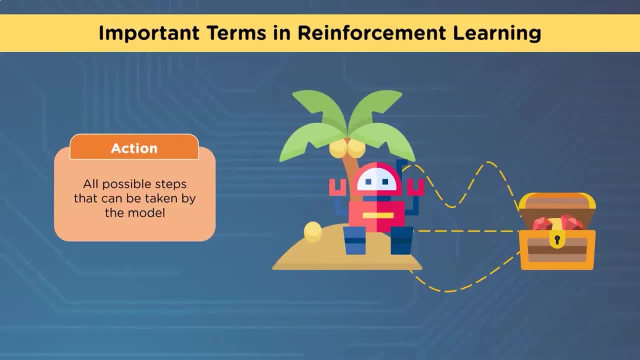 can see here that's picked three different routes to get to the chest of diamonds and gems. we have a state, the current position, condition returned by the model, and you could look at this. if you're playing like a video game, this is the screen you're looking at, so when you go back here, the environment is a whole. 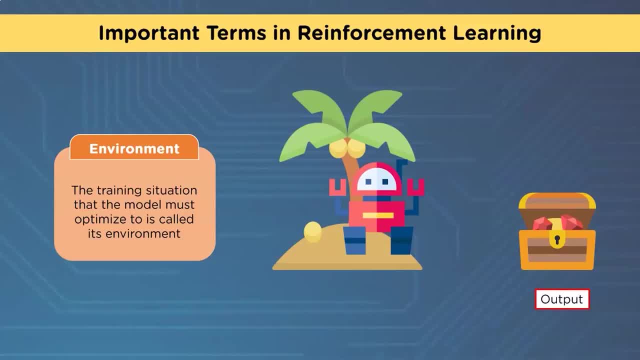 game board. so if you're playing one of those mobius games, you might have the whole game board going on, but then you have your current position. where are you on that game board? what's around that? what's around you? if you were talking about a robot, the environment might be moving around the 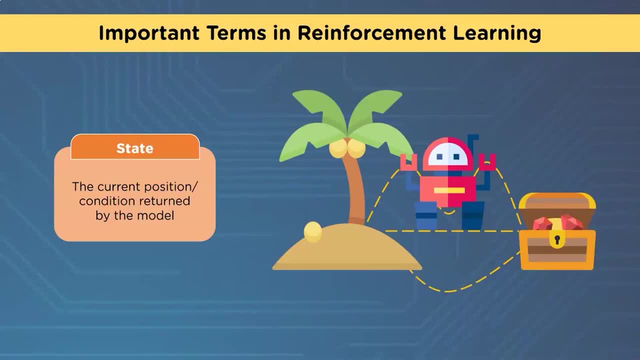 yard, where it is in the yard and what it can see, what input it has in that location. that would be the current position condition returned by the model. and then the reward: to help the model move in the right direction. it is rewarded, points are given to it to appraise some kind of action. so yeah, you. 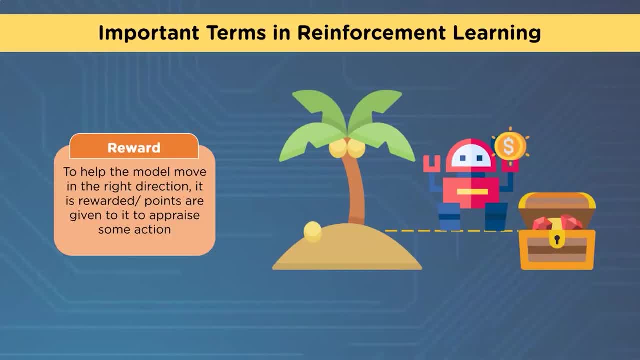 did good or didn't do as good, trying to maximize the reward and have the best reward possible policy. policy determines how an agent will behave at any time. it acts as a mapping between action and present state. this is part of the model, but it would. what is your action? that you're? you're going to take, what's the policy you're? 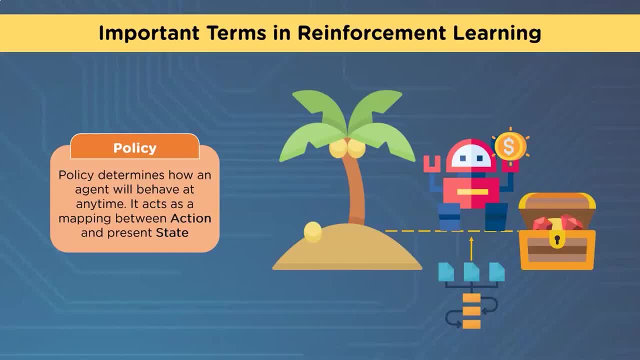 using to have an output from your agent. one of the reasons they separate policy as its own entity is that you usually have a prediction of a different options and then the policy will. how am I going to pick the based on those predictions, I'm going to guess at different options and will. 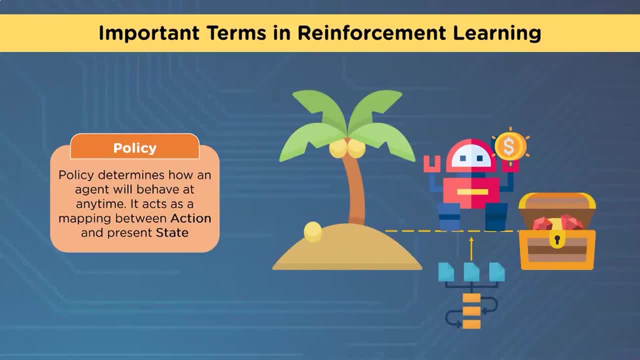 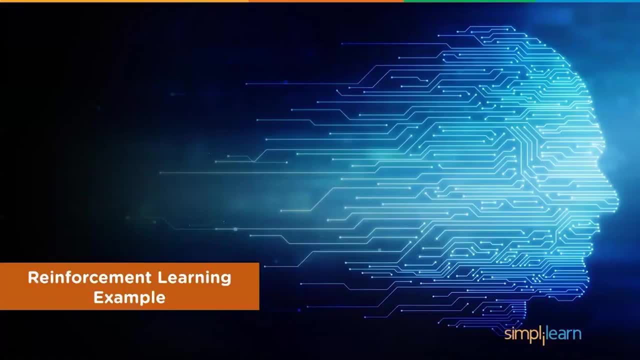 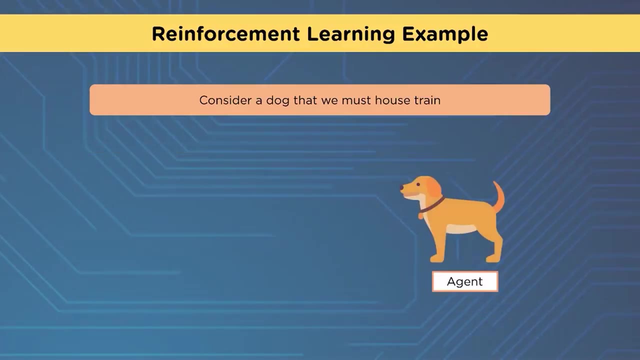 actually weigh those options in and find the best option we think will work. so it's a little tricky, but the policy thing is actually pretty cool how it works. let's go and take a look at a reinforcement learning example and just in looking at this we're going to take a look at consider what a dog that we want. 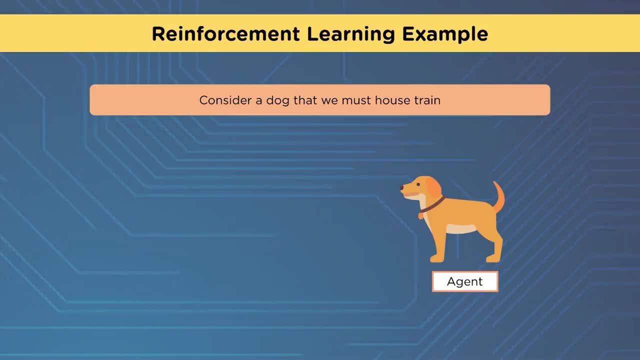 to train. so the dog would be like the agent: you have your, your puppy or whatever, and then your environment is going to be the whole house or whatever it is, or you're training them and then you have an action. we want to teach the dog to fetch. so action equals. 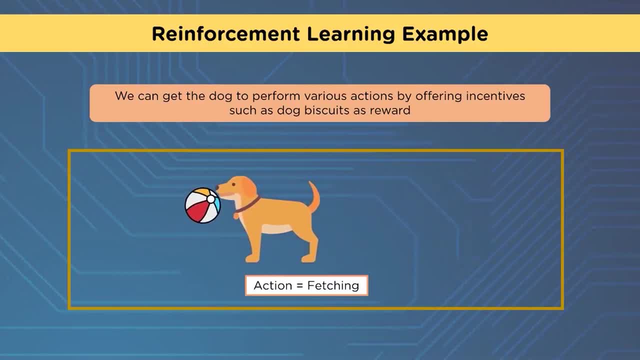 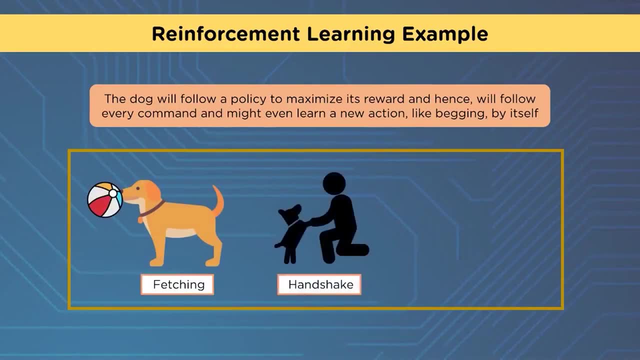 fetching. and then we have a little biscuit. so we can get the dog perform various actions by offering incentives such as a dog biscuit as a reward. the dog will follow a policy to maximize this reward and hence will follow every command and might even learn new actions, like begging, by itself. so we started off. 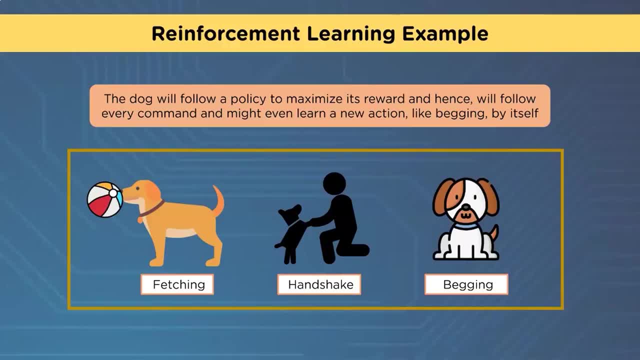 with fetching. it goes: oh, I get a biscuit for that. it tries something else. you get a handshake or begging or something like that and goes: oh, this is also reward based and so kind of explores things to find out what will bring. it is biscuit and it's very. 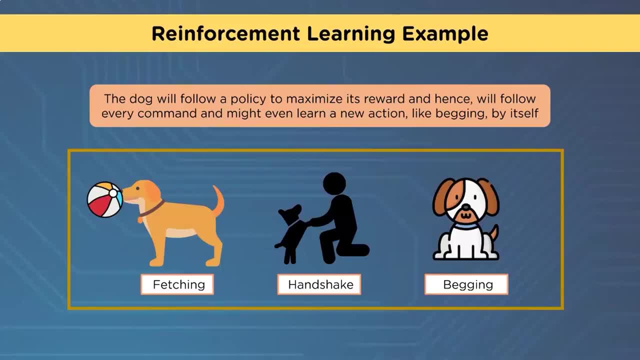 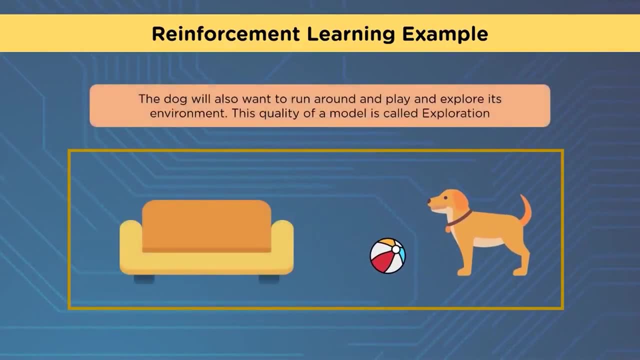 much like a reinforced model goes is it looks for different rewards. how do I find, can I try different things and find a reward that works? the dog also want to run around and play an explorers environment. this quality of model is called exploration, so there's a little randomness going on an exploration and explores new parts of 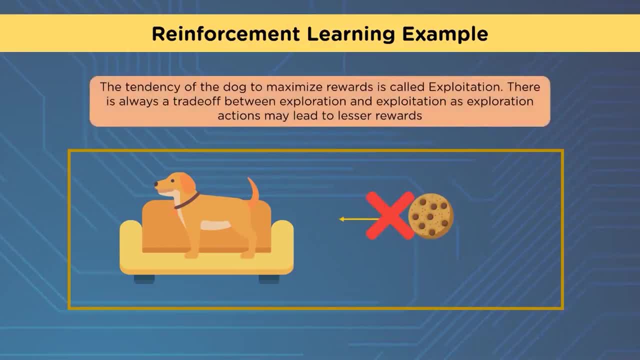 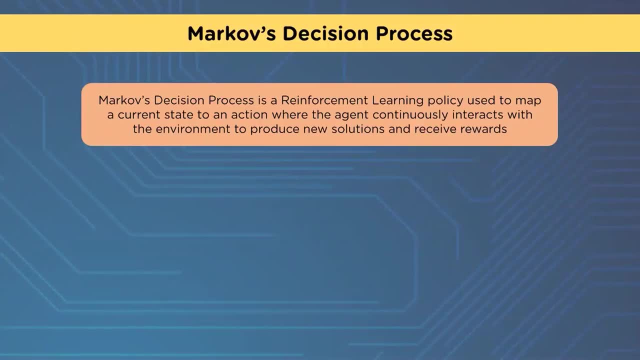 the house. climbing on the sofa doesn't get a reward effect, usually gets kicked off the sofa. so let's talk a little bit about Markov's decision process. Markov's decision process is a reinforcement learning policy used to map a current state to an action where the agent continuously interacts with the 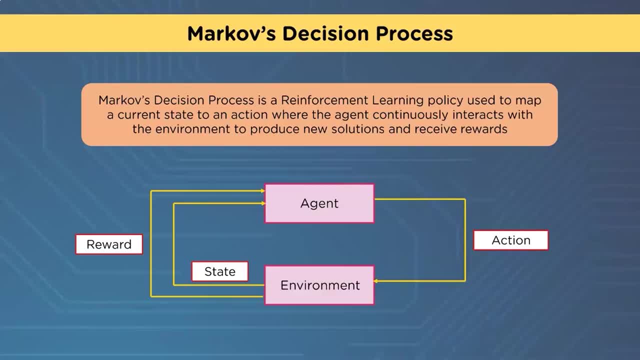 environment to produce new solutions and receive rewards. and you'll see, here's all of our different vocabulary we just went over. we have a reward or state or agent or environment interaction and so, even though the environment kind of contains everything that you really actually writing the program, your environments going to put out a reward in state that 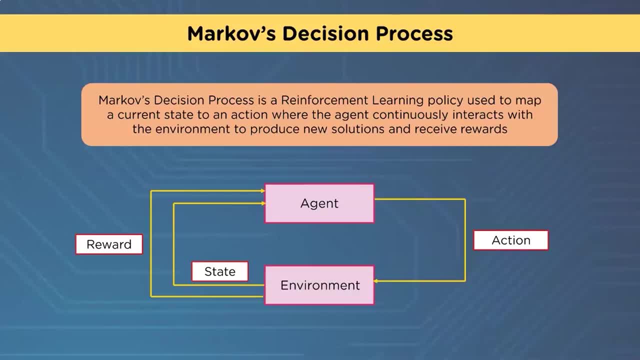 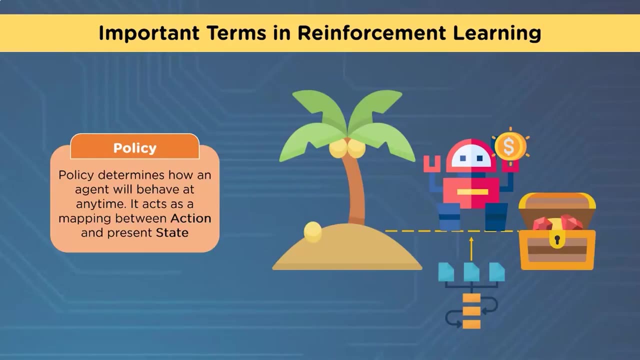 goes into the agent. the agent then looks at this state or looks at the reward, usually first, this is ok, I got rewarded for whatever I just did or didn't get rewarded- and it looks at the state. then it comes back and, if you remember from policy, the policy comes in and then we 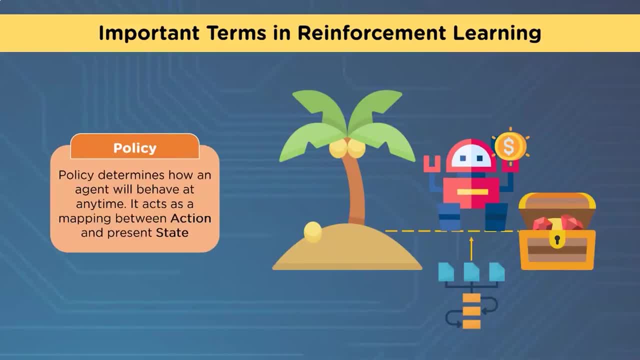 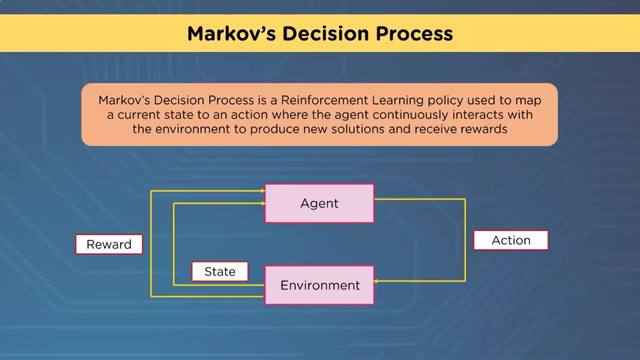 have a reward. the policy is that part that's connected at the bottom, and so it looks at that policy and says, hey, what's a good action? that will probably be similar to what I did or sometimes are completely random, but what's a good action that's going to bring me a different reward. 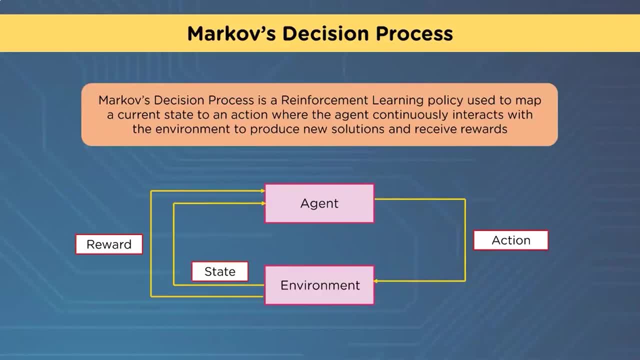 so taking the time to just understand these different pieces as they go is pretty important in most of the models today, and so a lot of them actually have templates. based on this, you can pull in and start using pretty straightforward as far as, once you start seeing how it works, you can see your environment, since it says: 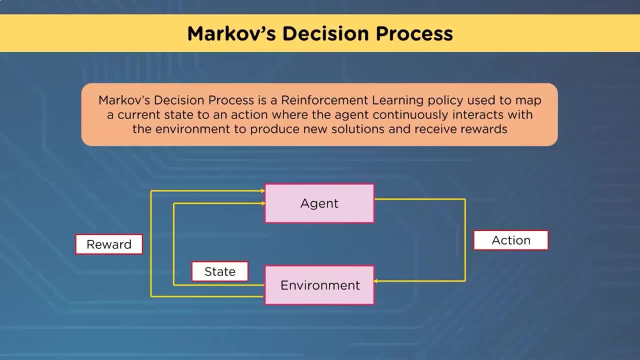 hey, this is what the agent did. this: if your character in the game this happened and it shoots at a reward in a state, the agent looks at the reward, looks at what the agent did, takes a reward before processing this all at once and then全部ul and looks at this values and so you get those key leads that come in: unique one to search for the materials that are needed for a reward list. 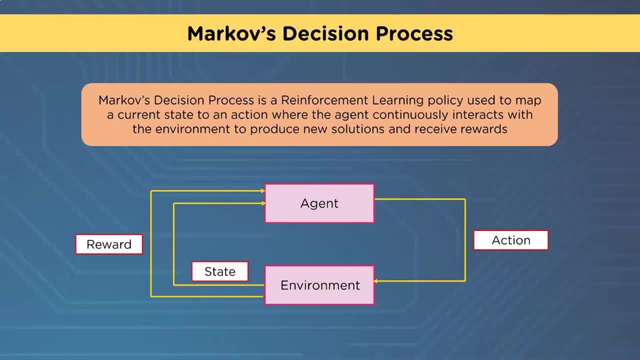 a new state and then takes a little guess and says I'm going to try this action. And then that action goes back into the environment. It affects the environment. The environment then changes depending on what the action was, And then it has a new state and a new reward that goes back to the 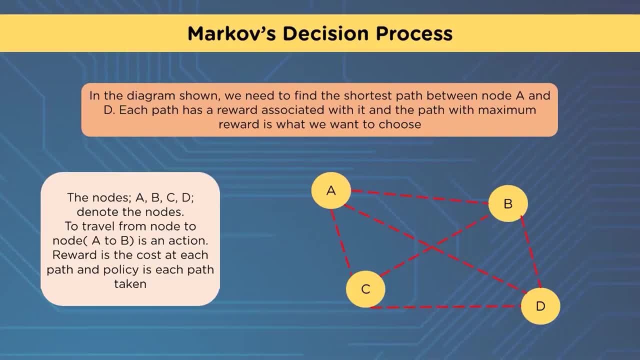 agent. So in the diagram shown we need to find the shortest path between node A and D. Each path has a reward associated with it and the path with a maximum reward is what we want to choose. The nodes A, B, C, D denote the nodes. to travel from node A to B is an action. Reward is a cost. 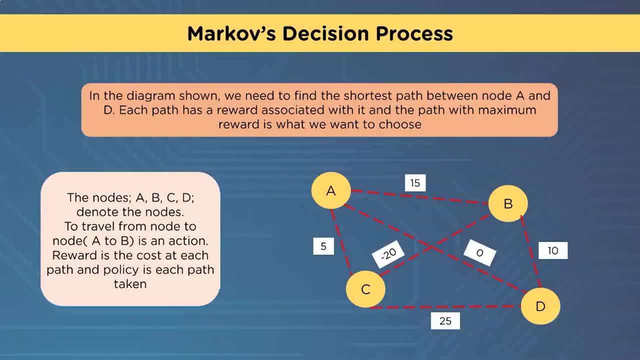 of each path and policy is each path taken, And you can see here: A can go to B, or A can go to C right off the bat, or it can go right to D, And if you explored all three of these you would find. 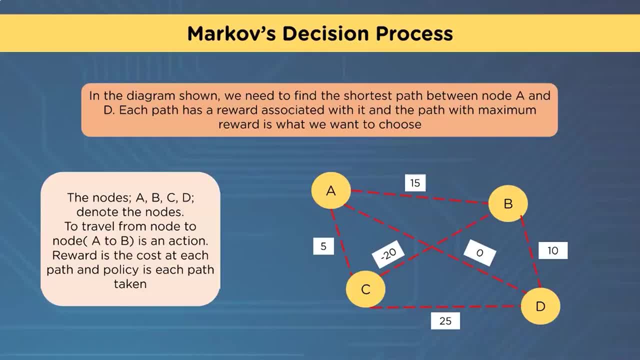 that A going to D was a zero reward. A going to C and D would generate a different reward. or you could go A going to C and D would generate a different reward, or you could go A going to D. going to A going to D. 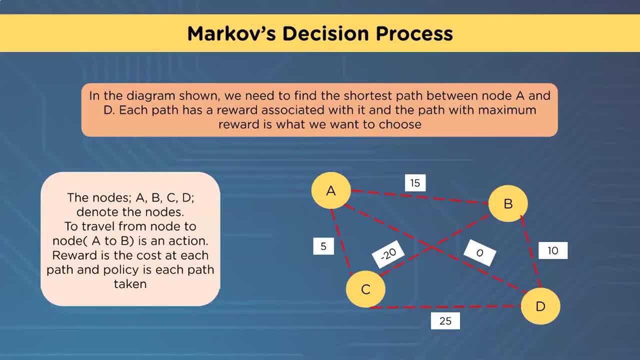 A, C, B, D. There's a lot of options here, And so when we start looking at this diagram, you start to realize that, even though today's reinforced learning models do really good at finding an answer, they end up trying almost all the different directions, you see, And 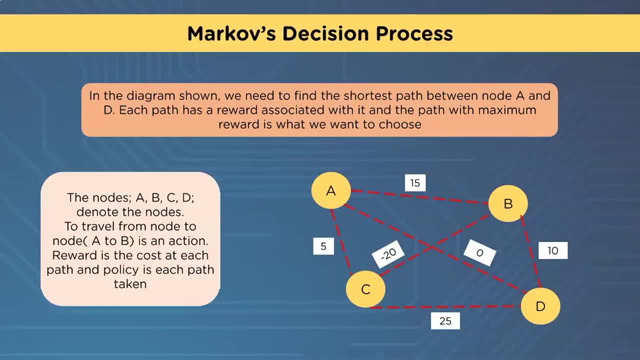 so they take up a lot of work or a lot of processing time for reinforcement learning. They're right now in their infant stage and they're really good at solving simple problems, And we'll take a look at one of those in just a minute in a tic-tac-toe game. But you can 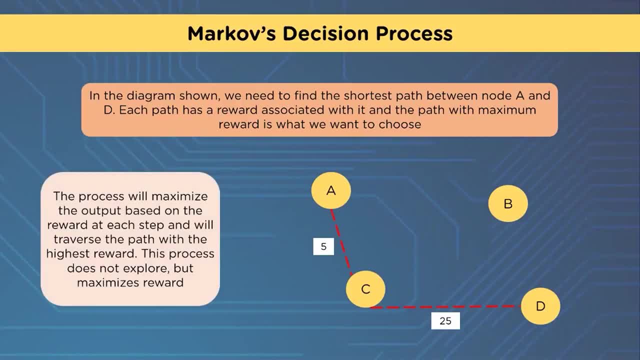 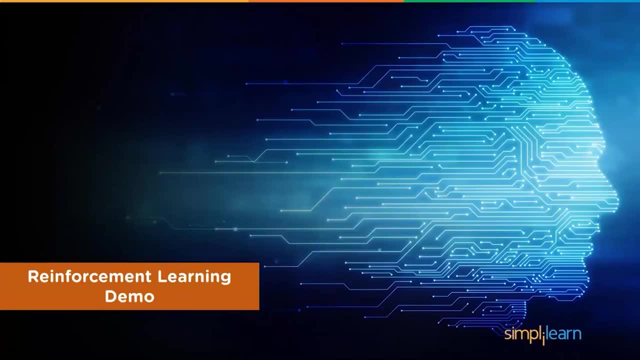 see here. once it's gone through these and it's explored, it's going to find the A, C, D is the best reward. It gets a full 30 points for it. So let's go ahead and take a look at a reinforcement learning demo. In this demo we're going to use reinforcement learning. 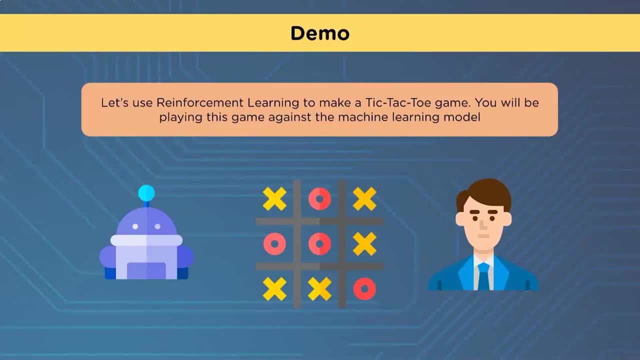 to make a tic-tac-toe game. You will be playing this game against the machine learning model And we'll go ahead. we're doing it in Python, So let's go ahead and take a look. We're going to take a look at a reinforcement learning. 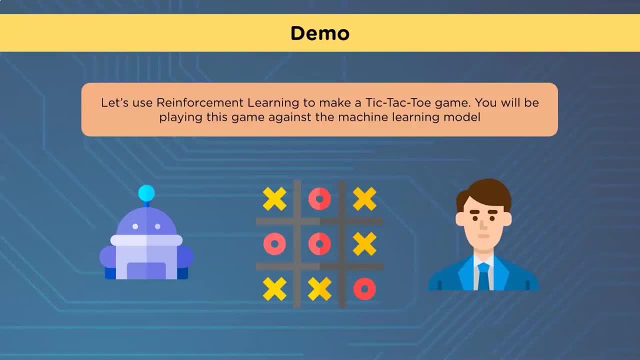 ahead and go through my always- not always- I actually have a lot of Python tools. Let's go through Anaconda, which will open up a Jupyter notebook. Seems like a lot of steps, but it's worth it to keep all my stuff separate and it also has a nice display when you're in the Jupyter. 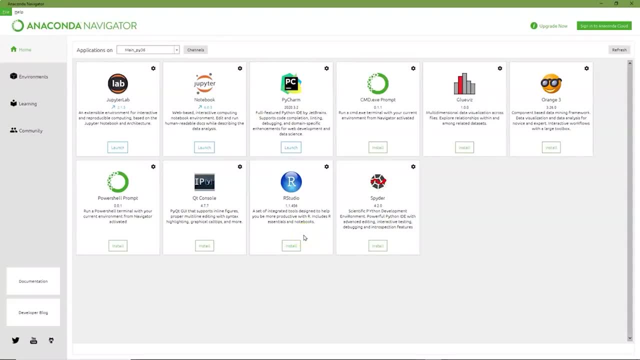 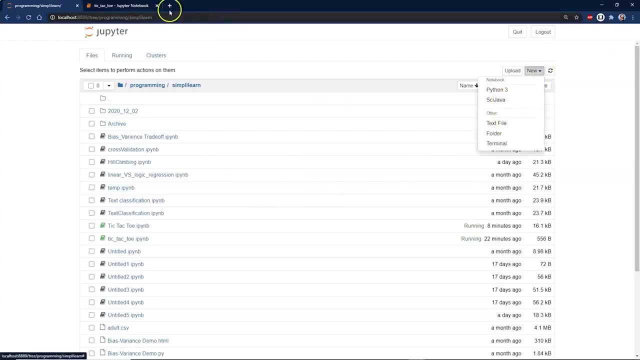 notebook for doing Python. So here's our Anaconda navigator. I open up the notebook, which is going to take me to a web page, and I've gone in here and created a new Python folder- In this case I've already done it- and enabled it to change the name to tic-tac-toe, And then for this example: 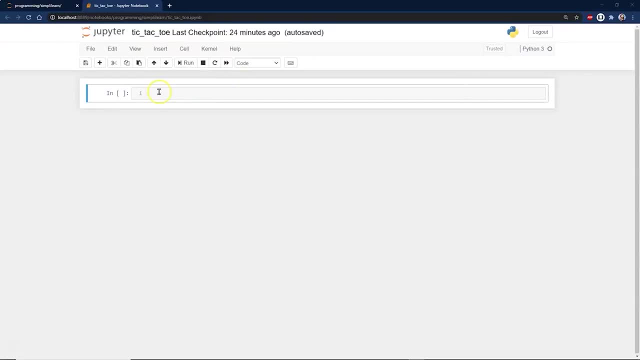 we're going to go ahead and import a couple things. We're going to import numpy as np. We'll go ahead and import pickle- Numpy of course is our number array- and then pickle is just a nice way sometimes for storing different information, different states that we're going to go through. 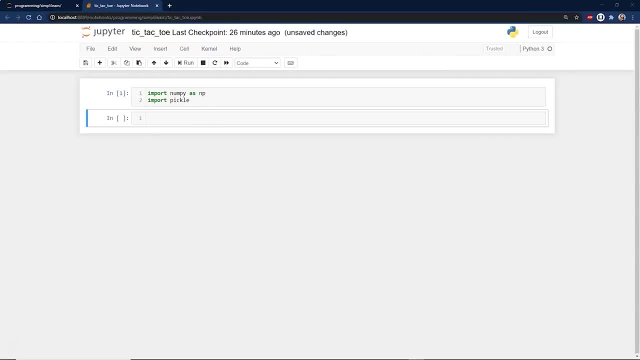 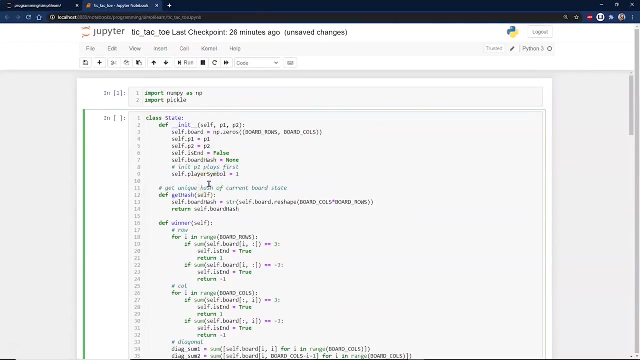 on here, And so we're going to create a class called state. We're going to start with that, And there's a lot of lines of code to this class that we're going to put in here. Don't let that scare you too much. There's not as much here. It looks like there's going to be a lot here. 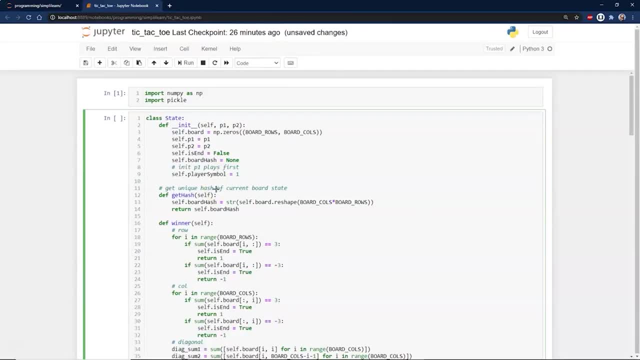 but there really is just a lot of setup going on in our class state And so we have up here, we're going to initialize it. We have our board. It's a tic-tac-toe board, so we're only dealing with nine spots on the board. We have player one, player two, player three, player four, player five. 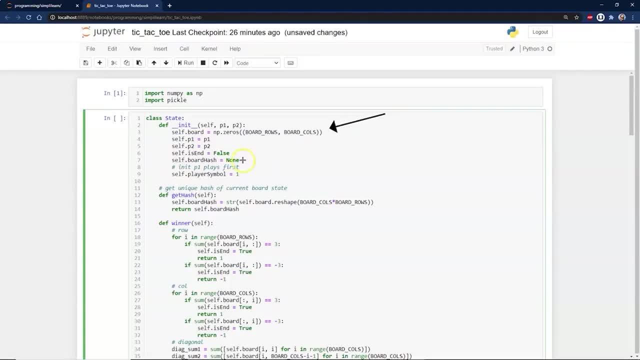 player two is end. We're going to create a board hash. We'll look at that in just a minute. We're just going to store some information in there. Symbol of player equals one. So there's a few things going on as far as the initialization. Then something simple we're just going to get. 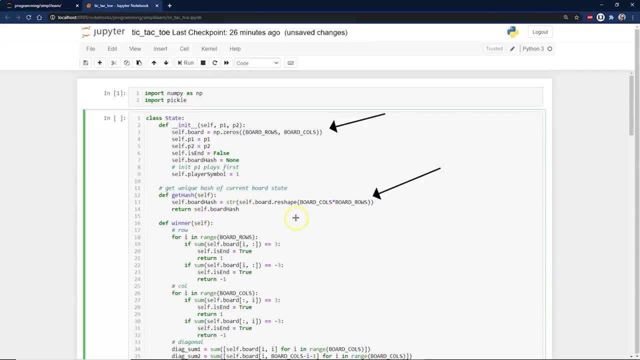 the hash of the board. We're going to get the information from the board on there, which is columns and rows. We want to know when a winner occurs, So if you get three in a row, that's what this whole section here is for. 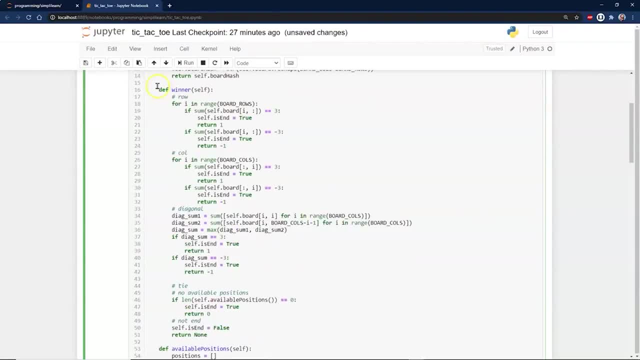 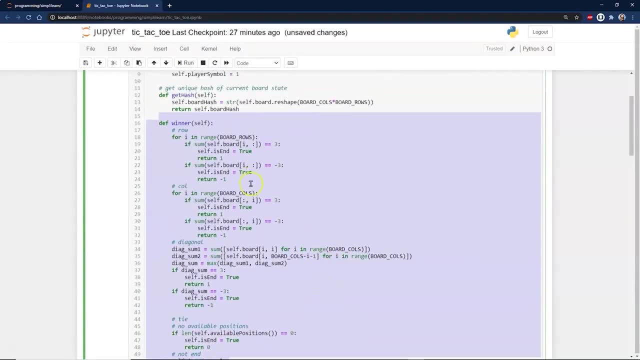 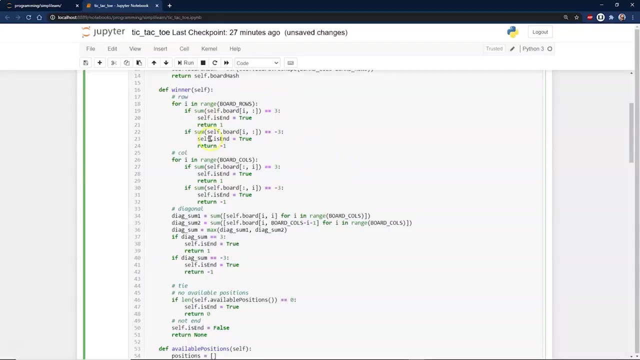 Let me go ahead and scroll up a little bit And you can get a copy of this code. if you send a note over to Simply Learn. We'll send you over this particular file and you can play with it yourself and see how it's put together. I don't want to spend a huge amount of time on this, because this 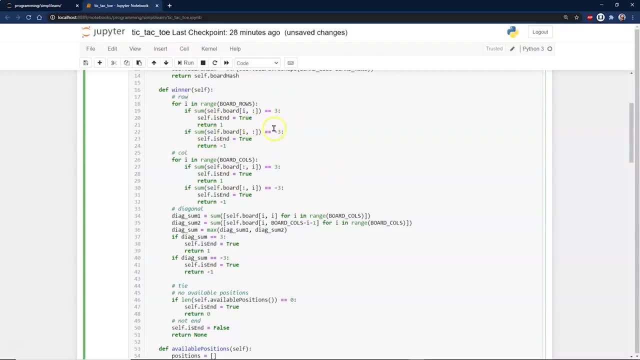 is just some real general Python coding. But you can see, here we're just going through all the rows and you add them together and if it equals three, three in a row, Same thing with columns Diagonal, so you've got to check the diagonal. That's what all this stuff does here, is it? 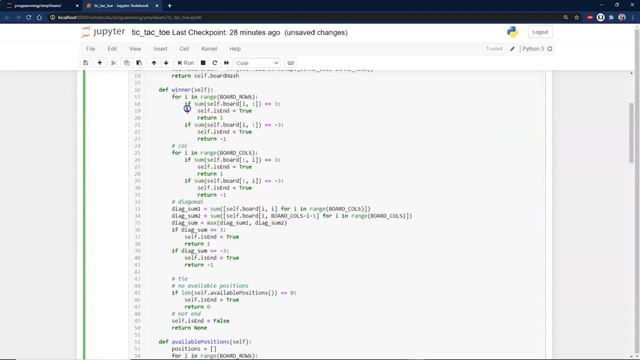 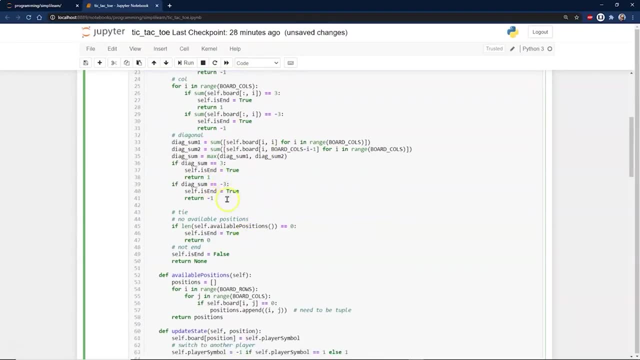 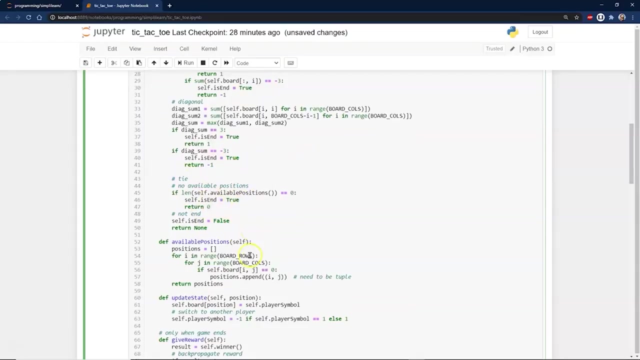 just goes through the different areas. Actually, let me go ahead and put there we go, And then it comes down here and we do our sum and it says true, minus three. It just says: did somebody win or is it a tie? So you've got to add up all the numbers on there anyway, just in case they're all. 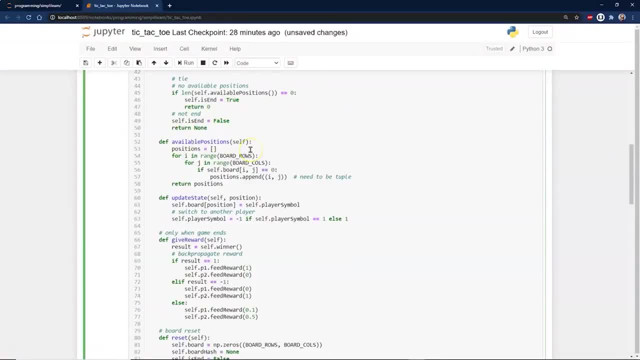 filled up, And next we also need to know available positions. These are ones that don't no one's ever used before. This way, when you try something or the computer tries something, it's not going to give it an illegal move. That's what the available positions is doing. Then we want to update our 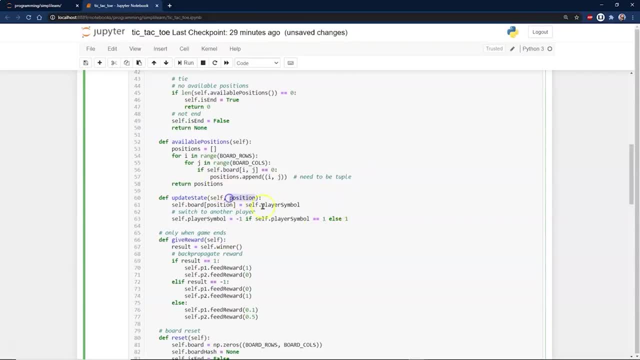 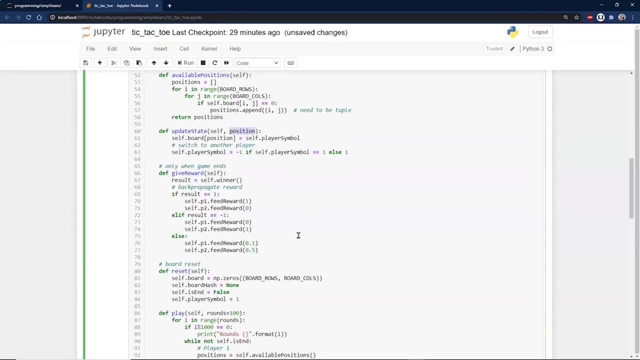 state and so you have your position going in. We're just sending in the position that you just chose and you'll see there's a little user interface we put in there. We can pick the row and column in there And again I mean, this is a lot of code, so really. 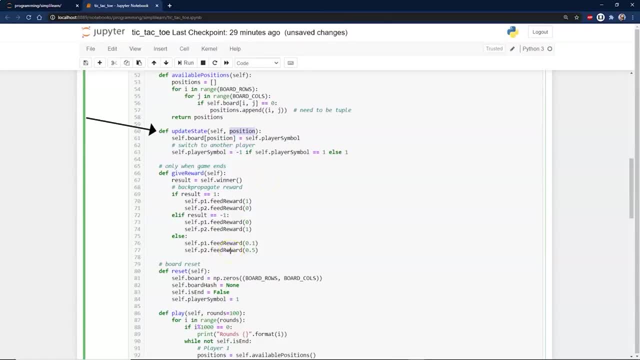 it's kind of a thing you'd want to go through and play with a little bit and just read through it, get a copy of it- A great way to understand how this works. And here is a given reward. So we're going to give a reward. result equals self winner. This is one of the hearts of what's. 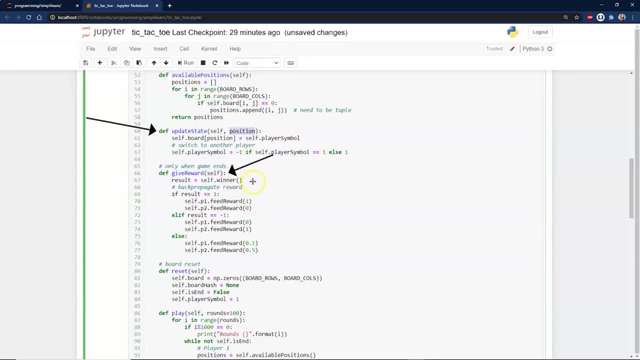 going on here is: we have a result selfwinner. So if there's a winner, then we have a result If the result equals one. here's our feedback. If it doesn't equal one, then it gets a zero. So it only gets a reward in this particular case if it wins, And that's important to know. 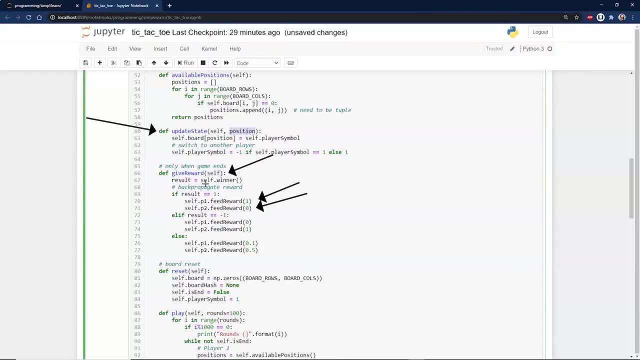 because different systems of reinforced learning do rewarding a lot differently, depending on what you're trying to do. This is a very simple example with a three by three board. Imagine if you're playing a video game. certainly, you only have so many actions, but your environment? 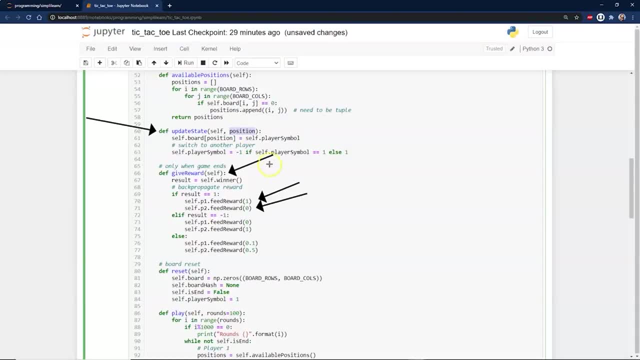 is huge. You have a lot going on in the environment And suddenly a reward system like this is going to be just. it's going to have to change a little bit. It's going to have to have different rewards and different setup, And there's all. 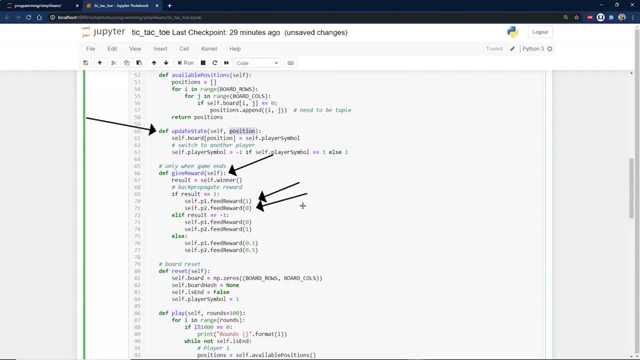 kinds of advanced ways to do that. as far as weighing, you add weights to it, And so they can add the weights up, depending on where the reward comes in. So it might be that you actually get a reward. In this case, you get the reward at the end of the game, And I'm 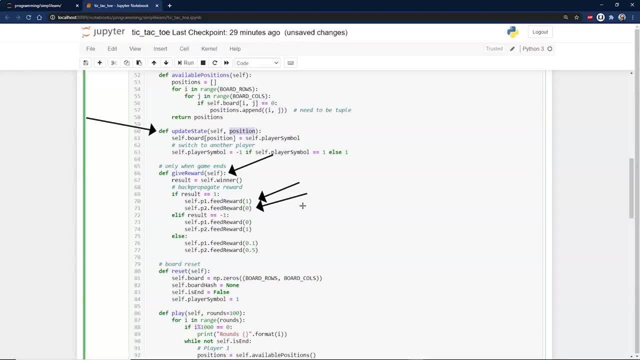 spending just a little bit of time on this, because this is an important thing to note. But there's different ways to add up those rewards. So if you're playing a video game, it might have like, if you take a certain path, the first reward is going to be weighed. 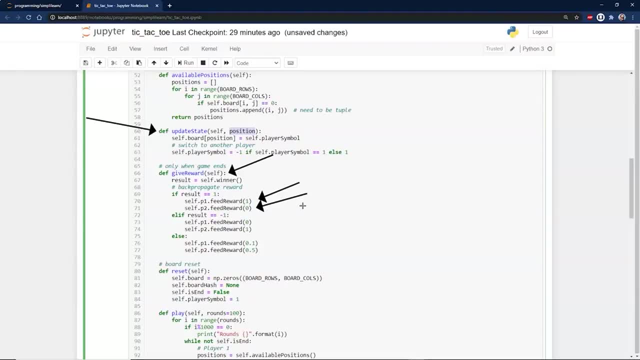 a little bit less than the last reward, because the last reward is actually winning the game or scoring, or whatever it is, So this reward system gets really complicated in some of the more advanced setups. In this case, though, you can see right here that they give a point. 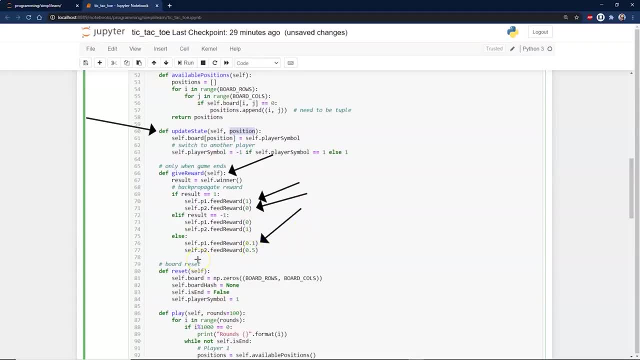 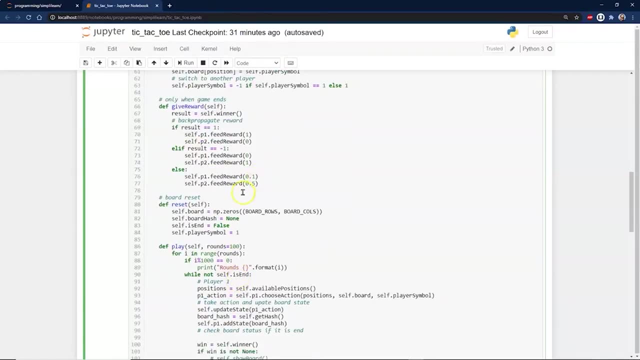 one and a point five: reward just for getting a, picking the right value And something that's actually valid, instead of picking an invalid value. So rewards again, that's like key, It's huge. How do you feed the rewards back in? Then we have a board. 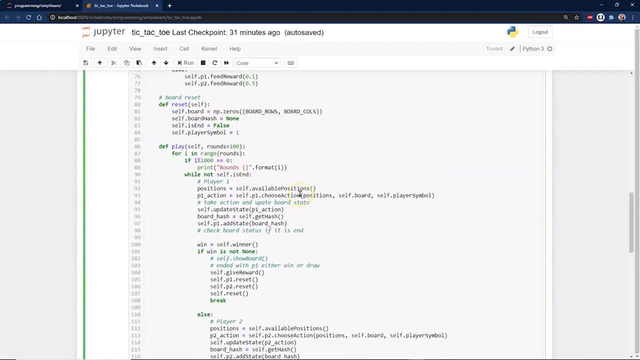 reset. That's pretty straightforward. It just goes back and resets the board at the beginning, because it's going to try out all these different things while it's learning. It's going to do it by trial and error, So you have to keep resetting it. And then, of course, there's 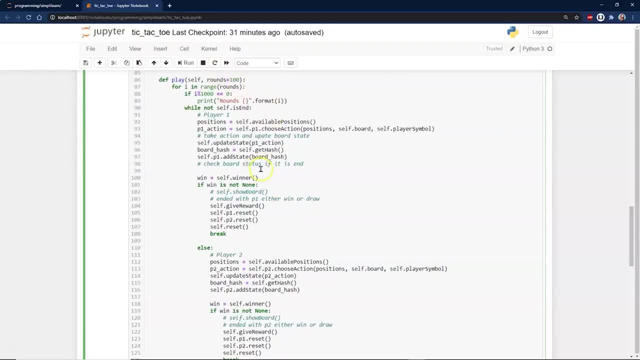 the play. We want to go ahead and play rounds equals 100.. Depends on what you want to do on here. I'm going to set this different, obviously, set that to higher level, But this is just going to go through and you'll see in here that we have player one and player two. This 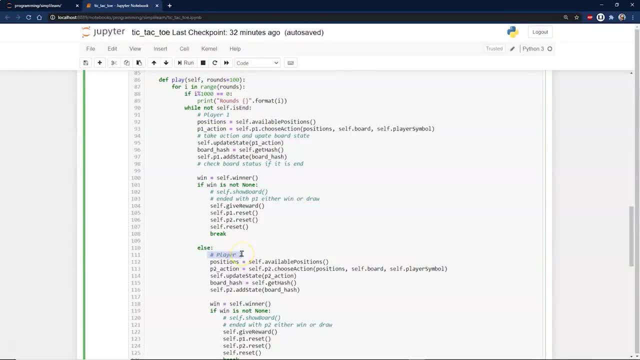 is the computer playing itself. One of the more powerful ways to learn to play a game, or even learn something that isn't a game, is to have two of these models that are basically trying to beat each other, And so they keep finding, explore new things. This one works. 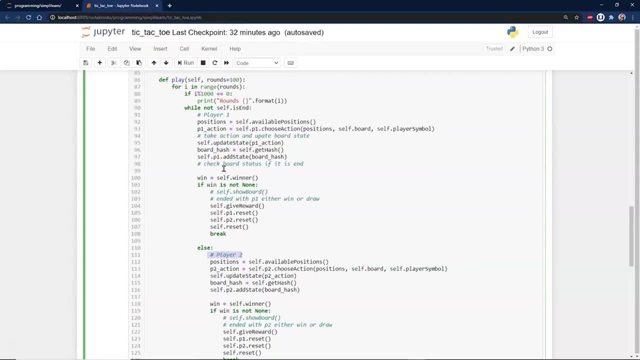 for this one. So this one tries new things. It beats this. We've seen this in chess. I think was a big one where they had the two players in chess with reinforcement learning. It was one of the ways they trained one of the top computer chess playing algorithms. 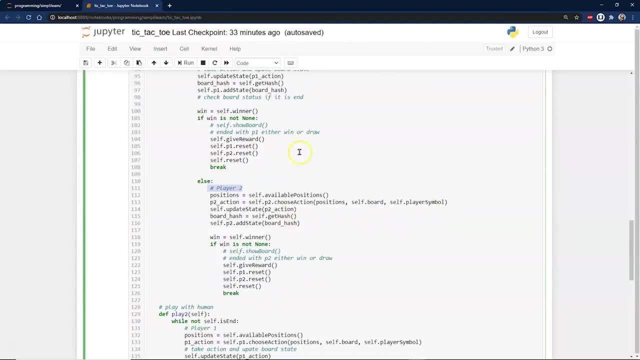 So this is just what this is. It's going to choose an action, It's going to try something, And the more it tries stuff, the more we're going to record the hash. We actually have a board hash where you can yourself get the hash set up on here where it stores all the 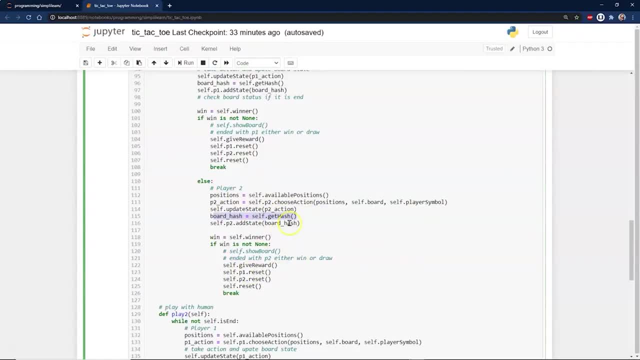 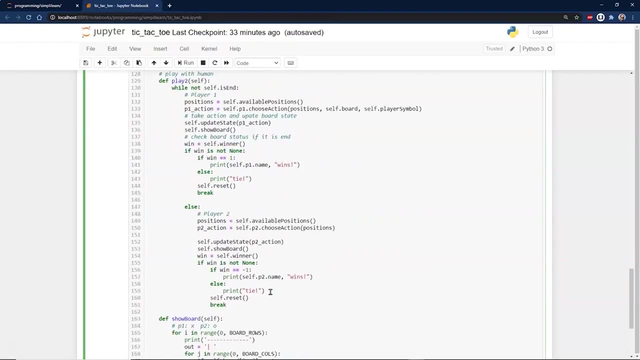 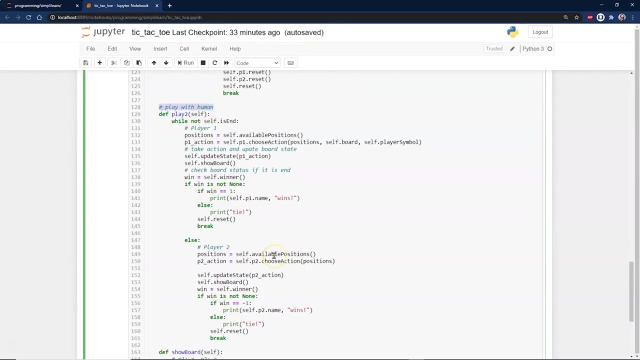 information And then once you get to a win- one of them wins It gets the reward. Then we go back and reset and try again And then kind of the fun part we actually get down here is we're going to play with a human, So we'll get a chance to come in here and see what that looks like when you 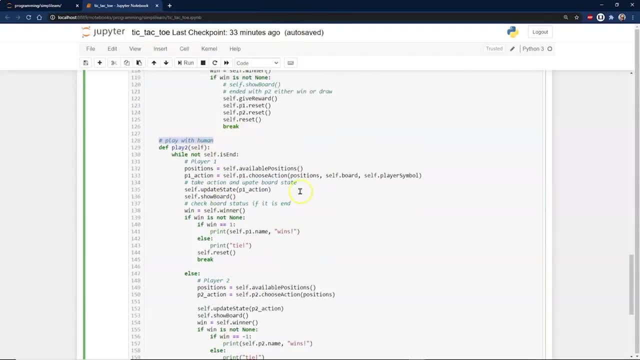 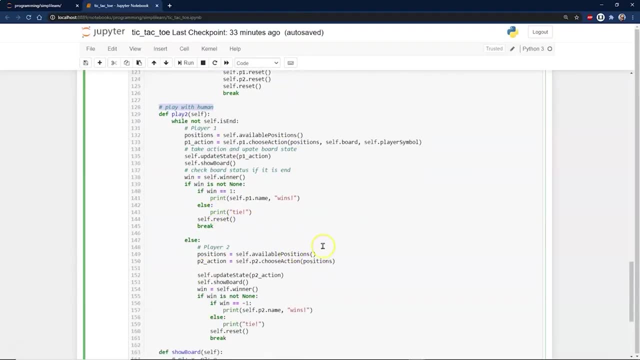 put your own information in, And then it just comes in here and does the same thing it did above. It gives it a reward for its things, or sees if it wins or ties, looks at available positions, all that kind of fun stuff, And then, finally, we want to show the board. So 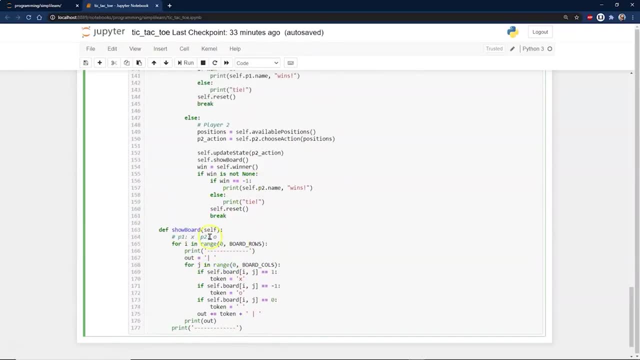 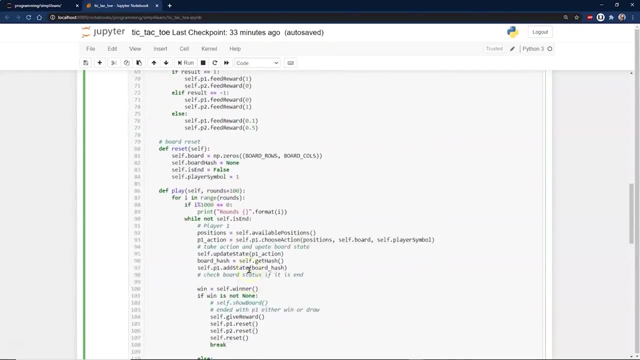 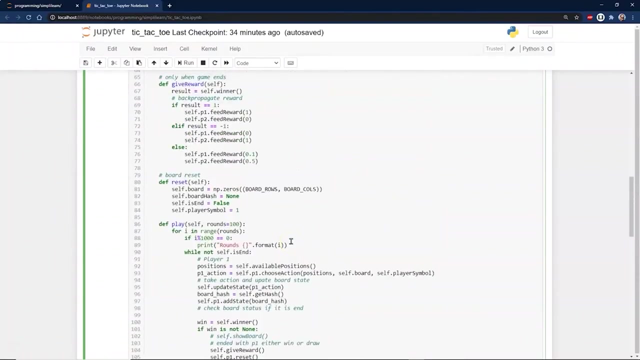 it's going to print the board out each time. Really, as an integration is not that exciting. What's exciting in here is one looking at this reward system. Whoops, play one more up. The reward system is really the heart of this. How do you reward the different setup? 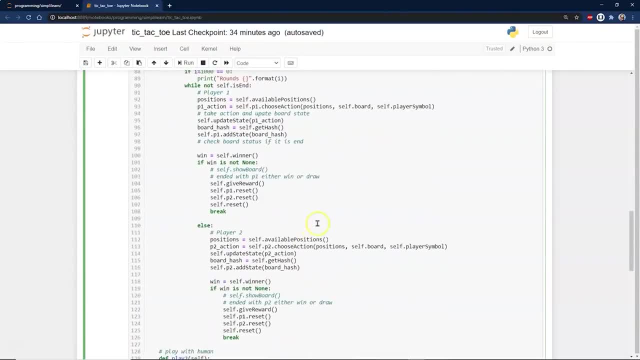 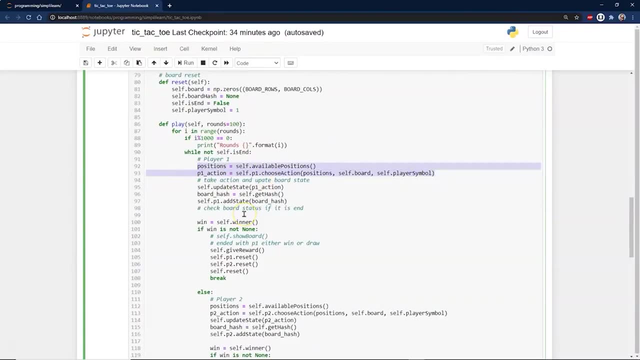 And the other one is when it's playing. it's got to take an action, And so what it chooses for an action is also the heart of reinforcement learning. How do we choose that action? And those are really key to right now. where reinforcement learning is in. today's technology is figuring. 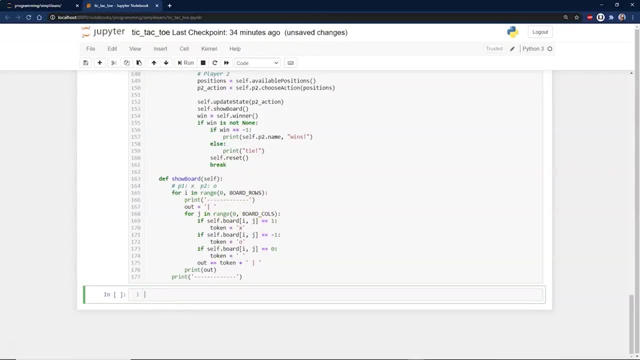 this out, How do we reward it and how do we guess the next best action? So we have our environment and you can see the environment is we're going to be, or the state, which is kind of like what's called the state. So we have our environment and you can see the. 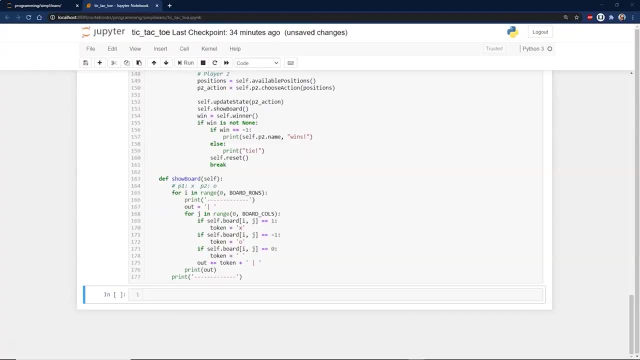 environment is we're going to be or the state, which is kind of like what's called the state. So we have our environment and you can see the environment is we're going to be or the be going on. We're going to return the state, depending on what happens, And we want to. 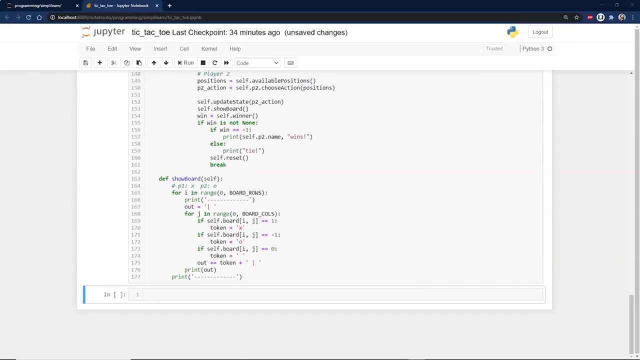 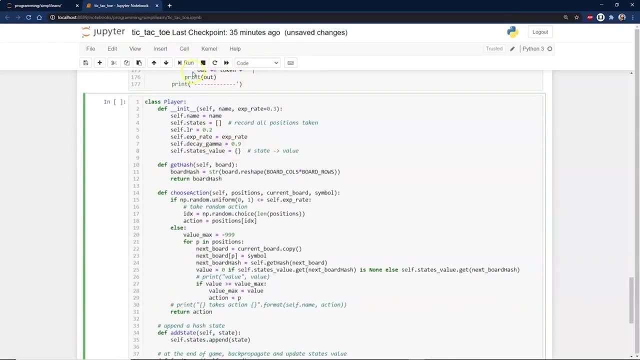 go ahead and create our agent in this place, our player. So each one is… let me go and grab that. And so when we look at a class player, this is where a lot of the magic is really going on. How is this player figuring out how to maneuver around the board And 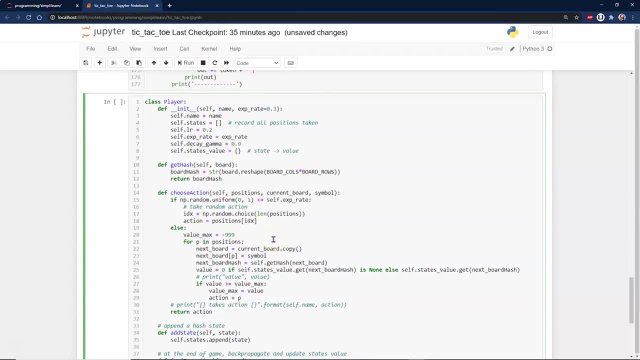 then, of course, the board returns a state that it can look at and reward. So we want to take a look at this. We have name selfstate, repairing, and then we go ahead and create. This is class player, And when you say class player, we're not talking about a human player. 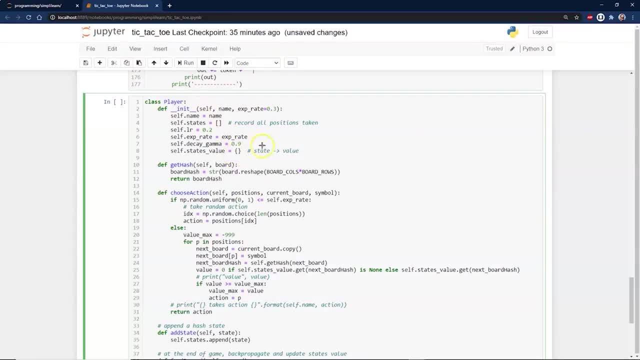 We're talking about just the computer players, And this is kind of interesting. So remember, I told you, depending on what you're doing, there's going to be a decay gamma explore rate. These are what I'm talking about is how do we train it? 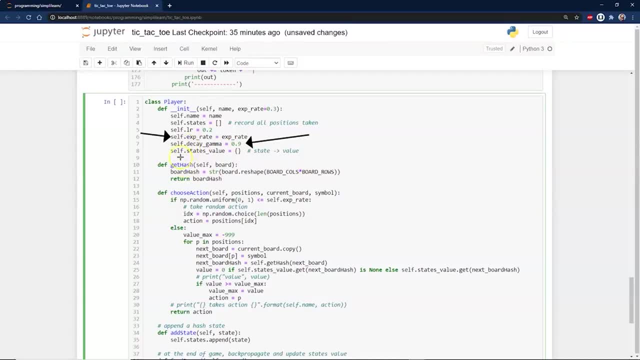 As you try different moves, it gets to the end. The first move is important, but it's not as important as the last one, And so you could say that the last one has the heaviest weight. and then, as you get there, the first one, let's see. 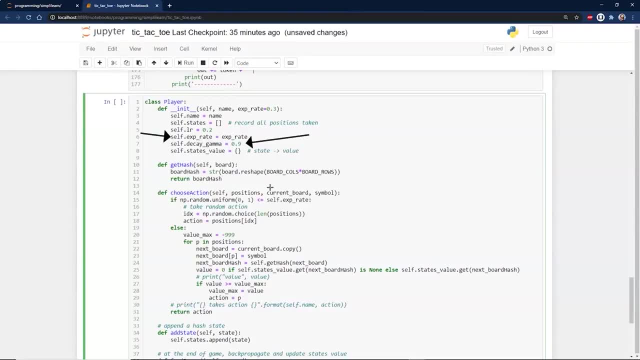 the first move gives you a five reward, the second gives you a two reward and the third one gives you a ten reward. because that's the final ending, You got it. The ten's going to count more than the first step, And here's our. we're going to get the board information coming in. 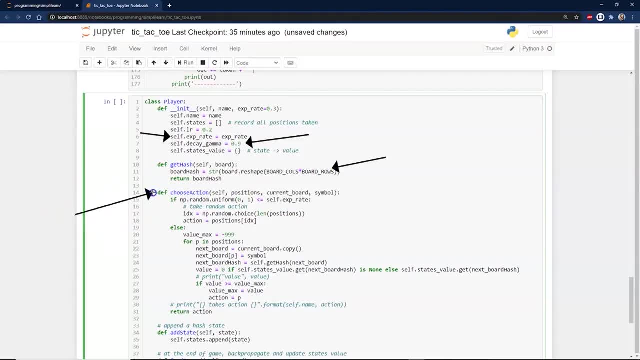 and then choose an action. This was the second part that I was talking about. that was so important. So once you have your training going on, we have to do a little randomness And you can see right here is our NP random uniform. So it's picking out a random number. 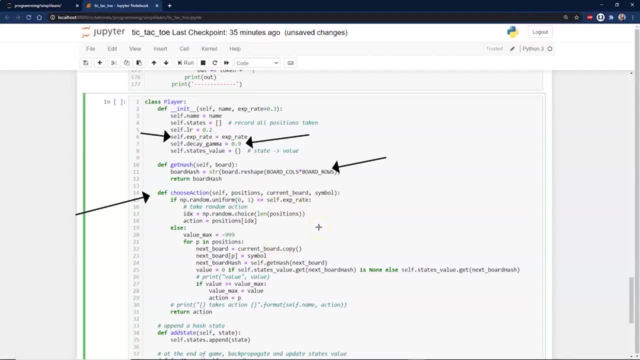 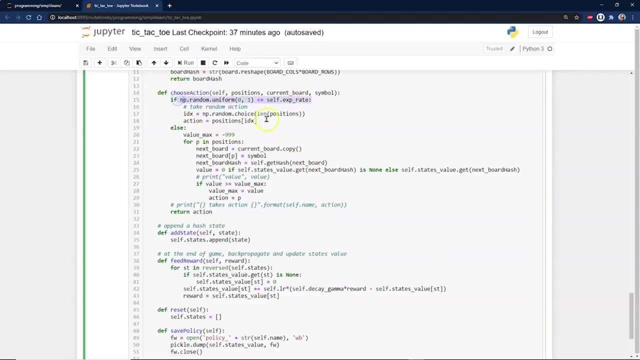 Take a random action. This is going to just pick which row and which column it is, And so choosing the action, this one. you can see we're just doing random states, choice, length of positions, action position. And then it skips in there and takes a look at the board. 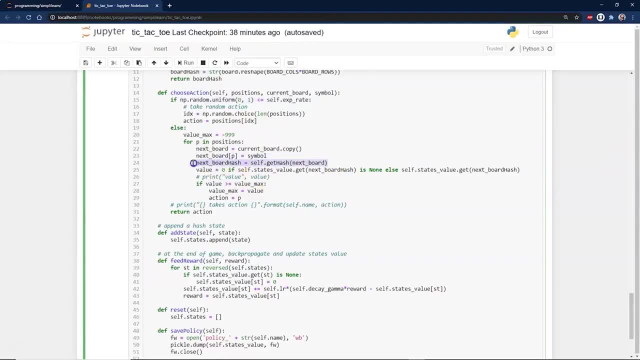 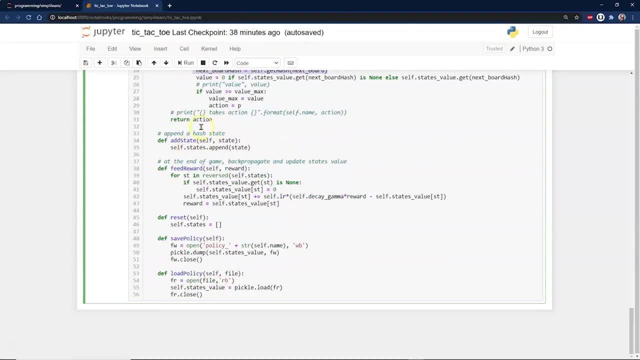 For P and positions. it's actually storing the different boards each time you go through, So it has a record of what it did, so it can properly weigh the values, And this simply just appends a hash state. What's the last state? 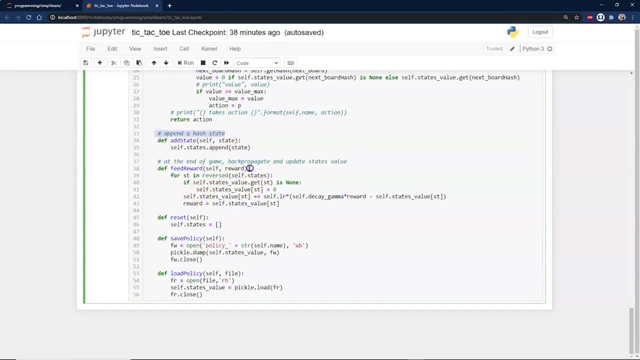 Append it to our states on here. Here's our feedback rewards. The reward comes in and it's going to take a look at this and say: is it none? What is the reward? And here is that formula, Remember I was telling you about up here. 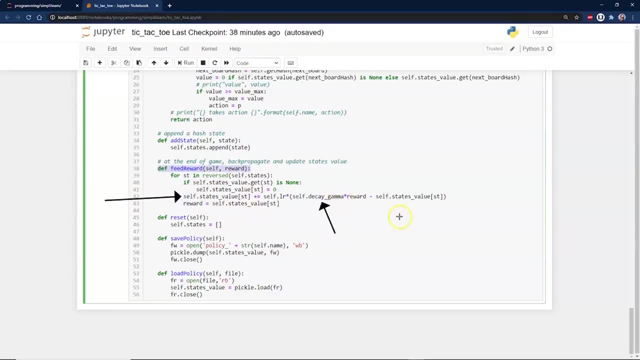 That was important because it has decay gamma times the reward. This is where, as it goes through each step- and this is really important- This is kind of the heart of this, of what I was talking about earlier- You have step one and this might have a reward of two. 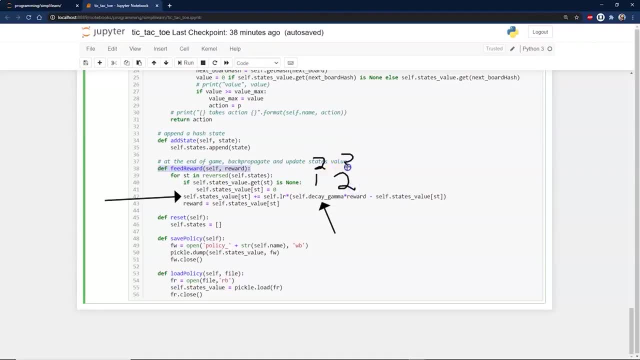 You have step two- I probably should have done ABC. This has a step three, step four and so on, Until you get to step in And this might have a reward of ten. So reward of ten, we're going to add that, but we're not adding. let's say this one right here: 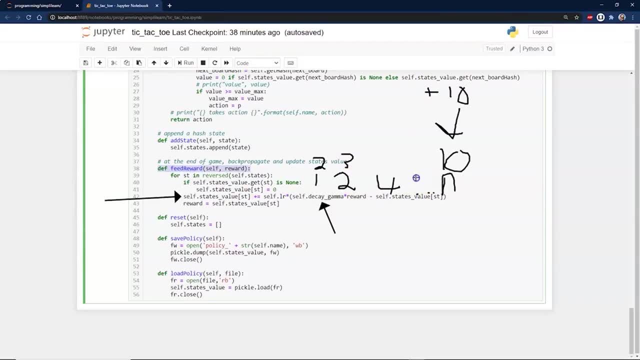 Let's say this reward here, right before ten was, let's say it's also ten. That just makes the math easy. So we had ten and ten. We had ten. this is ten and ten, n whatever it is, But this time it's .9.. 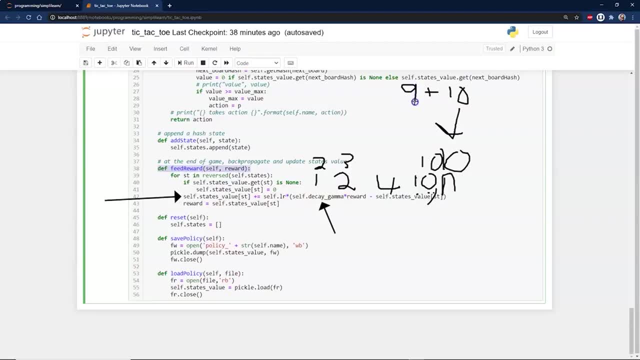 So instead of putting a full ten here, we only do nine. That's .9 times ten, And so this formula as far as the decay times the reward minus the self-state value it basically adds in, it says: here's one or here's two. I'm sorry, I should have done this ABC, it would have been easier. 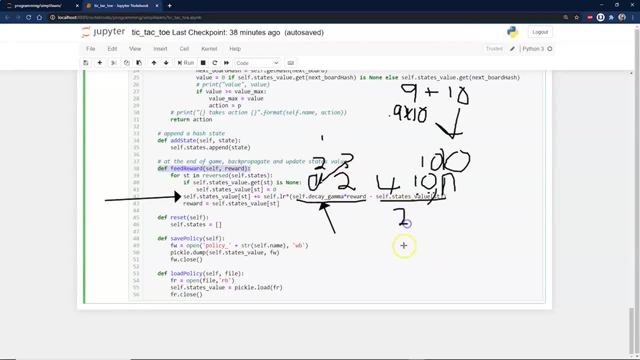 So the first move goes in here and it puts two in here. Then we have our self-setup on here. You can see how this gets pretty complicated in the math. But this is really the key is: how do we train our states, And we want the final state, the win, to get the most points. 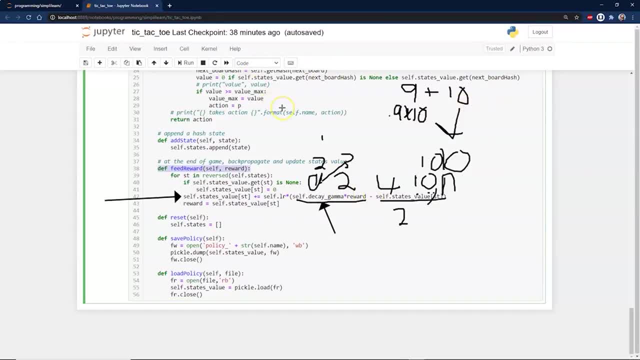 If you win, you get most points, And the first step gets the least amount of points. So you're really training this almost in reverse. You're training it from the last place where you have, like it says: okay, this is now where I need to sum up. 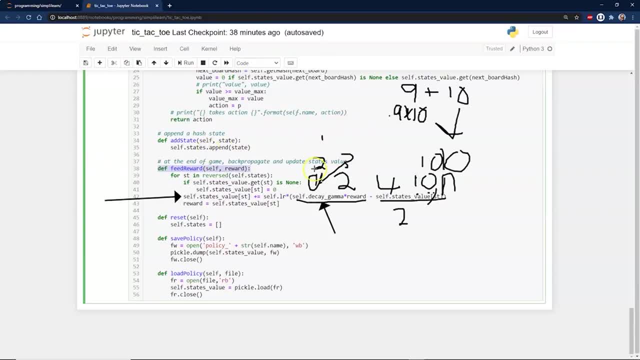 I want to sum up my rewards and I want to sum them up going in reverse, And I want to find the answer in reverse- Kind of an interesting play on the mind when you're trying to figure this stuff out. And of course, we want to go ahead and reset the board down here. save the policy. load policy. 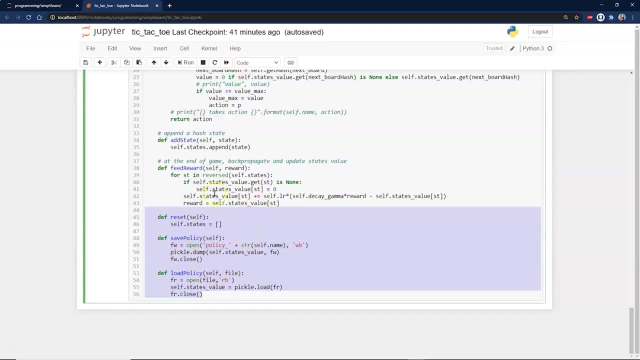 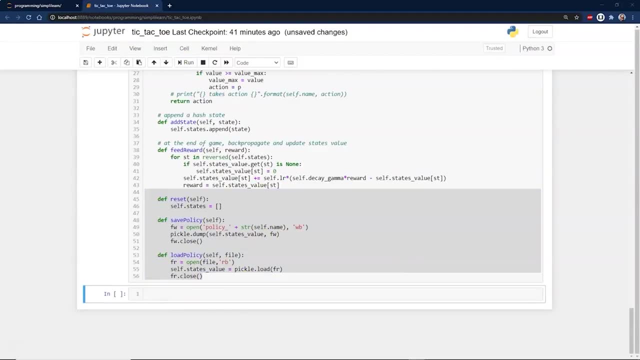 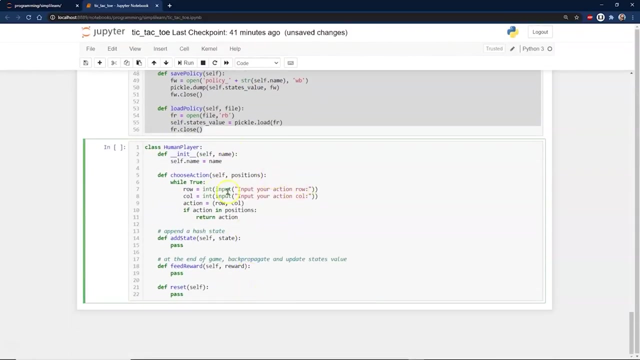 These are the different things that are going in between the agent and the state to figure out what's going on. Let's go ahead and load that up. And then, finally, we want to go ahead and create a human, And the human player is going to be a little different in that you choose an action row and column. 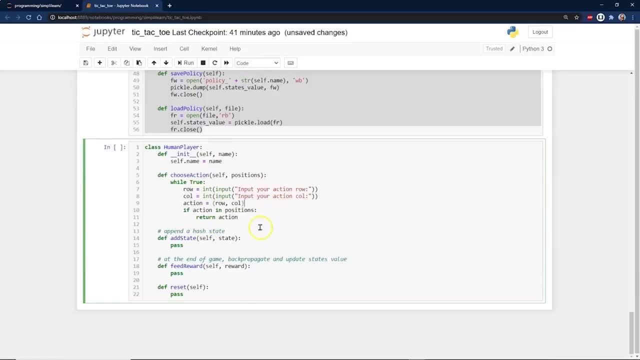 Here's your action: If action is in positions, meaning positions that are available, you return the action. If not, it just keeps asking you until you get an action that actually works, And then we're going to go ahead and append to the hash state, which we don't need to worry about because it returns the action up here. 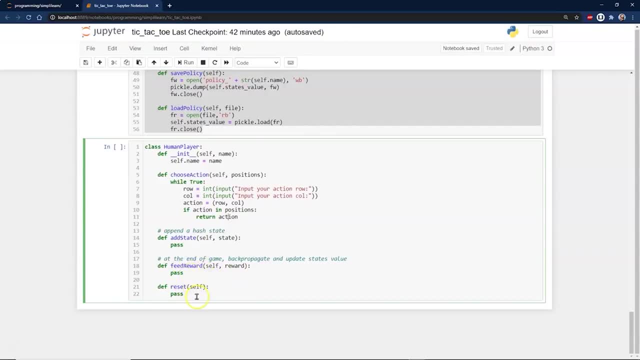 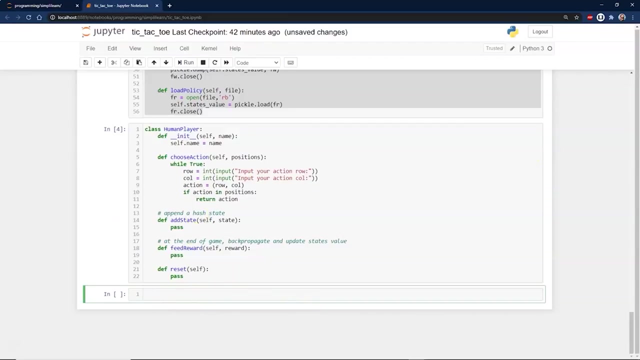 And feed forward- Again, this is because it's a human At the end of the game- bat, propagate and update state values. This part isn't being done because it's not programming the model. The model is getting its own rewards, So we've gone ahead and loaded this in here. 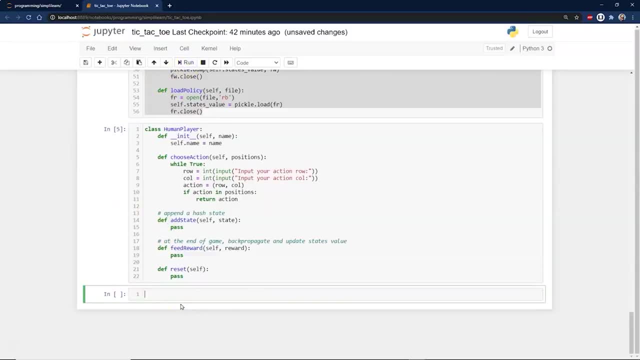 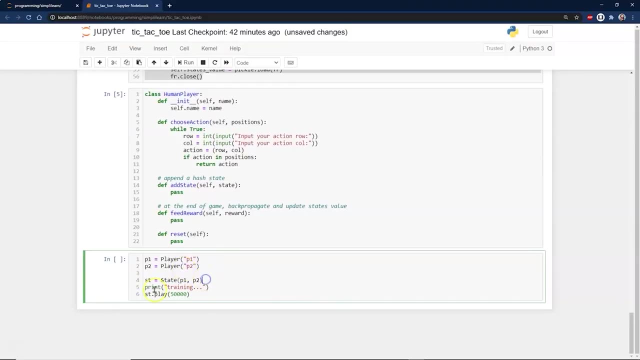 So here's all our pieces, And the first thing we want to do is set up P1, player 1.. P2, player 2.. And then we're going to send our players to our state. So now it has P1, P2.. 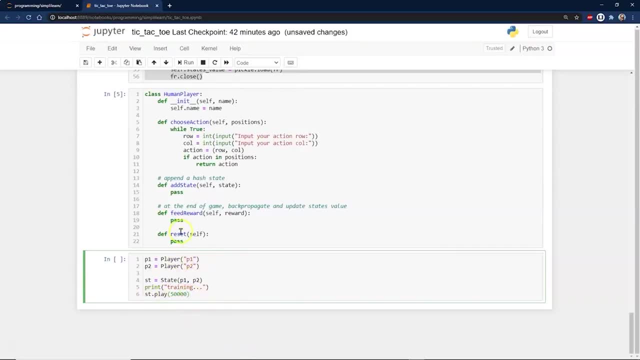 And it's going to play 50,000 rounds. Now, we can probably do a lot less than this, And it's not going to get the full results. In fact, you know what? Let's go ahead and just do 5.. 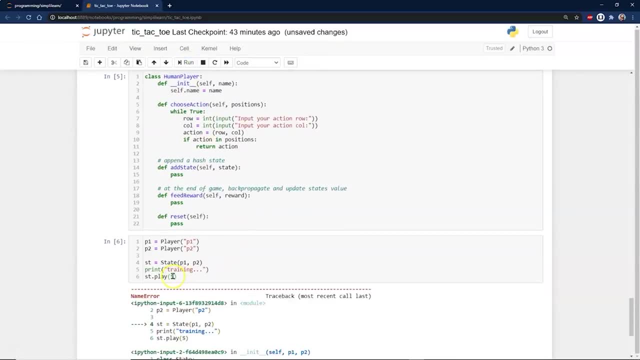 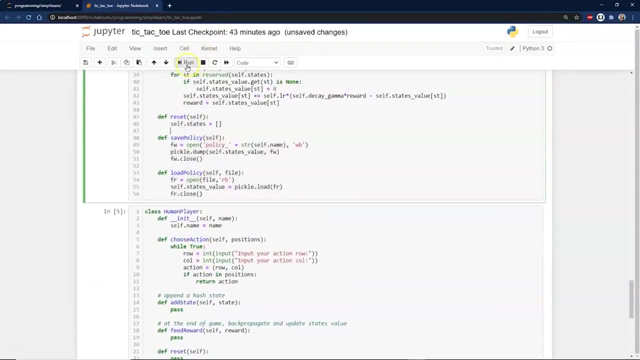 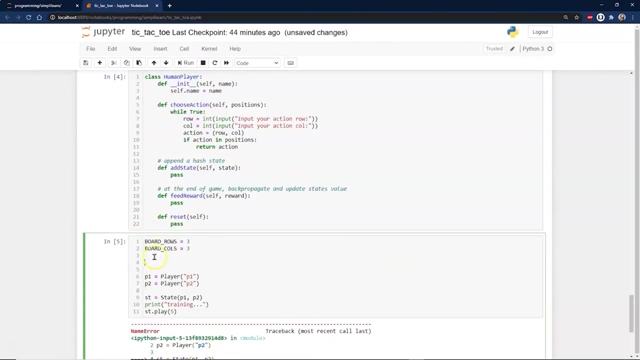 Just to play with it, because I want to show you something here. Oops, Somewhere in there I forgot to load something. There we go. I forgot to run this. There we go, Let's run. Oops, Forgot a reference there for the board rows and columns 3x3.. 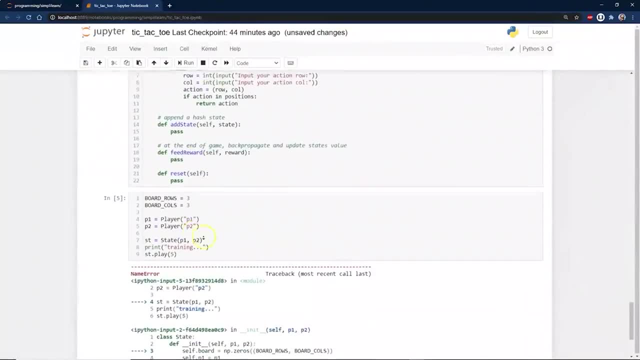 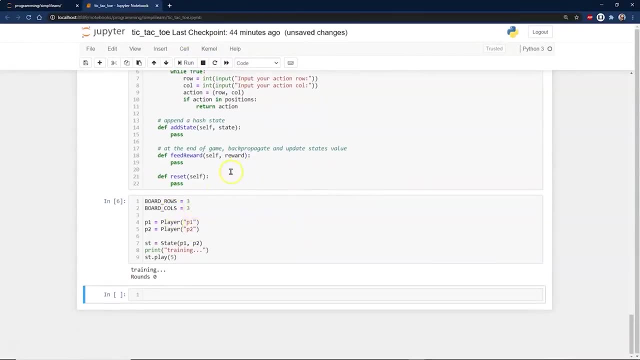 There's actually in the state it references that We can just tack it on on the end. It was supposed to be at the beginning. So now I've only set this up with Let's see Where are we going here. I've only set this up to train 5 times. 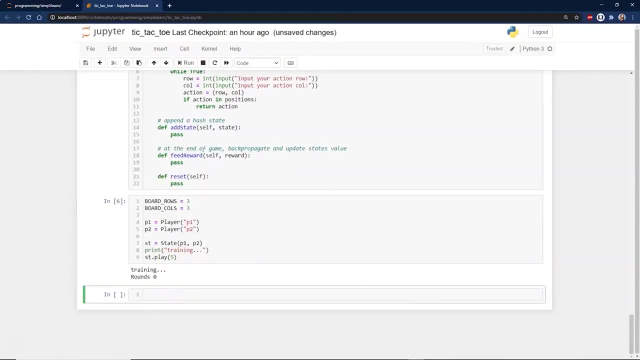 And the reason I did that is we're going to To come in and actually play it And then I'm going to change that And we can see how it differs on there. There we go, And it didn't even make it through a run. 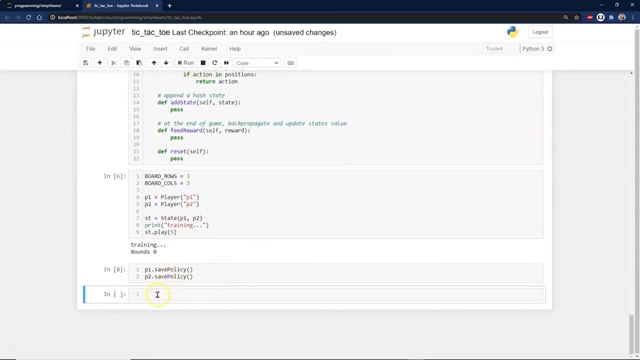 And we're going to go ahead and save the policy. So now we have our Player 1 and our Player 2 policy. The way we set it up, it has two separate policies loaded up in there, And then we're going to come in here and we're going to do: 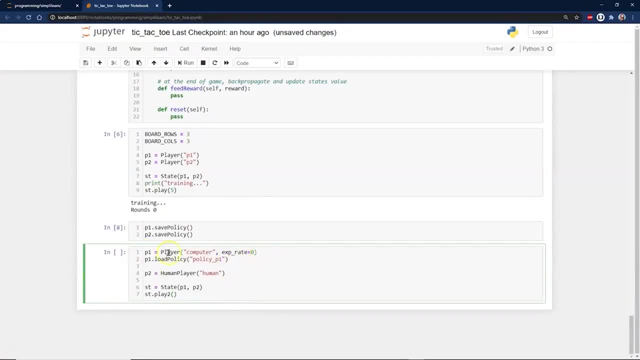 Player 1 is going to be the computer Experience rate 0.. Load policy: 1. Human player: human, And we're going to go ahead and play this Now. remember, I only went through it. just one round of training, In fact, minimal training. 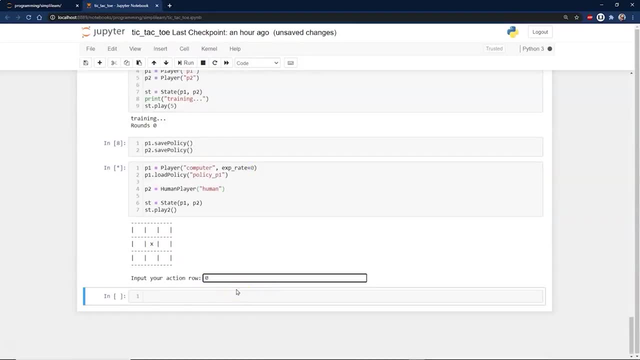 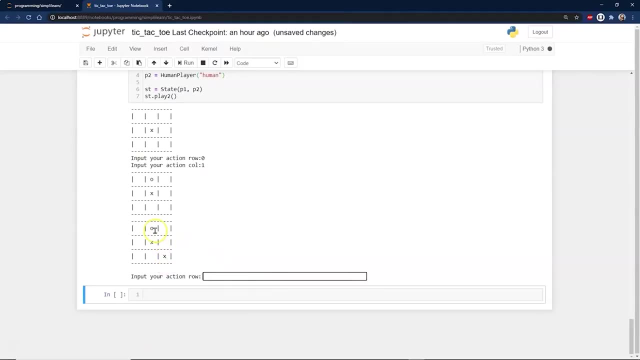 And so it puts an x there And I'm going to go ahead and do row 0,, column 1. And you can see this is very basic on here, And so I put in my 0. And then I'm going to go 0, block it. 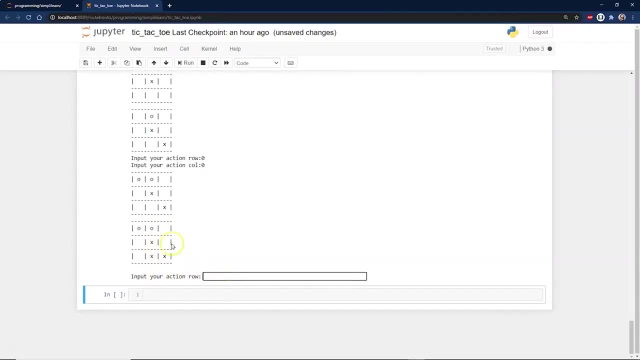 0, 0. And you can see right here it: let me win. Just like that, I was able to win 0. 2.. And Whoo, Human wins. So I only trained it five times. We're going to run this again. 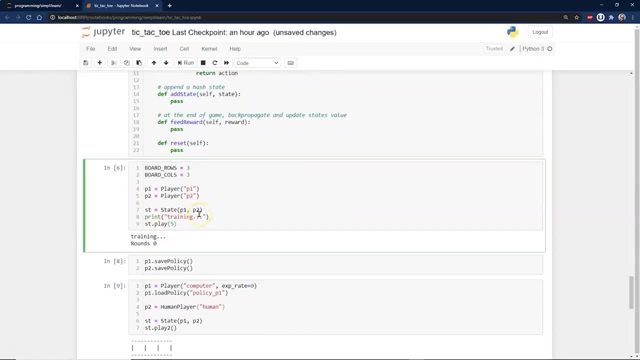 And this time, instead of 5, let's do 5,000 or 50,000.. I think that's what the guys in the back had, And this takes a while to train it. This is where reinforcement learning really falls apart. 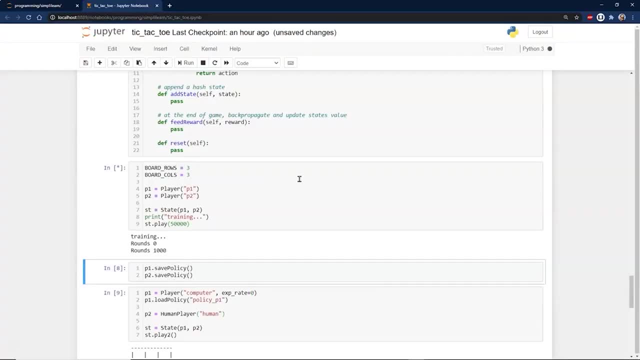 Look how simple this game is. We're talking about a 3x3 set of columns, And so for me to train it on this, I could do a cue table which would go much quicker. You could build a quick cue table with almost all the different options on there. 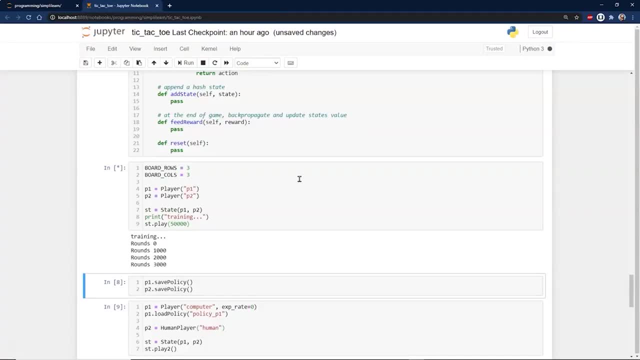 And you would probably get the same result much quicker. We're just using this as an example. So when we look at reinforcement learning, you need to be very careful what you apply it to. It sounds like a good deal until you do like a large neural network. 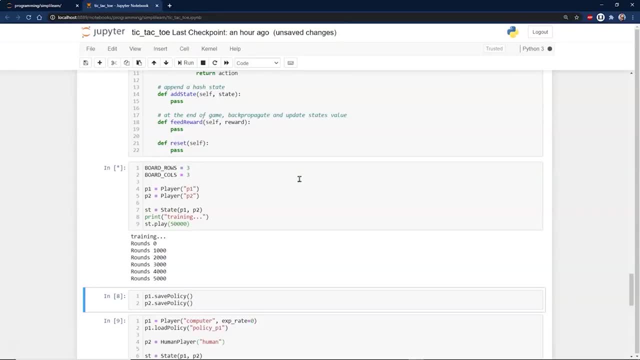 where you set the neural network to a learning increment of one, So every time it goes through it learns. And then you do your actions. You pick from the learning setup And you actually try actions on the learning setup until you get what you think is going to be the best action. 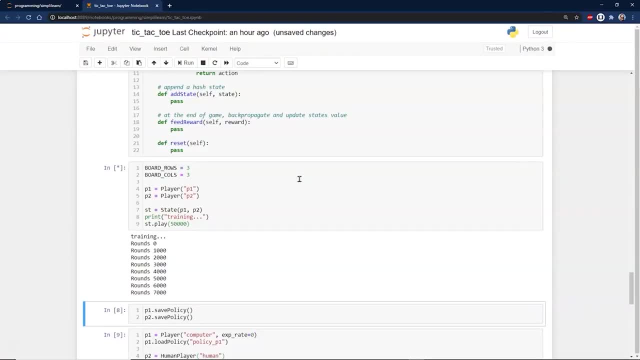 So you actually feed what you think is right back through the neural network. There's a whole, There's a whole layer there which is really fun to play with, And then it has an output. Well, think of all those processes. I mean that is just a huge amount of work it's going to do. 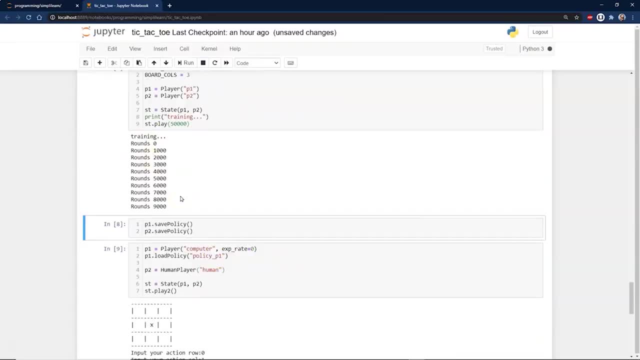 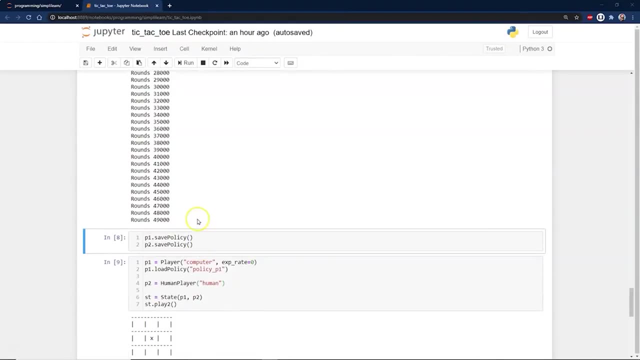 Let's go ahead and skip ahead here. Give it a moment. It's going to take a minute or two to go ahead and run Now to train it. we went ahead and let it run And it took a while. This took. 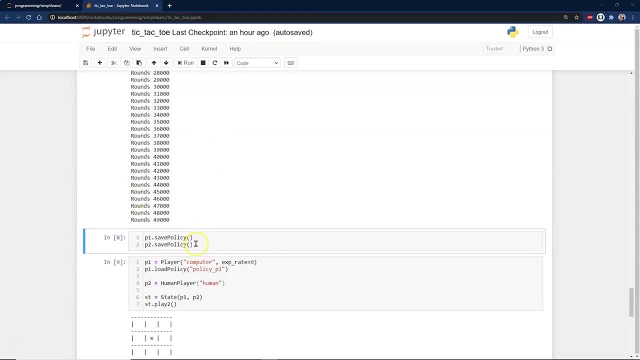 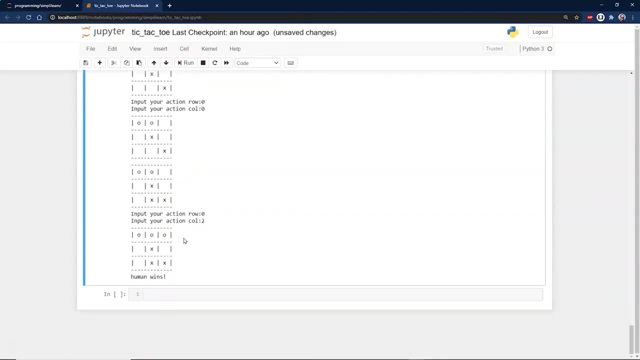 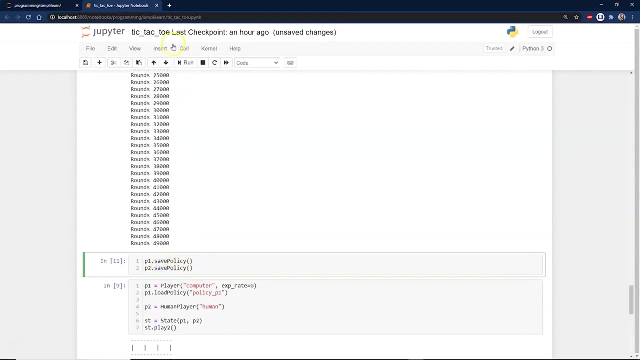 I got a pretty powerful processor and it took about five minutes plus to run it, And we'll go ahead and run our player setup on here. Whoops, it brought in the last. Whoops, it brought in the last round. So give me just a moment to redo the policy save. 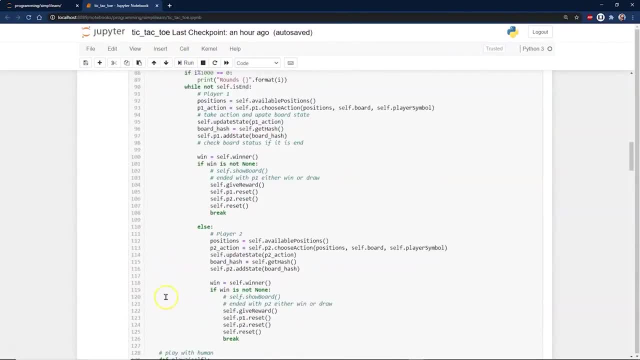 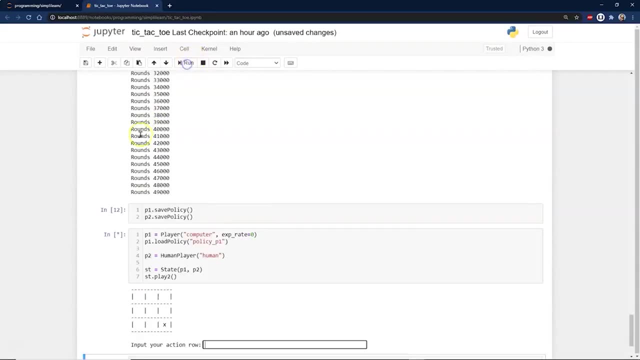 There we go. I forgot to save the policy back in there And then go ahead and run our player again. So we've saved the policy. Then we want to go ahead and load the policy for P1 as a computer And we can see the computer's gone. 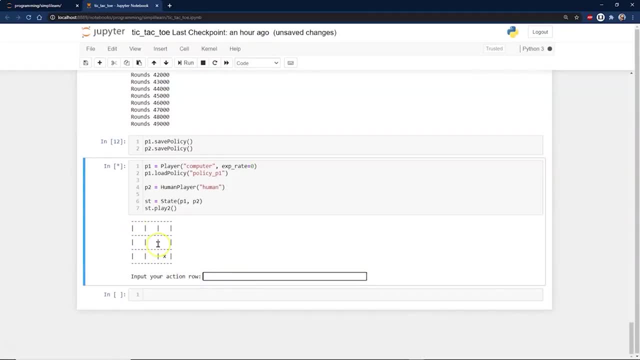 to the bottom right corner. I'm going to go ahead and go 1, 1,, which is the center, And it's gone right up the top And if you've ever played tic-tac-toe you know the computer has me. 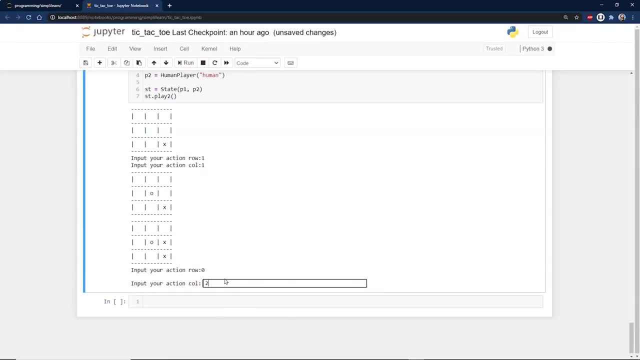 But we'll go ahead and play it out. Row 0, column 2.. There it is, And then it's gone here, And so I'm going to go ahead and go row 0, 1, 2.. No 0, 1.. 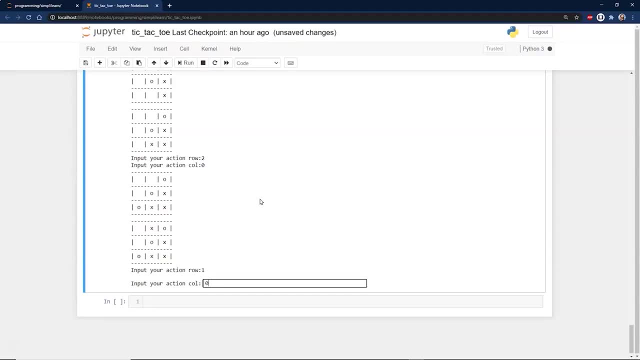 There we go And column 0. That's where I want it, Oh. and it says: OK, your action, There we go, Boom. So you can see here we didn't catch the win on this. It said: tie. 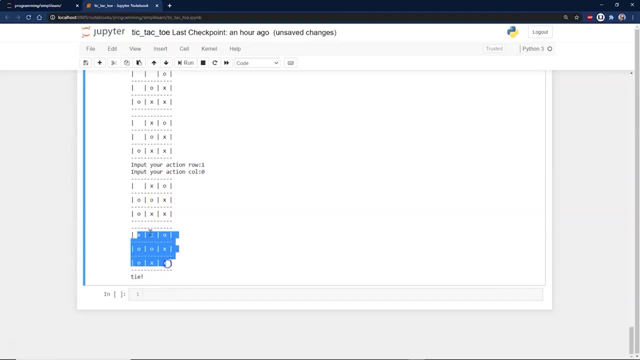 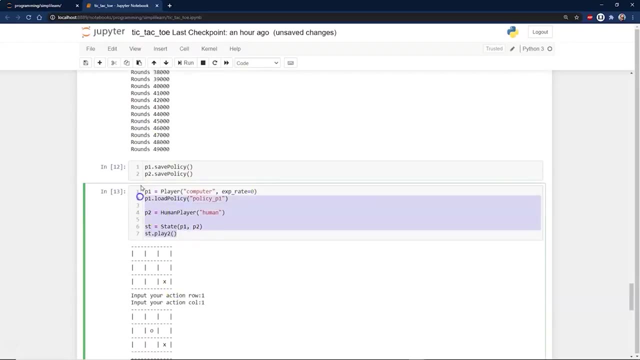 Kind of funny. they didn't catch the win on there. But if we play this a bunch of times you'll find that it's going to win more and more. The more we train it, the more the reinforcement happens. This lengthy training process is really 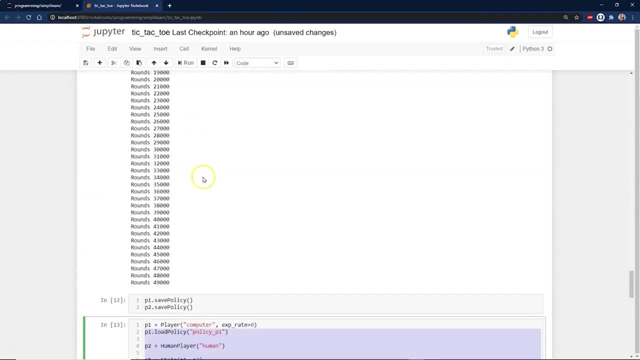 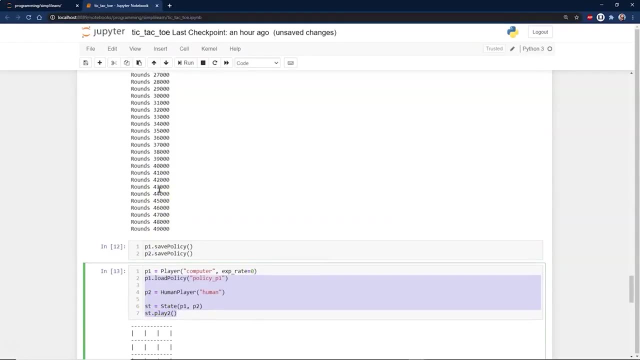 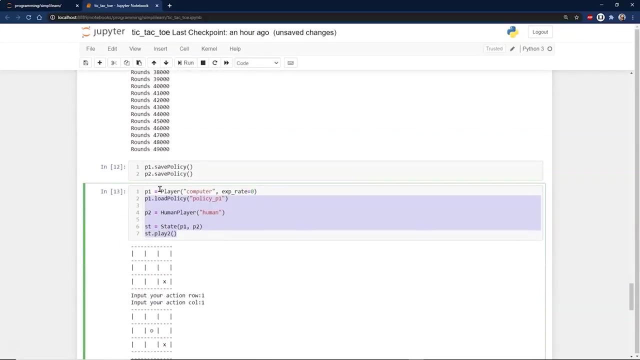 the stopper on reinforcement learning. As this changes, reinforcement learning will be one of the more powerful packages evolving over the next decade or two. In fact, I would even go as far as to say it is the most important machine learning tool and artificial intelligence tool out there. 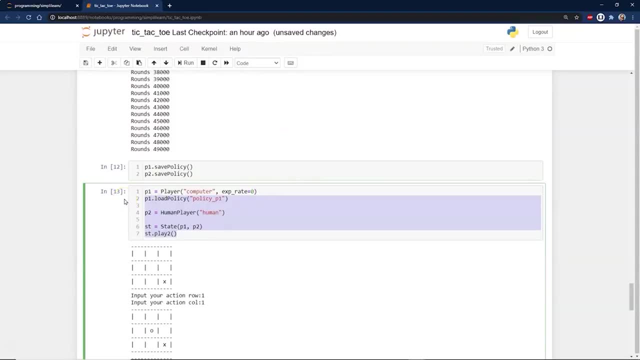 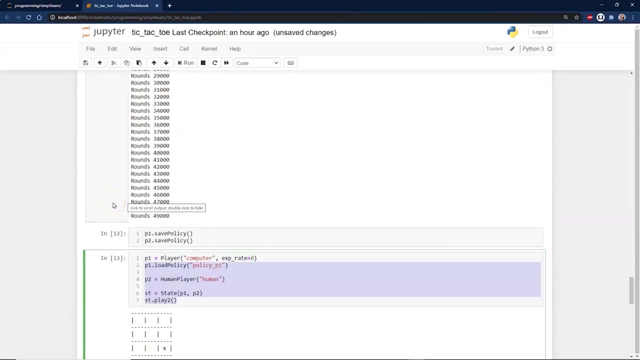 as it learns. not only a simple tic-tac-toe board, but we start learning environments, And the environment would be like a language. If you're translating a language or something from one language to the other, so much of it is lost if you don't know the context it's in. 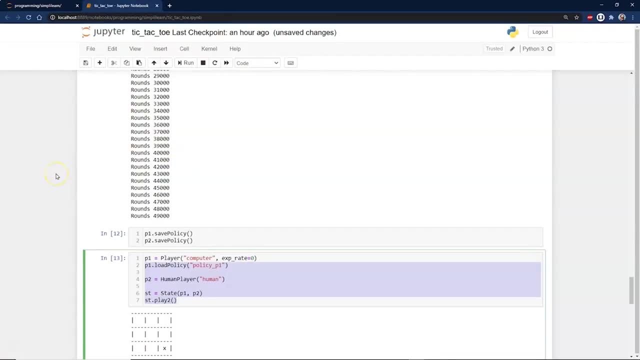 what's the environments it's in, And so being able to attach environment and context and all those things together is going to require reinforcement, learning to do So. again, if you want to get a copy of the tic-tac-toe board, it's kind of fun to play with. 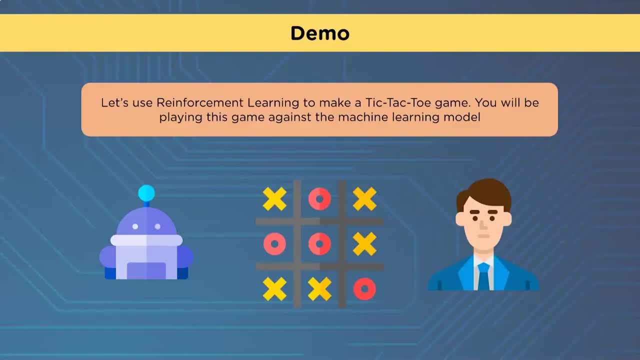 Run it and you can test it out. You can test it for different values. You can switch from P1 computer where we loaded the policy 1, to load the policy 2 and just see how it varies. There's all kinds of things you can do on there. 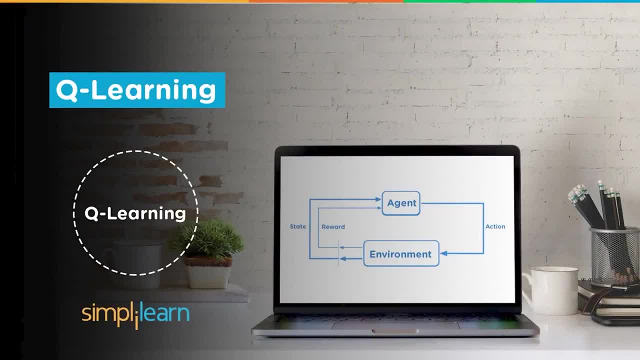 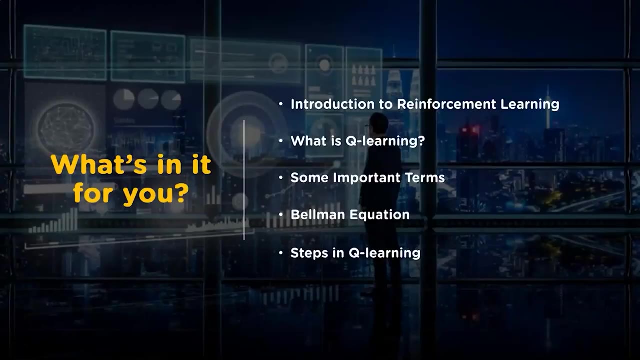 Welcome to Q-Learning. My name is Richard Kirshner with the Simply Learn team, wwwsimplylearncom. Get certified, Get ahead. What's in it for you today? An introduction to reinforcement learning. What is Q-Learning? Some important terms. 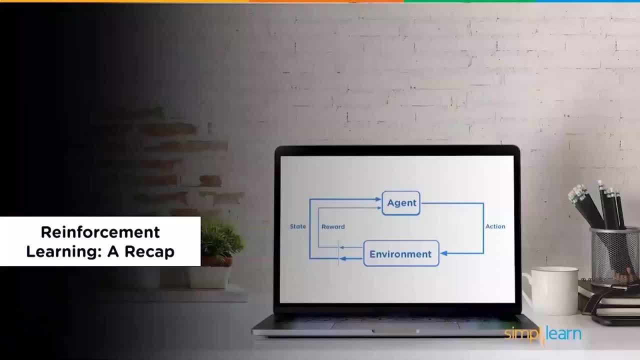 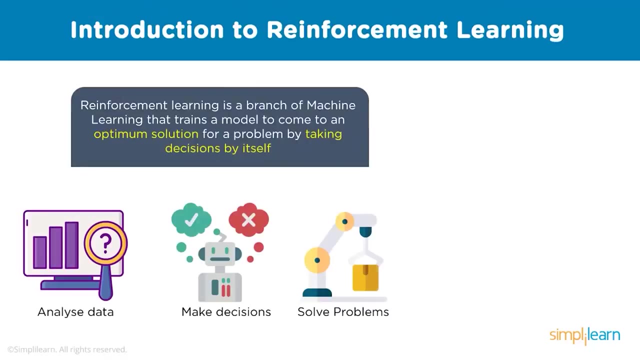 Bellman equation Steps in Q-Learning. A quick recap. So we're going to go back and do a reinforcement learning recap And you'll remember we have our agent, our environment, and our reward and the state, And so reinforcement learning is a branch of machine learning. 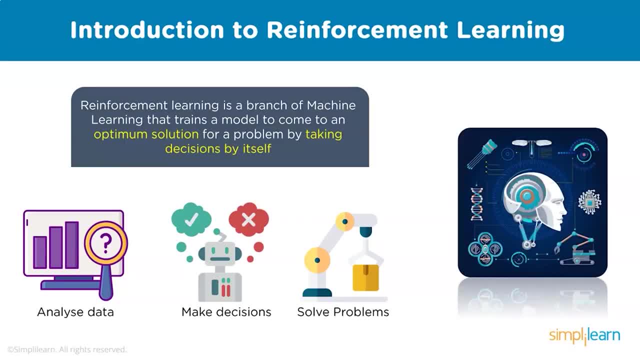 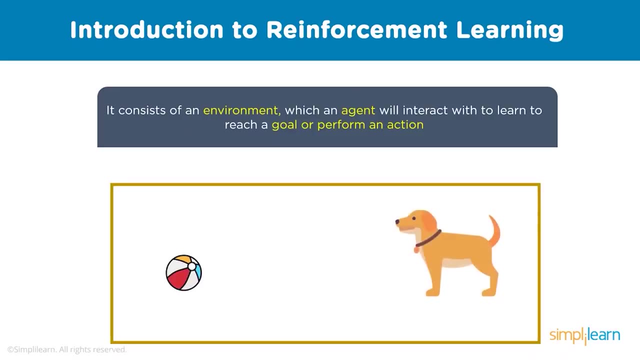 that trains a model to come to an optimum solution for a problem by taking decisions by itself. So we look at it, we analyze the data, make decisions, solve problems. It consists of an environment which an agent will interact with to learn to reach a goal or perform an action. 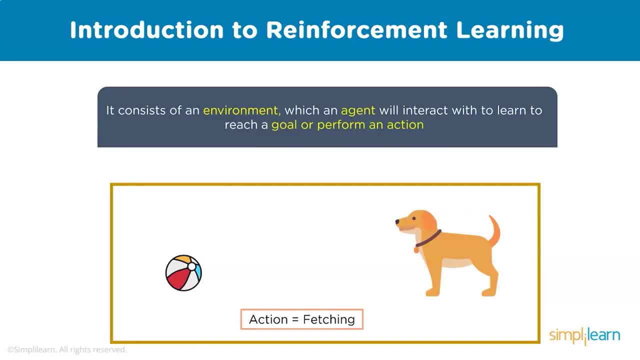 And you see, here we have the dog, and the action equals fetching. And the first thing you're going to notice here- and I'll talk a little bit more about this- is that our action is kind of a singularity. The action isn't a regression type model. 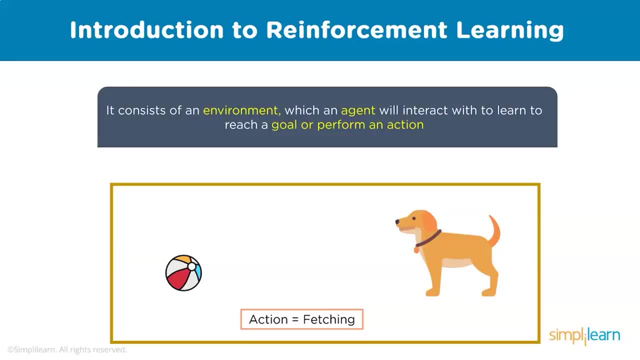 where we're looking at float numbers or we're trying to predict something or doing a reinforcement learning, where we're trying to guess the value of the stock market, where you have 5.33, $5.33.. This is a little bit different. 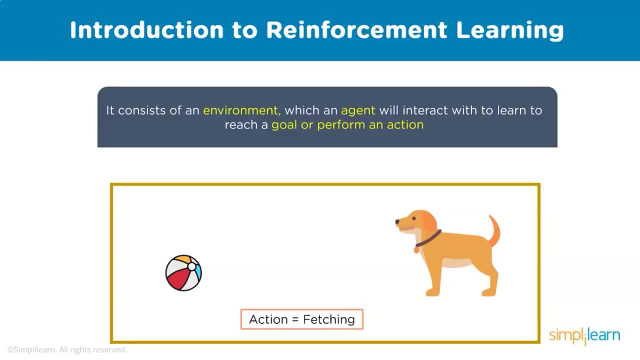 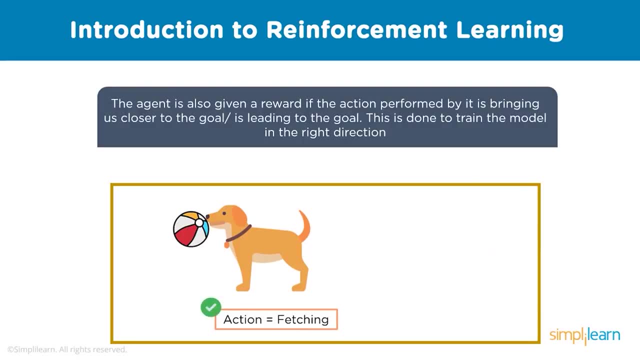 And you'll see why Q-learning is so powerful, but also where it falls short. The agent is also given a reward if the action performed by it is bringing it closer to the goal, is leading to the goal. This is done to train the model in the right direction. 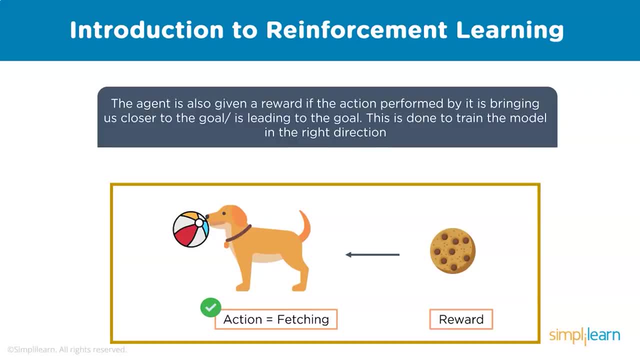 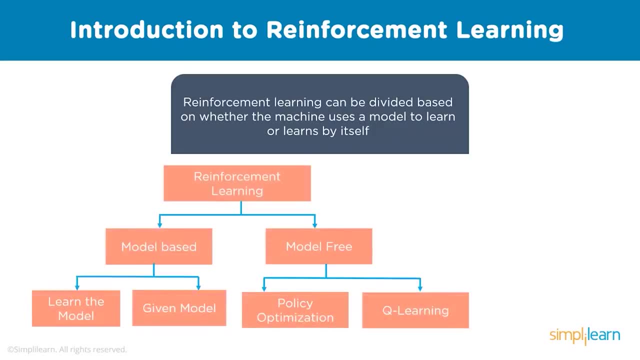 You have a reward of, hopefully, a doggy cookie, and action equals fetching, So it gets a reward. it gets to go fetch the ball. Reinforcement learning can be divided based on whether the machine uses a model to learn or learns by itself. So reinforcement learning, 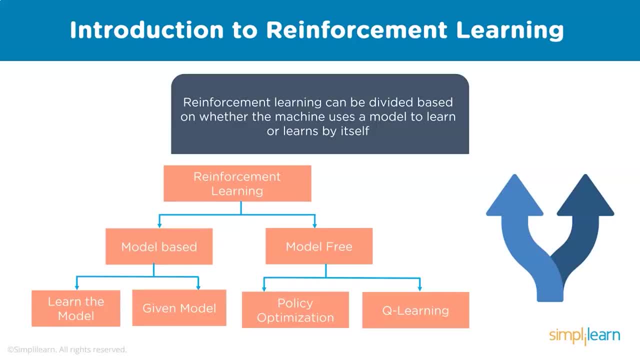 It's model based. learn the model, given model, And you can think of neural networks, I think are the most common right now used for reinforcement learning. There certainly are a lot of other options out there, But you have this black box and you go back and you send the error back up. 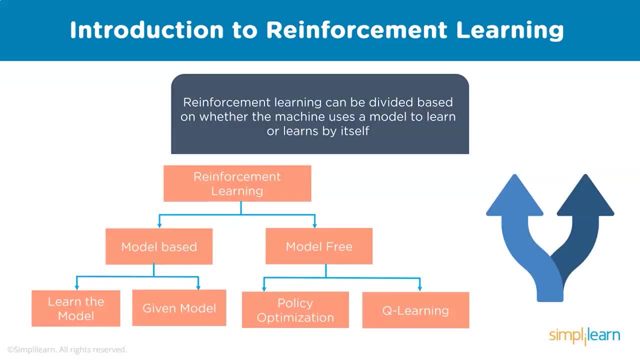 and it trains it based on how much of an error The error could be computed based on, maybe a maximum reward or subtraction or something like that. So the closer you get to the maximum reward, the better, And so we talk about a model free. 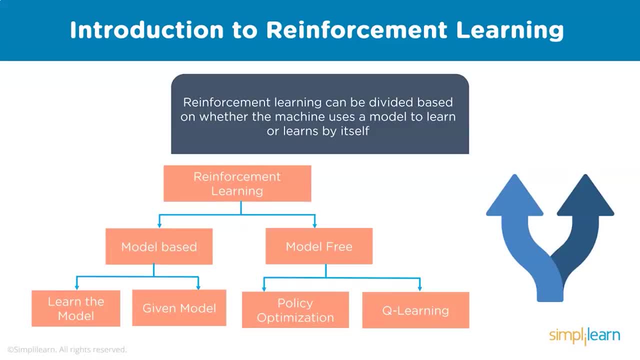 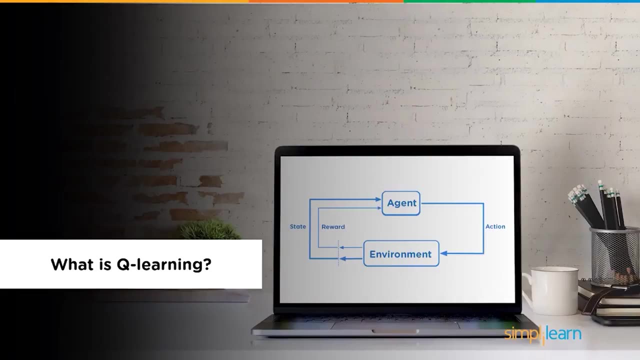 You have your policy optimization and your Q-learning, And this is kind of the cool thing about Q-learning is it's very powerful on certain things, making it very quick and easy to do a reinforcement learning. So what is Q-learning? Q-learning is reinforcement learning policy. 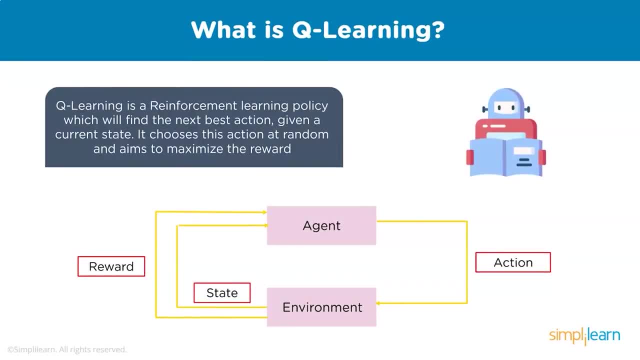 which will fill the next best action given a current state. It chooses this action at random and aims to maximize the reward, And so you can see here's our standard reinforcement learning graph By now. if you're doing any reinforcement learning, you should be familiar with this. 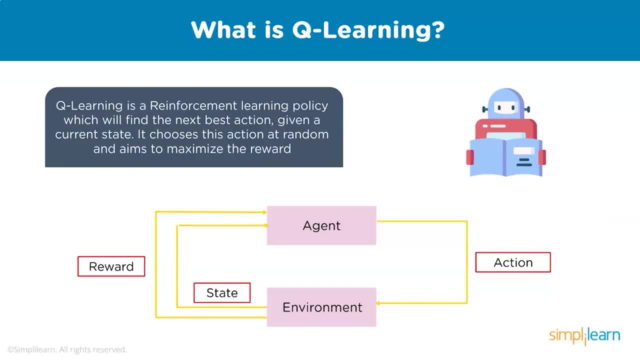 where you have your agent. Your agent takes an action, The action affects the environment And then the environment sends back the reward or the feedback, and the state is the new state, the agent's, in. Where is it at on the chessboard? Where is it at in the video game? 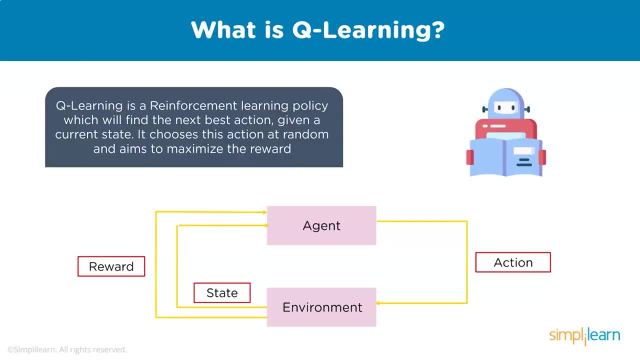 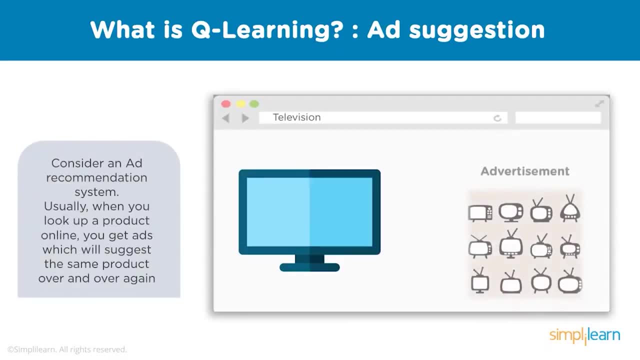 If your robot's out there picking trash up off the side of the road, where is it at on the road? Consider an ad recommendation system. Usually, when you look up a product online, you get ads which will suggest the same product over and over again. 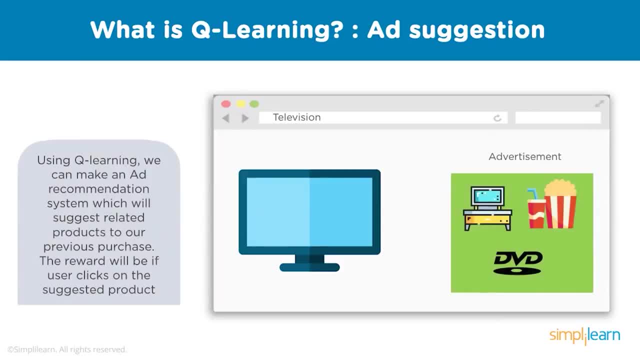 Using Q-learning we can make an ad recommendation system which will suggest related products to our previous purchase. The reward will be if user clicks on the suggested product And again you can see. you might have a lot of products on your web advertisement or your pages. 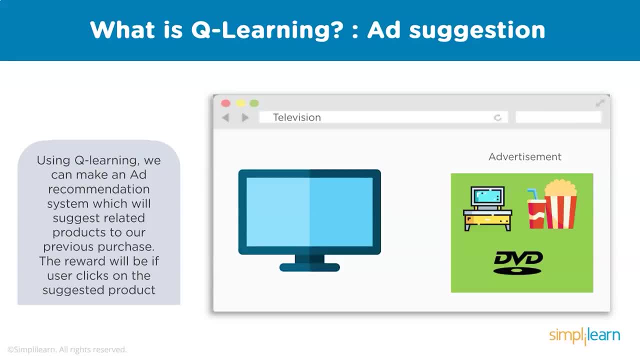 but it's still not a float number, It's still a set number And that's something to be aware of when you're using Q-learning. And you can see here that if you have a hundred people clicking on ads and you click on one of the ads, 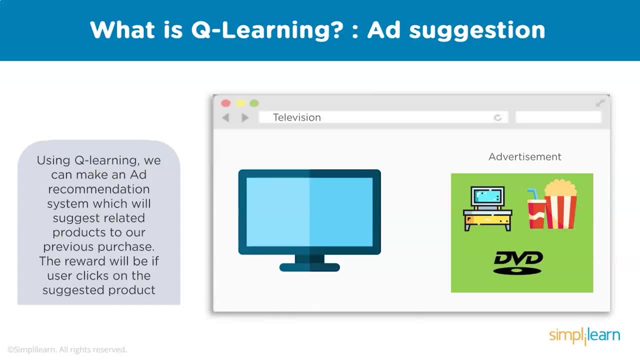 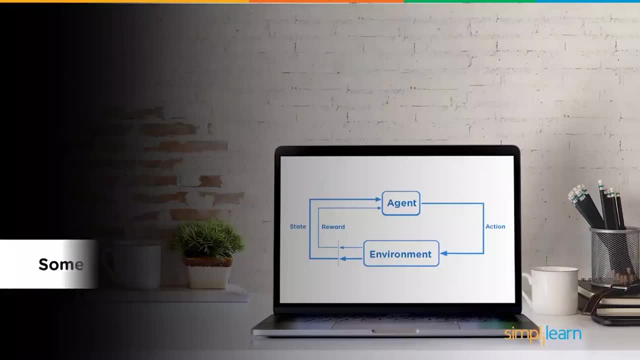 it might go in there and say, okay, this person clicked on this ad. What is the best set of ads, based on clicking on this ad, Or these two ads afterwards, based on where they are browsing? So let's go ahead and take a look at some important terms. 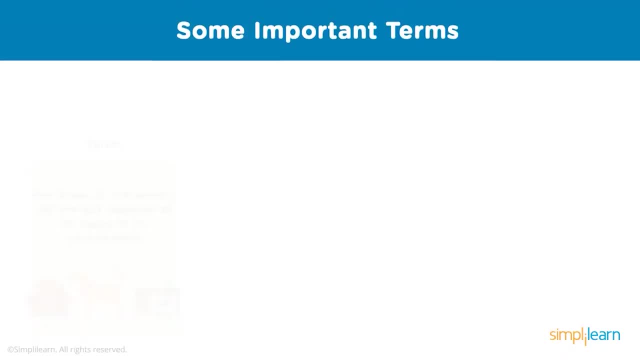 when we talk about Q-learning, We have states. The state S represents the current position of an agent in an environment. The action- The action A- is the step taken by the agent when it is a particular state. Rewards For every action the agent will get. 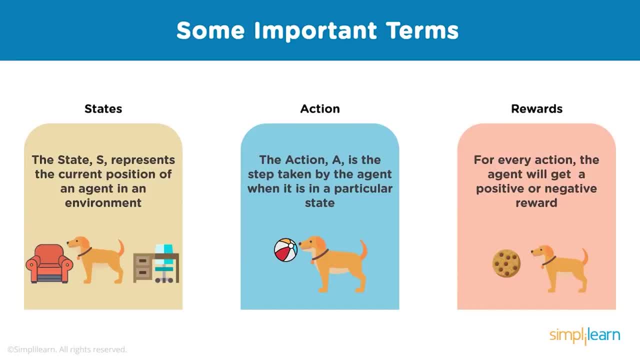 a positive or negative reward. And again, when we talk about states, we're usually not. when you're using a Q-table, you're not usually talking about float variables. You're talking about true-false And we'll take a closer look at that. 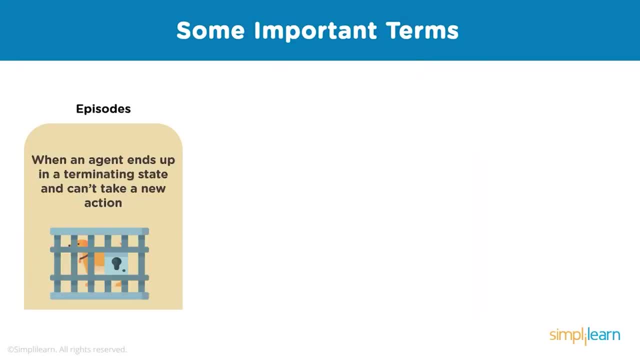 in a second And episodes When an agent ends up in a terminating state and can't take a new action. This might be if you're playing a video game: Your character stepped in and is now dead, or whatever Q-values used to determine. 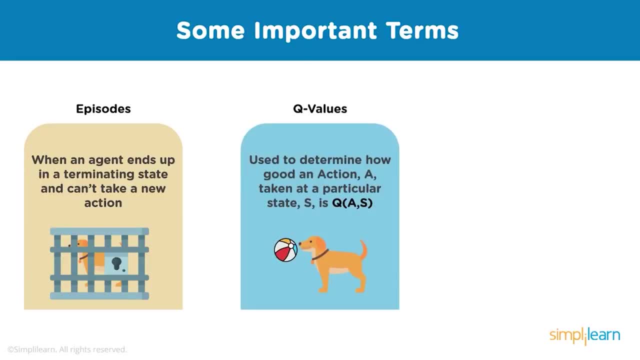 how good an action A taken at a particular state. S is Q A of S And temporal difference. A formula used to find the Q-value by using the value of the current state and action and previous state and action, And very I mean there's Bellman's equation. 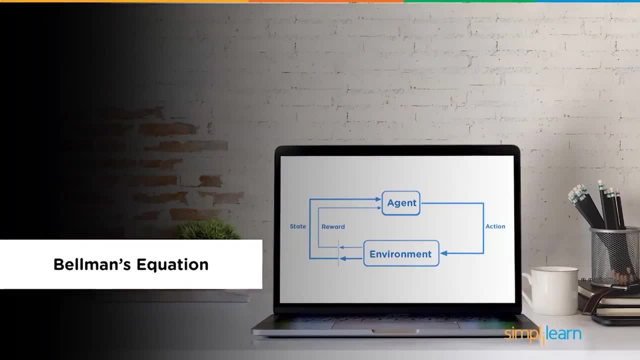 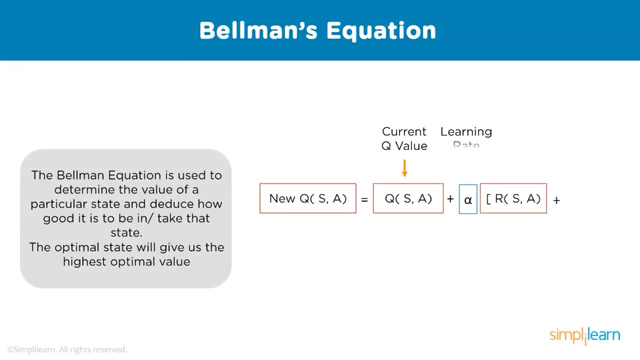 which basically is the equation that kind of covers what we just looked at in all those different terms. The Bellman equation is used to determine the values of a particular state and deduce how good it is to be in. take that state. The optimal state will give us. 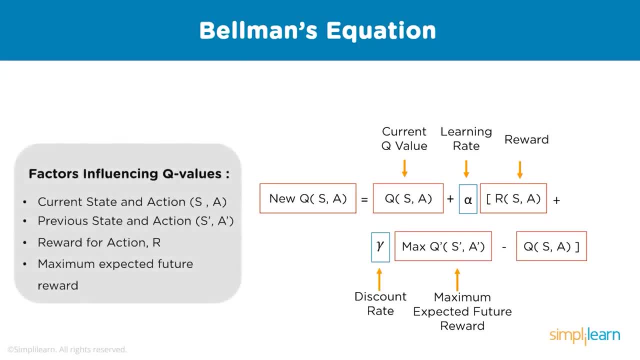 the highest optimal value Factor influencing Q-values, the current state and action. That's your S A. So your current state and your action. Then you have your previous state and action, which is your S, I guess, prime. I'm not sure how they reference that. 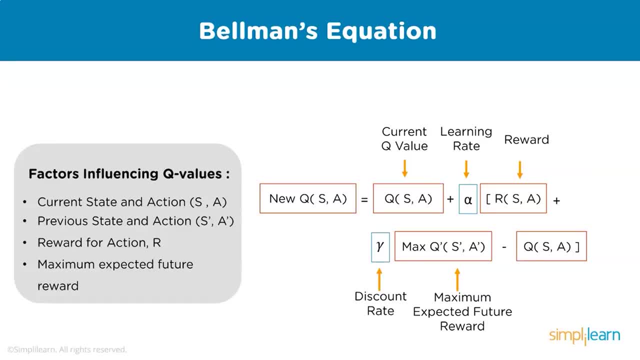 S prime A prime. So this is what happened before. Then you have a reward for action, So you have your R reward And you have your maximum expected future reward And you can see there's also a learning rate put in there and a discount rate. 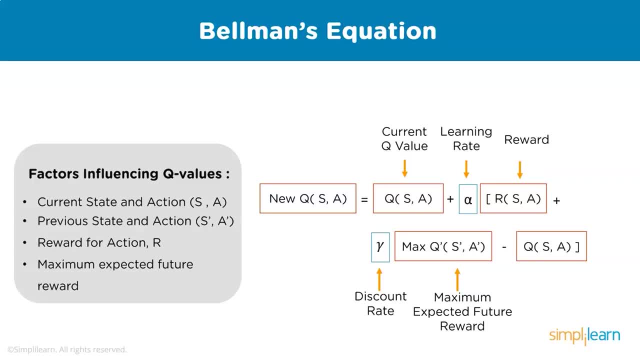 So when we're looking at these, just like any other model, we don't want to have an absolute final value on here. We don't want it to. if you do absolute values instead of taking smaller steps, you don't really have that approach to the solution. 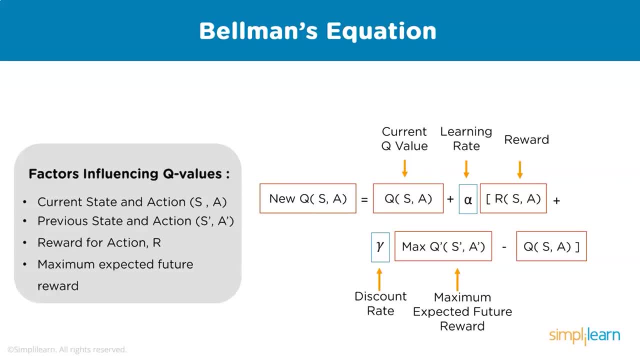 You just have a jump and then pretty soon, if you jump one solution out, that's what's going to be the new solution, Whichever one jumps up really high first, Kind of ruining the whole idea of doing a random selection. And I'll go into the random selection. 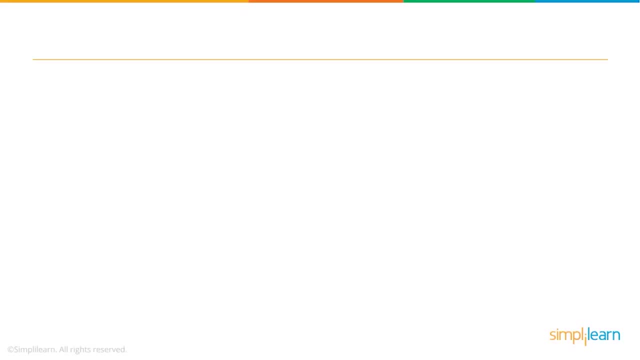 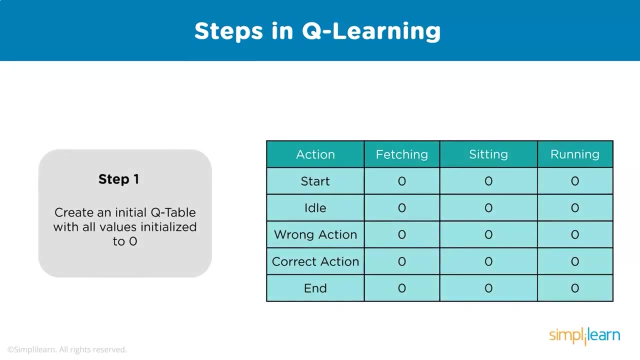 in just a second. Steps in Q learning. Step one: Create an initial Q table with all values initialized to zero. Again, we're looking at zero one. So here's our action: We start. We're in idle, We took a wrong action. 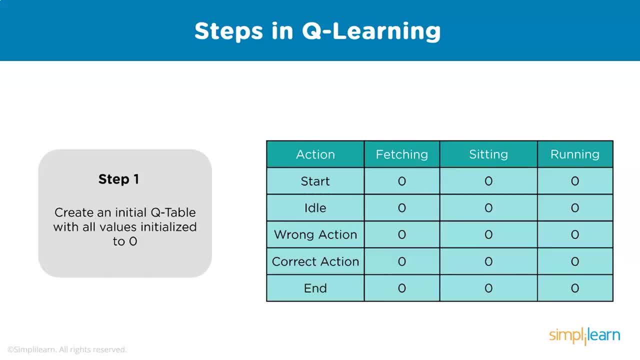 We took a correct action, An end. And then we have our actions: Fetching, sitting and running. Of course, we're just using the dog example And choose an action and perform it, Update values in the table And, of course, when we're choosing an action, 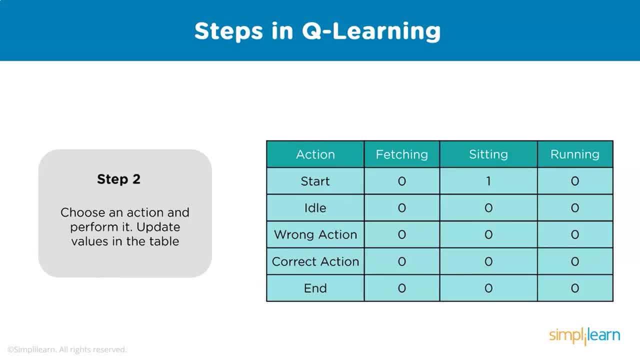 we're going to kind of do something random and just randomly pick one. So you start out and you sit And you have. then, depending on that action you took, you can now update the value for sitting after you start. From start to sitting, Get the value of the reward. 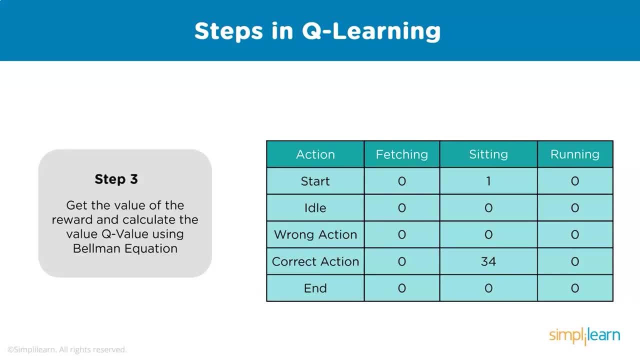 and calculate the value, Q value, using the Bellman equation. And so now we attach a reward to sitting And when we attach all those rewards, we continue the same until the table is filled with or an episode ends, And my image now is going to come back. 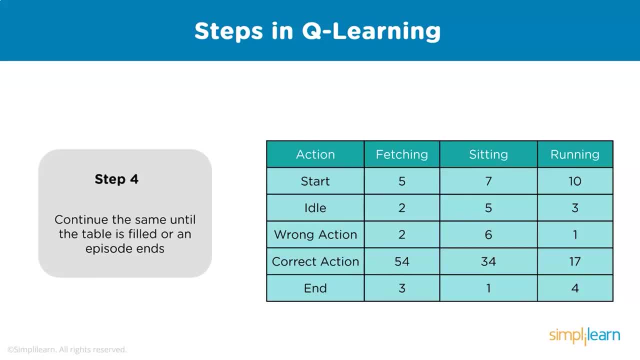 to the random side of this And there's a few different formulas they use for the random set up to pick it. I usually let whatever Q model I'm using do their standard one, because someone's usually gone in and done the math for the optimal spread. 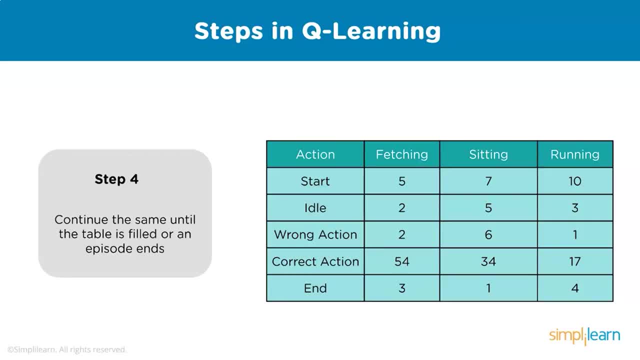 But you can look at this: If I have, running has a reward of 10, sitting has a reward of 7, fetching has a reward of 5, just kind of without doing like a means, using the bell curve for the means value and, like I said, there's some math. 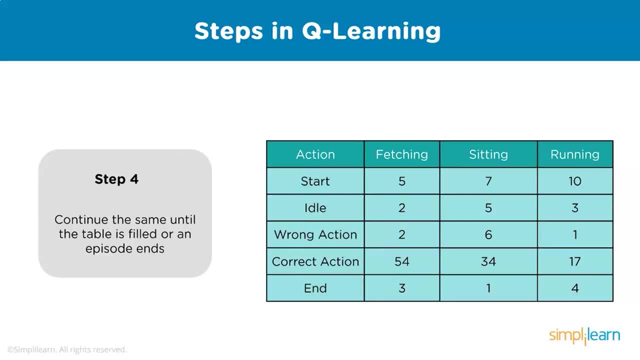 you can put in there to pick, so that running has even a higher chance. But even if you were just going to do an average on this, You could do an average, a random number, by adding them all together. So you get 10 plus 7 plus 5 is 22.. 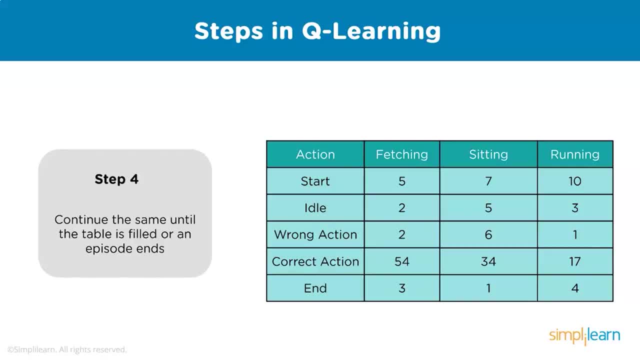 You could do 0 to 22 or 0 to 21, but 1 to 22.. 1 to 5 would be fetching, and so forth. You know the last 10.. So you can just look at this as what percentage are you going to go for? 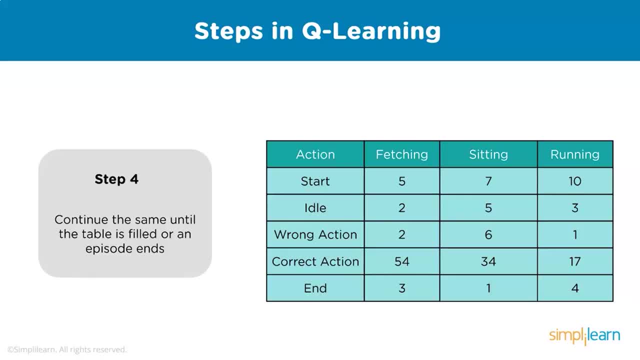 that particular option And then that gets your random set up in there, And then, as you slowly increment these up, you see that if you're idle where's 1, here we go sitting at the end. if you're at the end of wherever you're at, 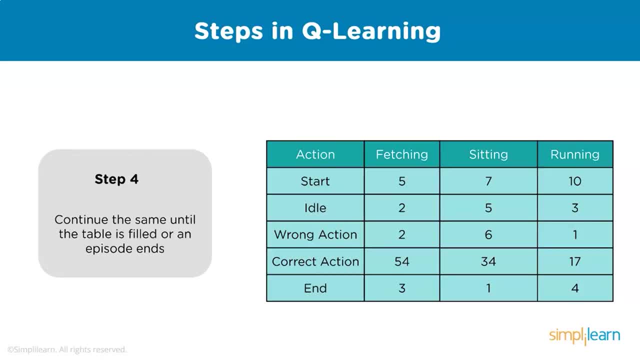 sitting gets a reward of 1.. Where's a good one on here? Oh, wrong action. Running for a wrong action gets almost no reward. So that becomes very, very less likely to happen, but it still might happen. It still might have a percentage of coming up. 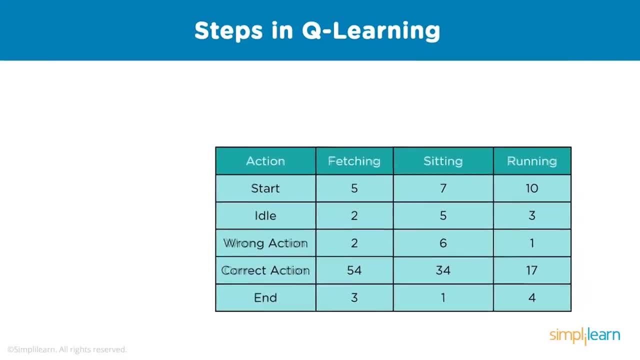 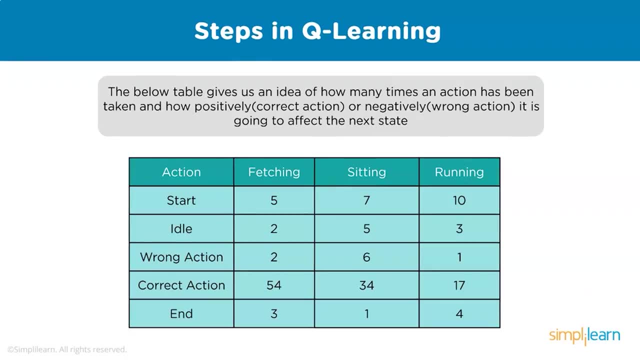 And that's where the random programming and Q-learning comes in. The below table gives us an idea of how many times an action has been taken and how positively correct action or negatively wrong action- it is going to affect the next state. So let's go ahead and dive in. 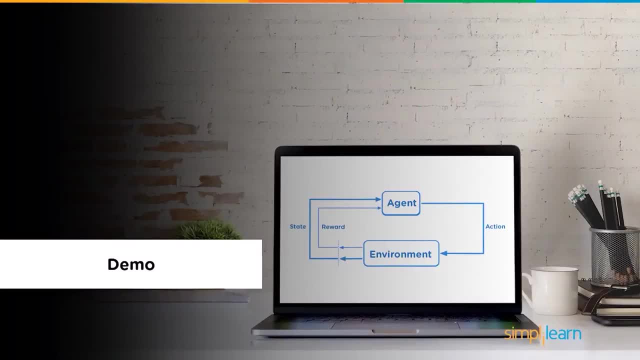 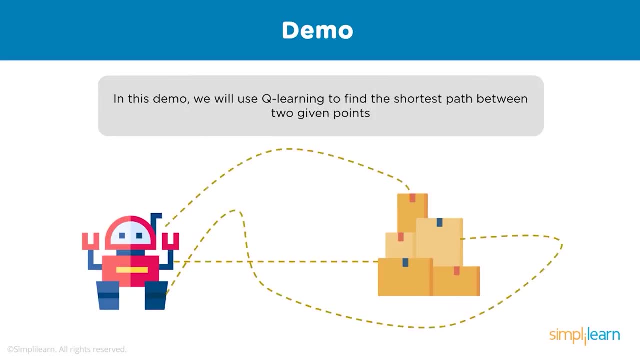 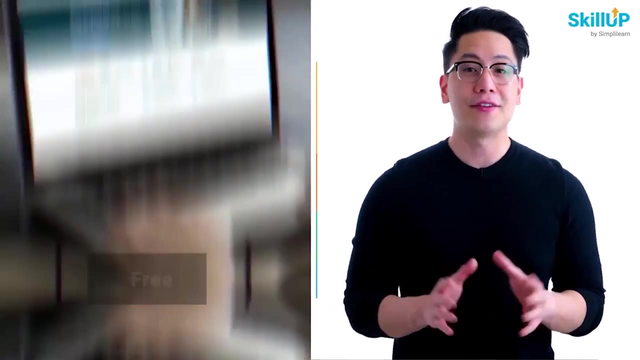 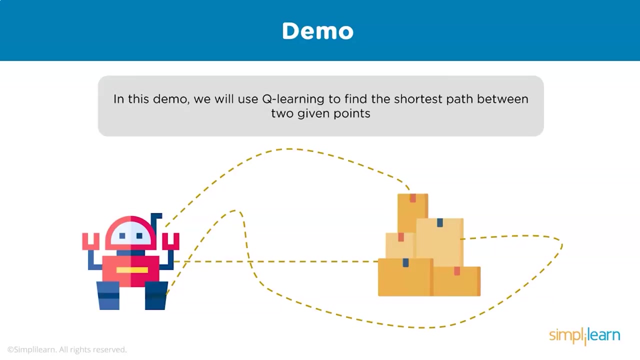 and pull up a little piece of code and see what this looks like in Python. In this demo we'll use Q-learning to find the shortest path between two given points. Find the link in the description to know more, If you've seen my videos before. 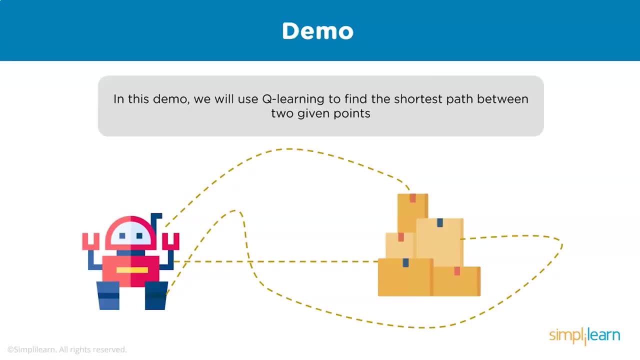 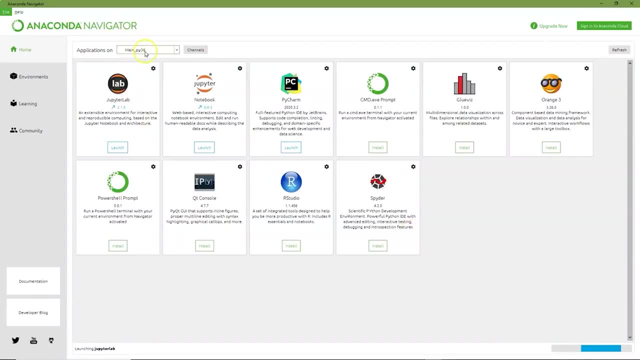 I like to do it in the Anaconda Jupyter Notebook setup, just because it's really easy to see and it's a nice demo. And so here's my Anaconda- This one. I'm actually using Python 3.6 environment that I set up in here. 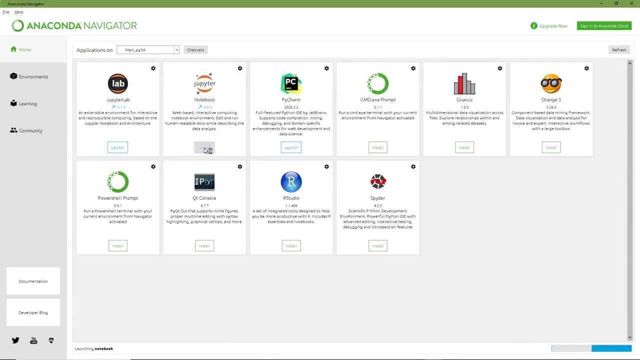 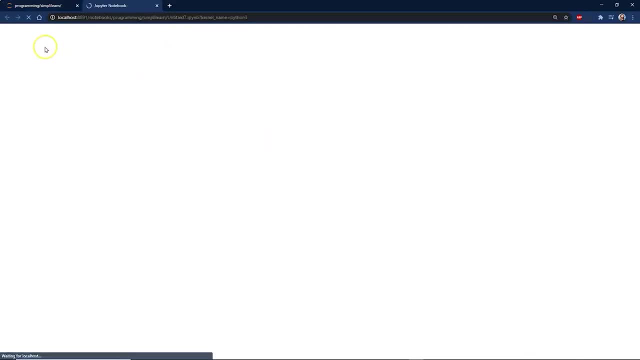 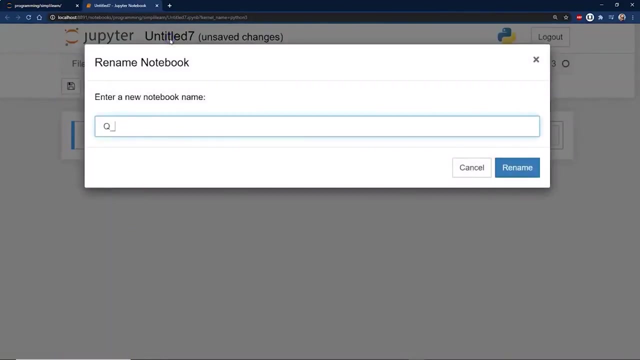 And we'll go ahead and launch the Jupyter Notebook on this. And once we're in our Jupyter Notebook, which has the kernel loaded with Python 3, we'll go ahead and create a new Python 3 folder in here And we'll call this Q-learning. 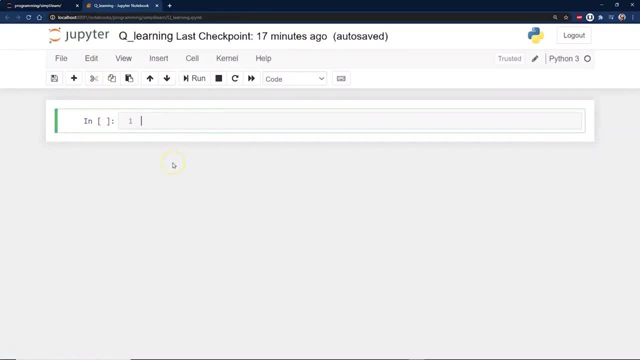 And to start this demo, let's go ahead and import our numpy array. We'll just run that, so it's imported. And, like a lot of these model programs, when you're building them you spend a lot of time putting it all together and then you end up with this really short answer at the end. 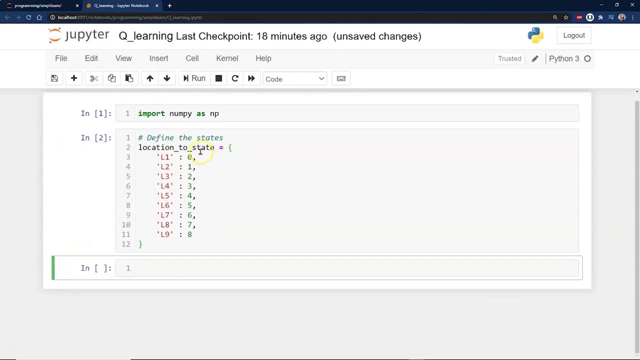 Heh, And we'll take a look at that as we come into it. So we go ahead and start with our location to state. So we have L1, L2. these are our nine locations, one to nine, And then, of course, the state is going to be 0,. 1, 2, 3, 4. 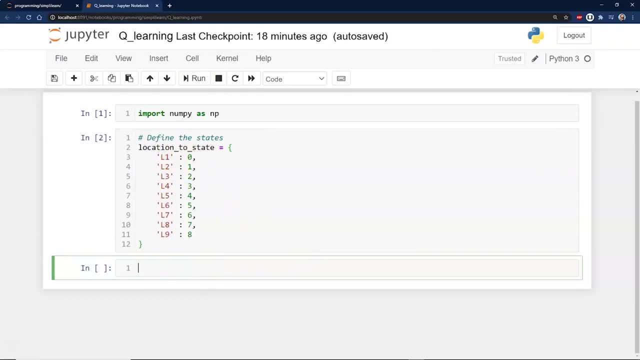 it's just a mapping of our location to an integer on there, And then we have our actions. Our actions are simply moving from one location to another. So I can go to location 0, I can go to location 1,, 2,, 3,, 4,, 5,, 6,, 7, 8.. 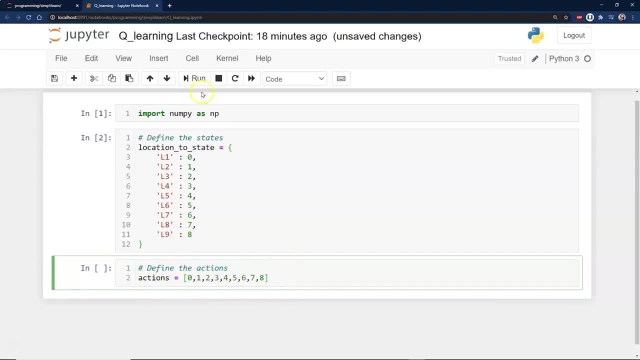 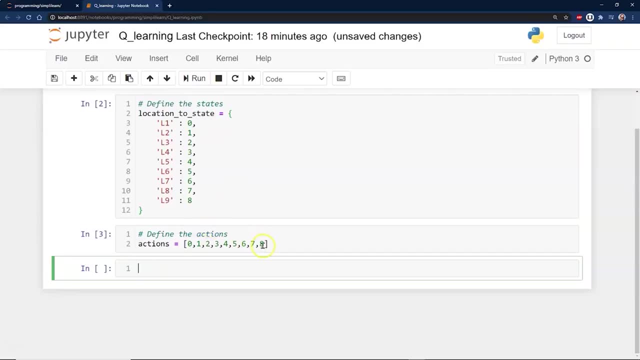 So these are my actions. I can choose. These are the locations of our state And, if you remember, earlier I mentioned that the limitation is that you don't want to put in a continually growing table, because you can actually create a dynamic queue table where you continually add in new values as they arise. 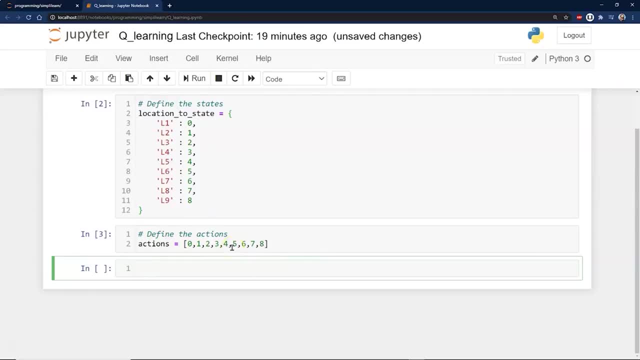 Because if you have float values it just becomes infinite, and then your memory on your computer is gone or it's not going to work. At the same time you might think, well, that kind of really limits the queue learning setup, But there are ways to use it in conjunction with other systems. 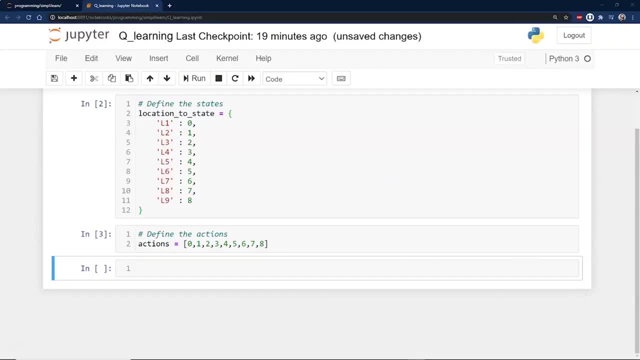 And so you might look at. well, I do, I've been doing some work in stock and one of the questions that comes out is to buy or sell the stock And the stake coming in might be. you might take it and create what we call buckets. 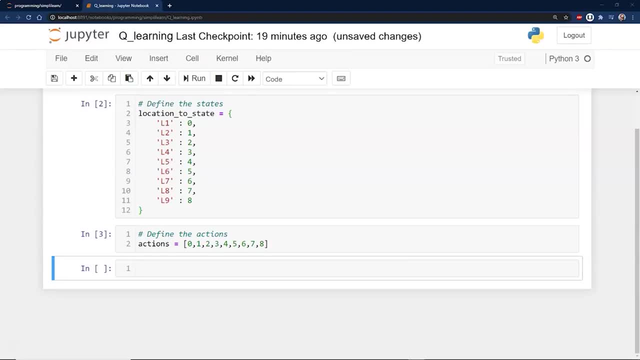 where anything that you predict is going to return more than a certain amount of money- The error for that stock that you've had in the past. you put those in buckets and suddenly, as you start creating these buckets, you realize you do have a limited amount of information coming in. 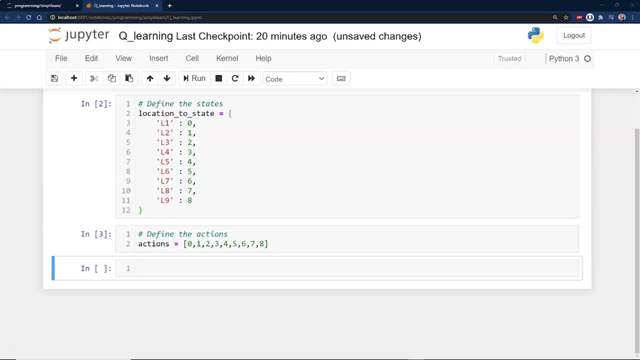 You no longer have a float number. You now have bucket 1,, 2,, 3, and 4.. And then you can take those buckets, put them through a queue learning table and come up with the best action. which stock should I buy? 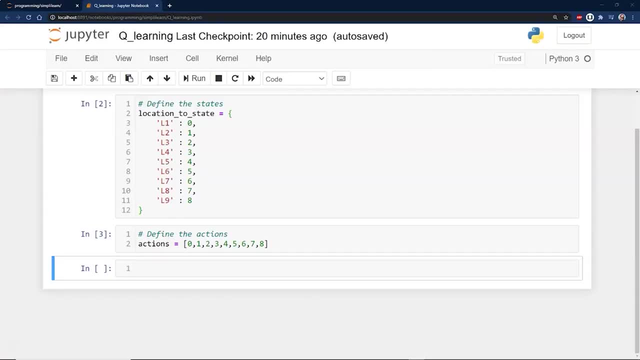 It's like gambling. Stock is pretty much gambling. if you're doing day trading, You're not doing long term investments, And so you can start looking at it like that. A lot of the current feeds say that the best algorithms used for day traders 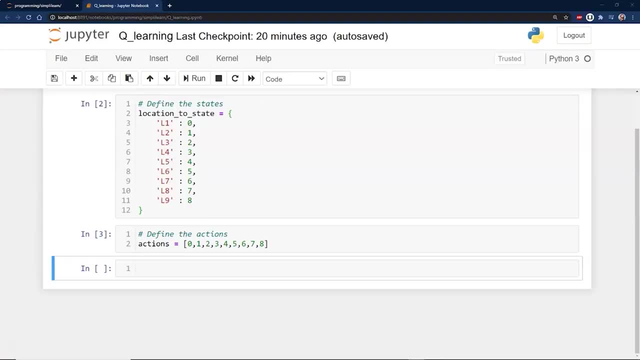 when you're doing it on your own, is really to ask the question: do I want to trade the stock, Yes or no? And now you have it in a queue learning table and now you can take it to that next level and you can see where that can be a really powerful tool. 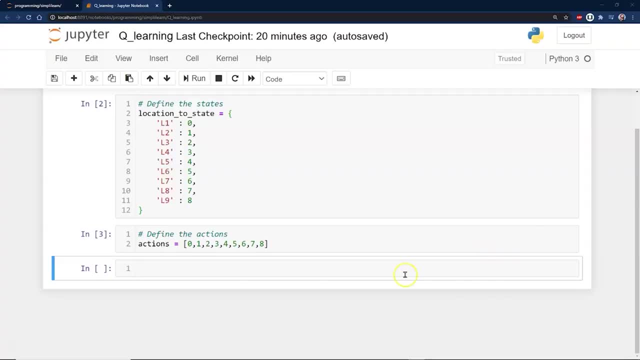 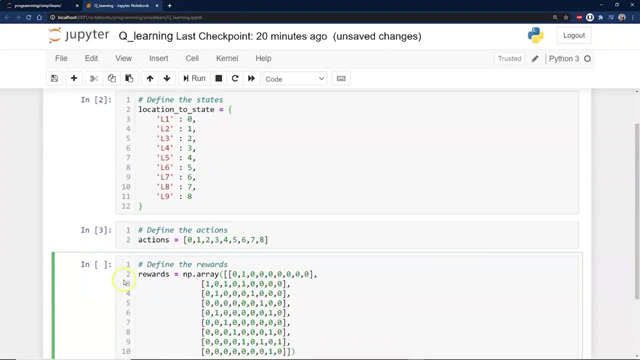 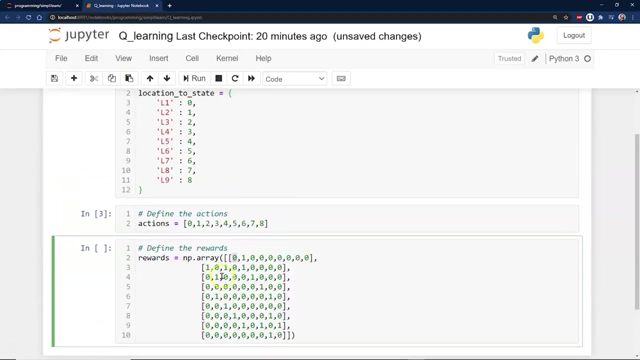 at the end of doing a basic linear regression model or something, What is the best investment? And you start getting the best reward on there, And so if we're going to have rewards, these rewards we just create. It says basically: if you're, this should match our queue table. 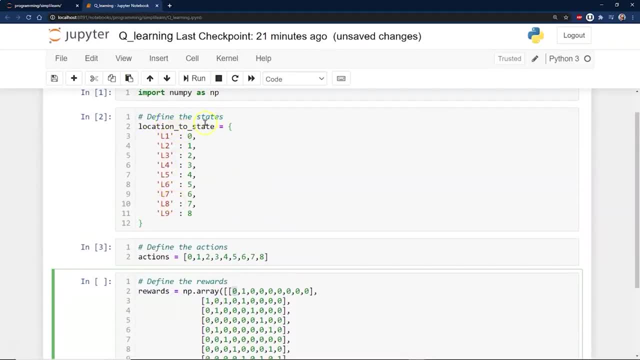 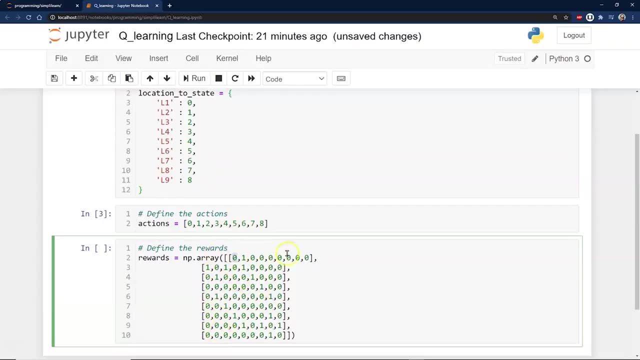 because it's going to be. you have your state and you have your action across the top, If you remember from the dog- And so we have whatever state we're in, going down and then the next action and what the reward is for it. And, of course, if you were actually doing, 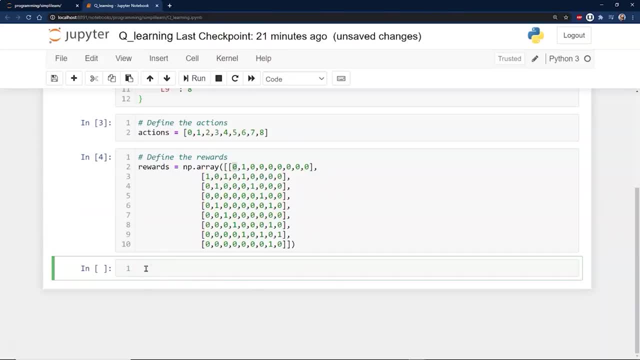 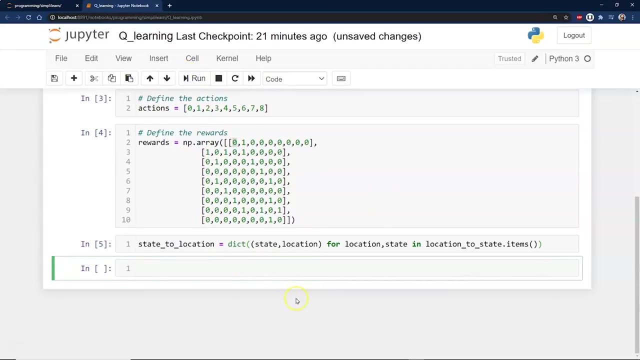 something more connected. your reward would be based on the actual environment it's in, And then we want to go ahead and create a state to location so we can map the indexes. So, just like we defined our rewards, we're going to go ahead and do state to location. 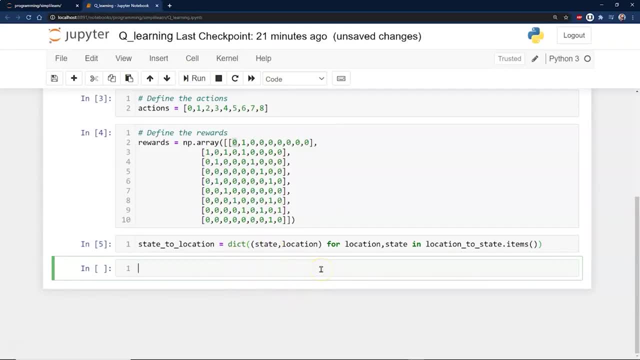 And you can see here, it's a dictionary set up for location, state and location to state with items, And we also need to define what we want for learning rates. You remember we had our two different rates as far as like learning from the past and learning from the current. 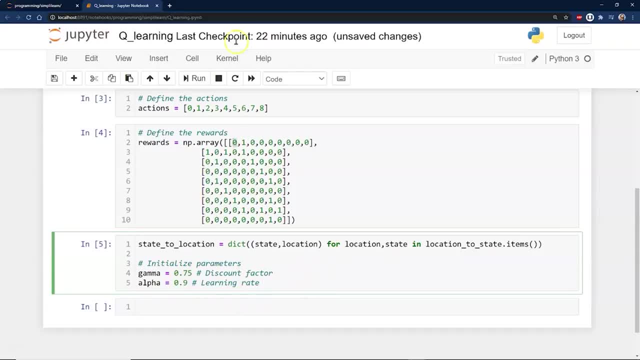 So we'll go ahead and set those to .75 and the alpha set to .9.. And we'll see that when we do the formula And, of course, any of this code, send a note to our Simply Learn team. they'll get you a copy of this code on here. 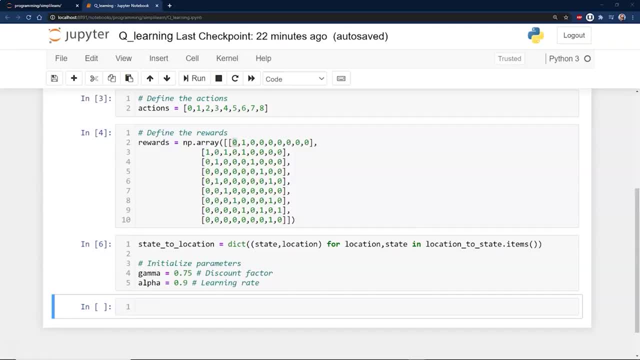 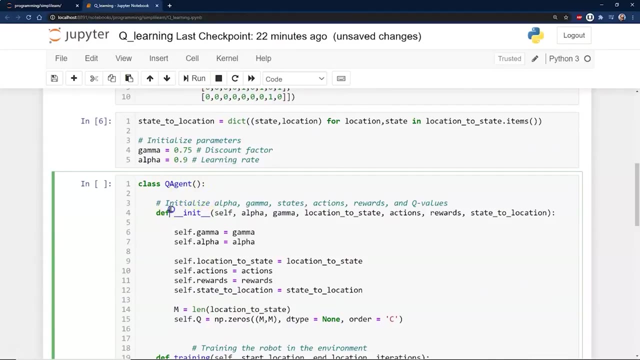 Let's go ahead and pull, There we go, The next two sections, Since we're going to keep it short and sweet. Here we go. So let's go ahead and create our agent. So our agent is going to have our initialization, where we send it all the information. 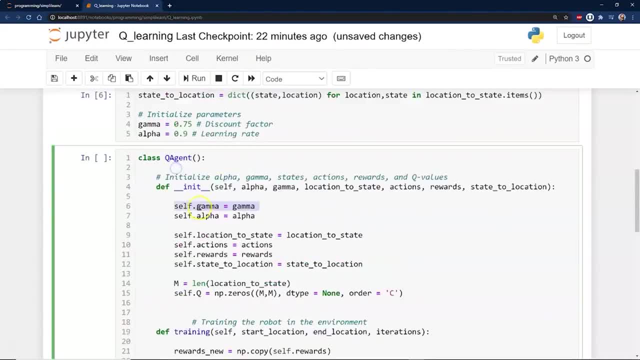 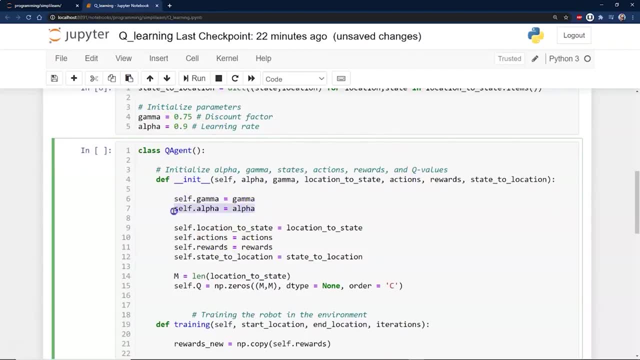 We'll define our self. gamma equals gamma. We could have just set the gamma rate down here instead of submitting it. It's kind of nice to keep them separate, because you can play with these numbers, Our self alpha. Then we have our location state. 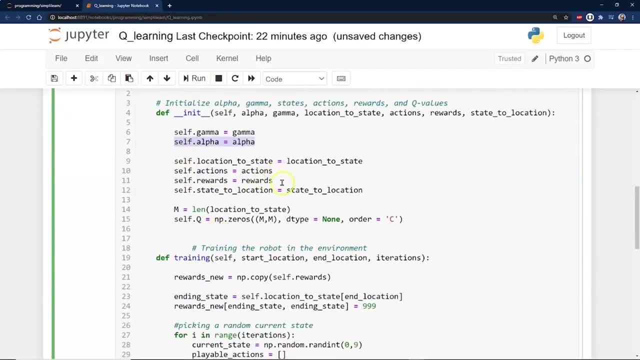 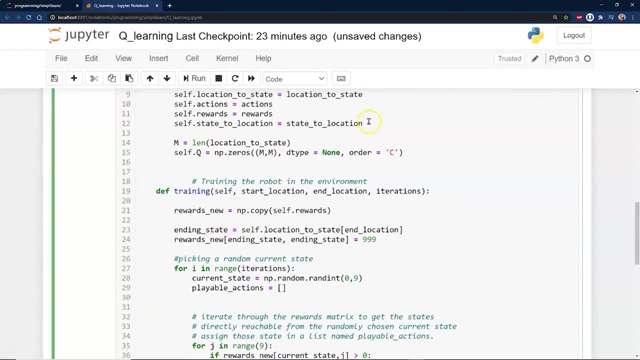 We'll set that in here. We have our choice of actions. We're going to go ahead and just embed the rewards right into the agent, So obviously this would be coming from somewhere else Instead of from self generated And then a self state to location. 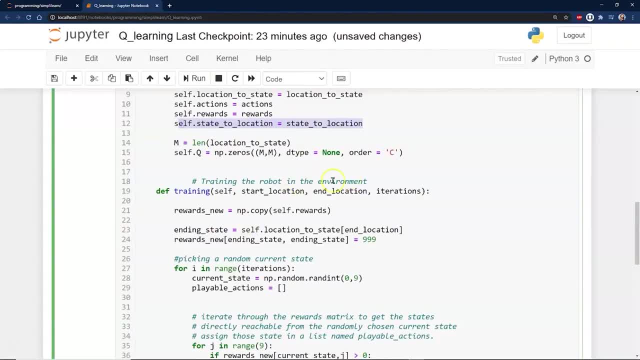 equals our state to location dictionary. And we go ahead and create a Q learning table And I went ahead and just set the Q learning table up to zero, to zero What the setup is, Location to state How many of them are there. 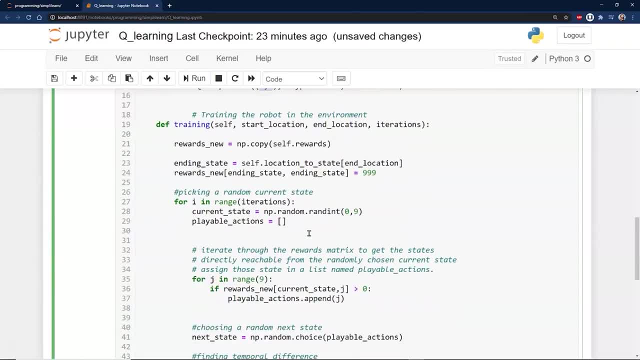 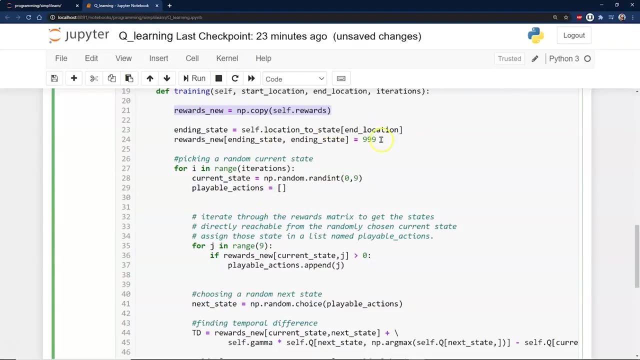 This just creates an array of zero to zero setup on there. And then the big part is the training. We have our rewards: new equals a copy of self dot rewards. Ending state equals the self location state in location. So this is whatever we end up at. 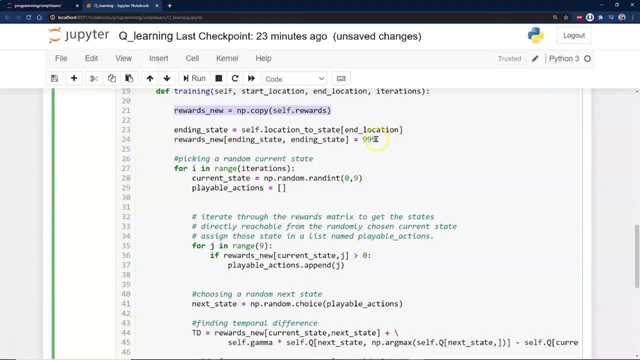 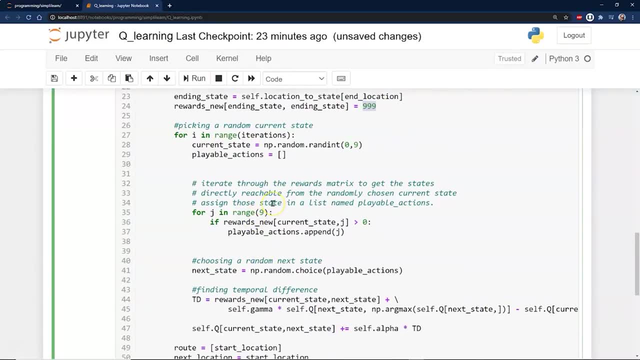 Rewards: new equals ending state. plus ending state equals 999.. Just kind of goes to a dead end And we start going through iterations And we'll go ahead. Let's do this. So this, we're going to come back And we're going to call it on here. 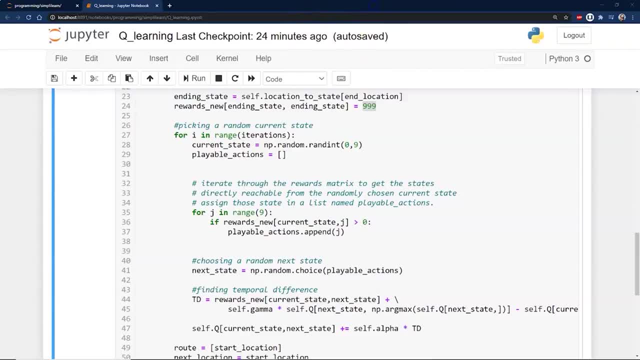 Let me just erase that. Switch it to an arrow. There we go. So what we're doing is we're going to send in here to train it. We're going to say, hey, I want to iterate through this a thousand times And see what happens. 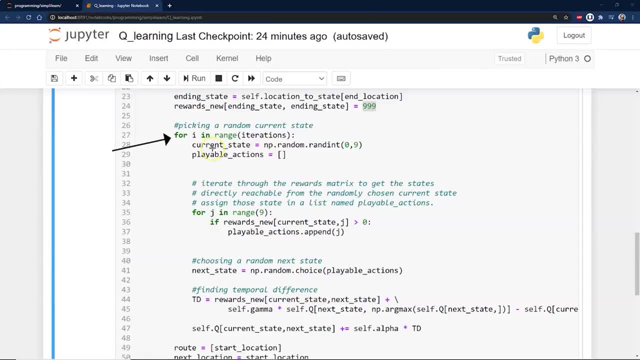 Now this part would actually be: Instead of iterating, you might have your external environment And they're going back and forth And you iterate through outside of here. But just for ease of use, Our agent's going to come in here and iterate through this. 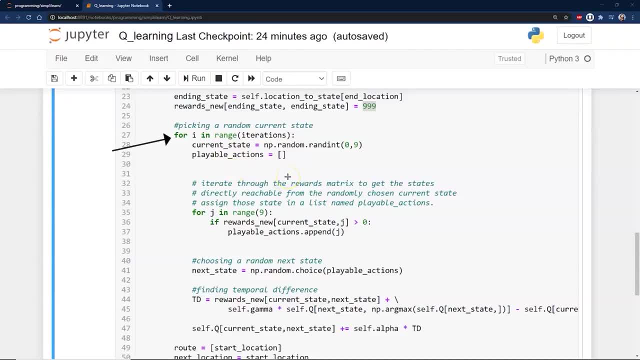 Sometimes I'll put this iteration in here And I'll have it call the environment And say, hey, This is what I did. What's the next state? And the environment does its thing right in here as I iterate through it, And then we want to go ahead and pick a random state to start with. 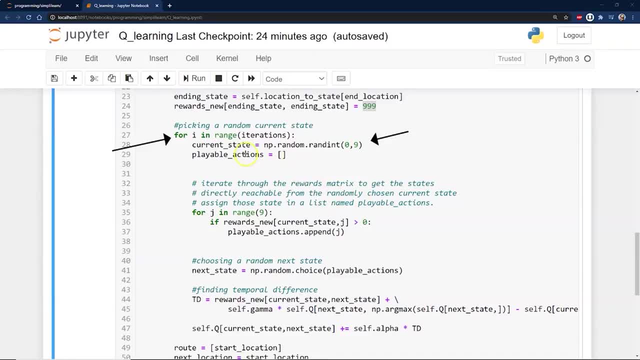 That's what's going on here. You have to start somewhere And then you have your playable actions. We're going to start with just an empty thing for playable actions And we'll fill that up. So that's what choices I have. 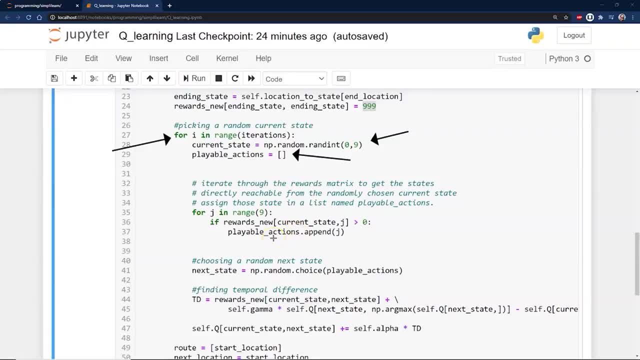 And so we're going to iterate through the rewards matrix to get the states Directly reachable from the randomly chosen current state, Assign those states to a list named playable actions, And so you can see, here we have range 9.. I usually use lengths of whatever I'm looking at. 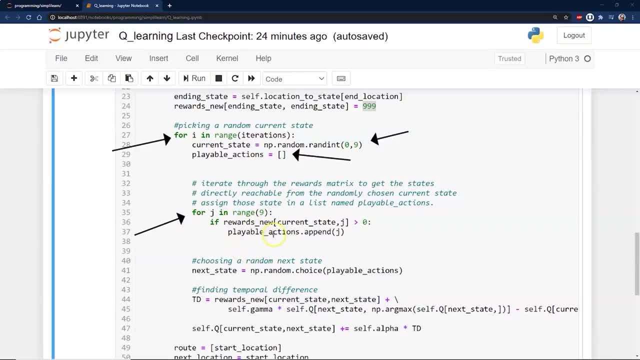 Which is our locations Or states as they are. We have a reward. So we want to look at the current The rewards. The new reward Is our Is in our chart here of rewards, underscore new Current state Plus J. 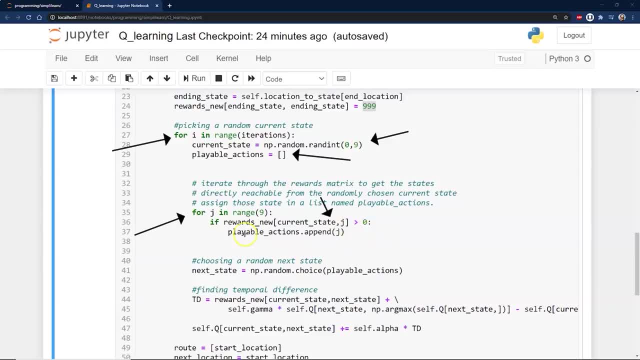 J being what is the next state we want to try, And so we go ahead and do our playable actions And we append J, And so what we're doing is we're randomly trying different things in here To see what's going to generate a better reward. 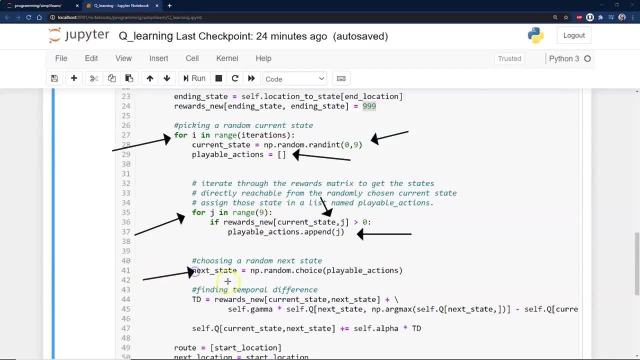 And then, of course, we go ahead and choose our next state. So we have our random choice, playable actions And if you remember, I mentioned- on this- Let me just go ahead and do a free form- When we were talking about the next state. 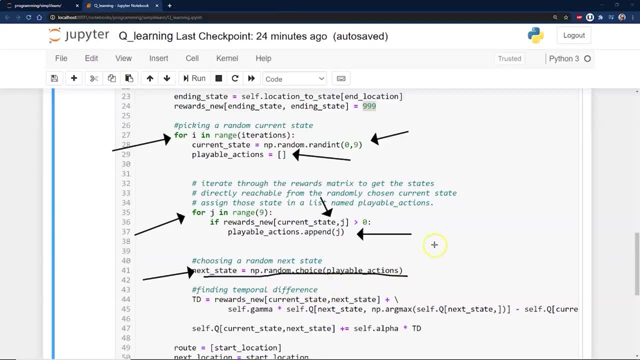 This right here just does a random selection. Instead of a random selection, You might do something where, Whatever the best selection is, Which might be option 3. Here And then, So you can see that it might use a bell curve. 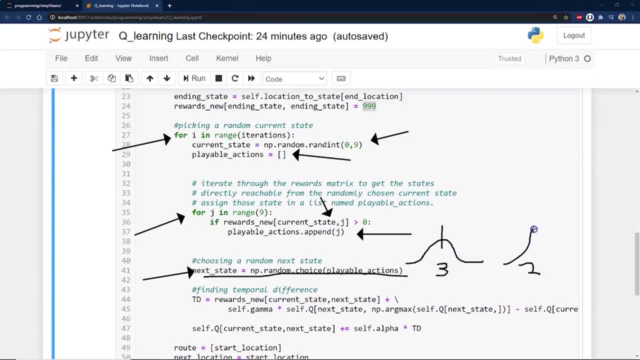 And then option 2 over here Might have a bell curve like this: Oops, And we start looking at these averages And these spreads, Or we can just add them all together And pick the one that kind of goes in all of those. 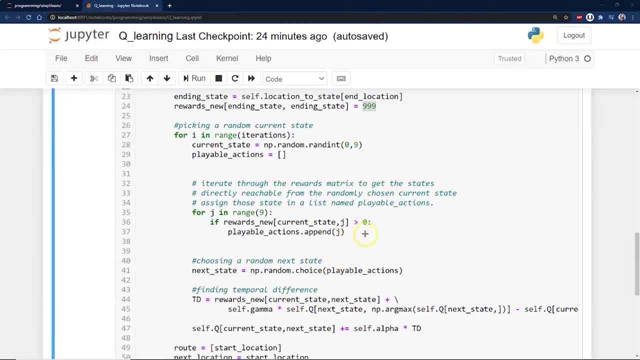 So those are some of the options we have in here. We just go with a random choice. That's usually where you start to play with it, And then we have our reward section down here, And so we want to go ahead and find. 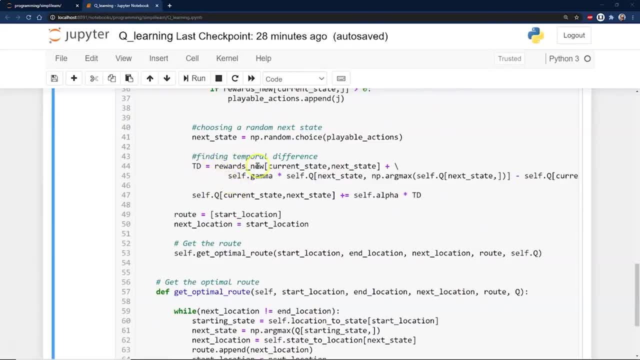 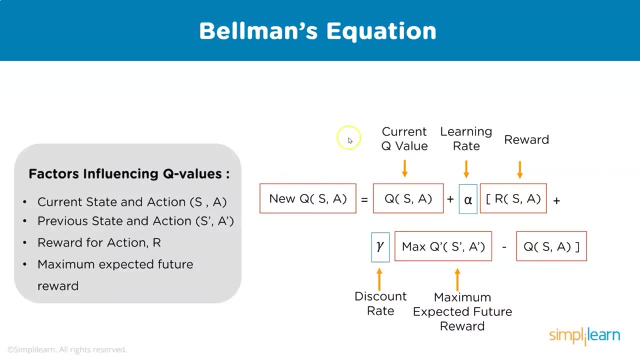 Well, in this case the temporal difference. So you have your rewards new Plus the self gamma, And this is the formula we were looking at. This is Bellman's equation here. So we have our current value, Our learning rate, Our discount rate involved in there. 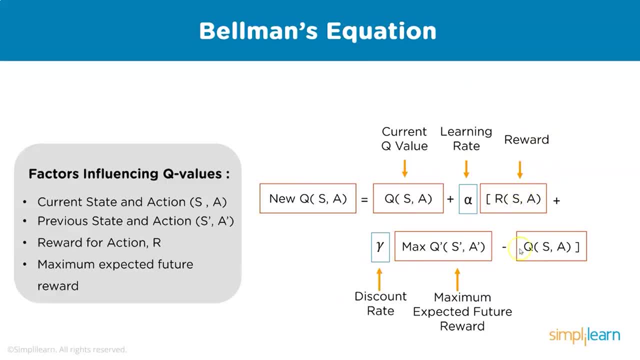 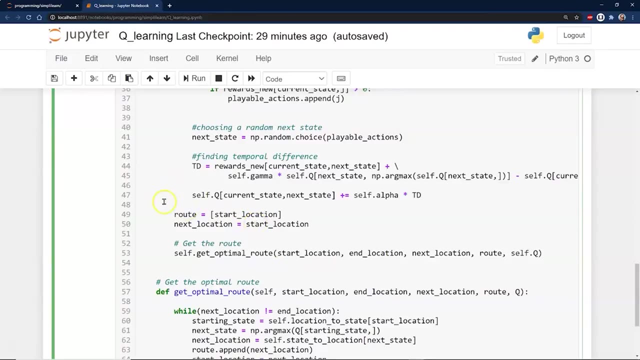 The reward system coming in for that, And we can add it all together. This is, of course, our maximum expected future setup in here. So this is all of our Bellman's equation that we're looking at here, And then we come up in here and we update our queue table. 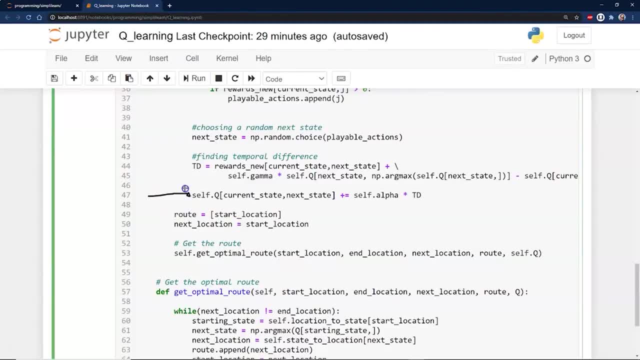 That's all. this is on this one. That's right. here We have self queue- current state, next state- And we add in our alpha- Because we don't want to train all of it at once- In case there's slight differentials coming in there. 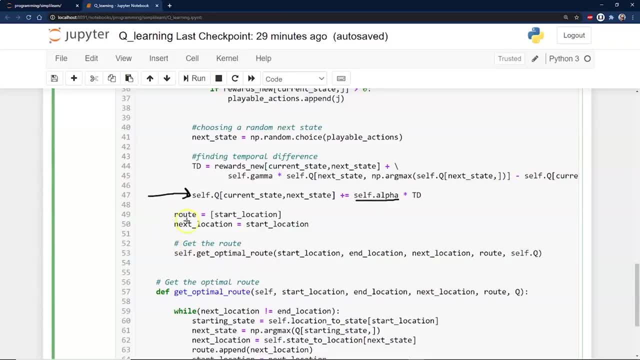 We want to slowly approach the answer. And then we have our route equals the start location And next location equals start location. So we're just incrementing, We took a step forward And then finally, Remember I was telling you how we're going to do all this. 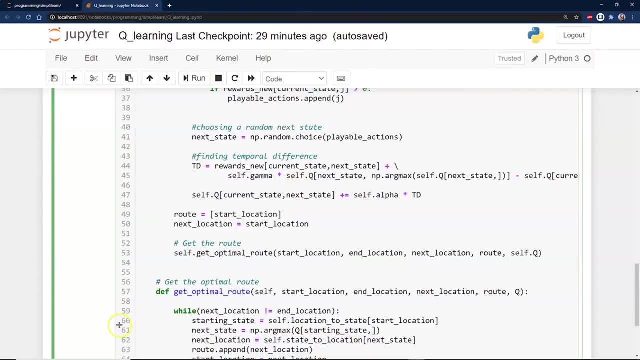 And just have some simple thing at the end Or just generates a simple path. We're going to go ahead and get the optimal route. We want to find the best route in here, And so we've created a definition for the optimal route down here. 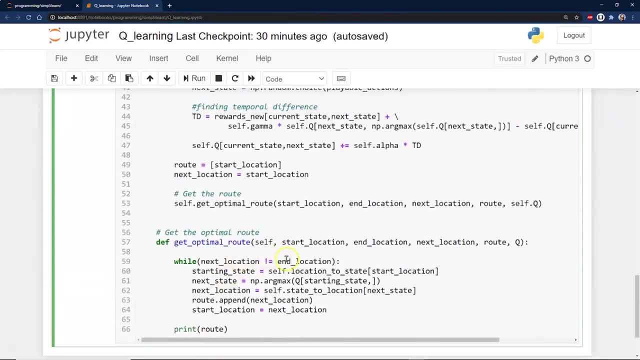 Just scroll down for that And we get the optimal route. We go ahead and put the information in Including the queue table: Self start location, End location, Next location- End queue, And it says: while next location is not equal to end location. 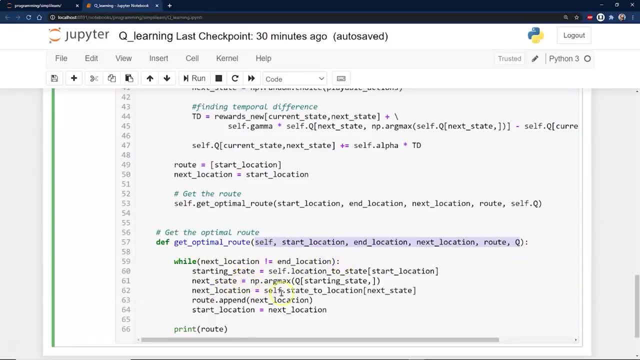 So while we can still go, Our start location equals self location to state start location. So we already have our best value for the start location. The next state looks at the queue table And says, hey, what's the next one with the best value. 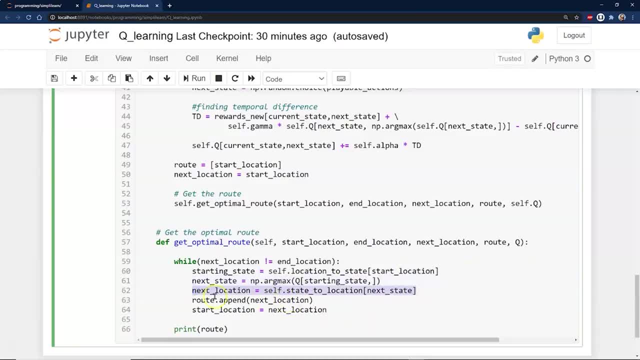 And then the next location. we go ahead and pull that in And we just append it. That's what's going on down here. And then our start location equals the next location And we just go through all the steps And we'll go ahead and run this. 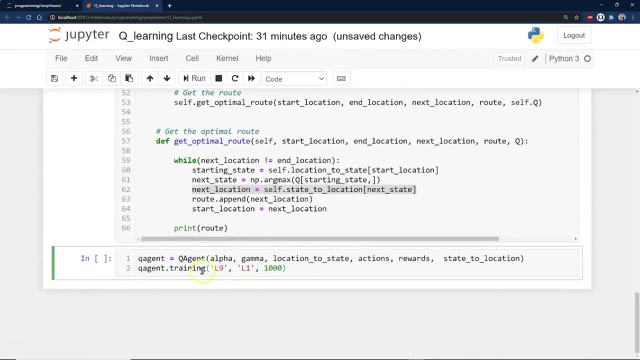 And now that we have our queue table, Our queue agent loaded, We're going to go ahead and take our queue agent, Load them up with our alpha gamma that we set up above, Along with the location step Action rewards State to location. 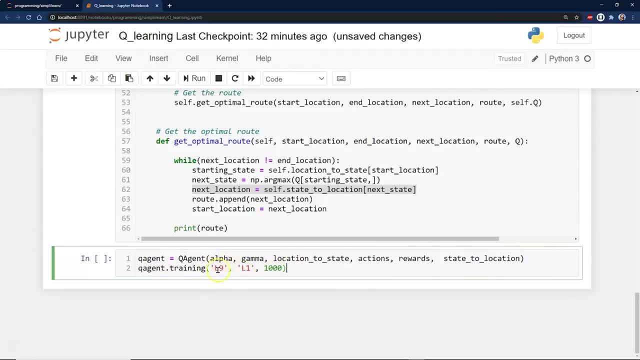 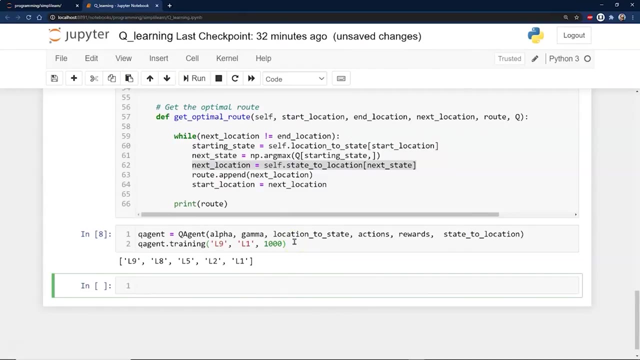 And our goal is to plot a course between L9 and L1.. And we're going to go through a hundred, A thousand iterations on here, And so when I run that It runs pretty quick. Why is this so fast If you've been running neural networks? 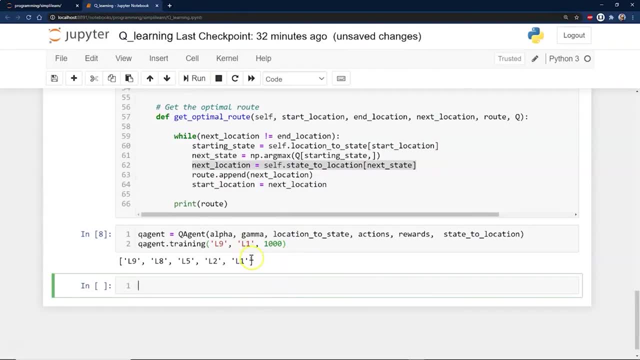 And you've been doing all these other models. You sit here and wait a long time. Well, we're a very small amount of data. These are all integers. These aren't float values. The math is not heavy on the processing end, And this is where queue tables are so powerful. 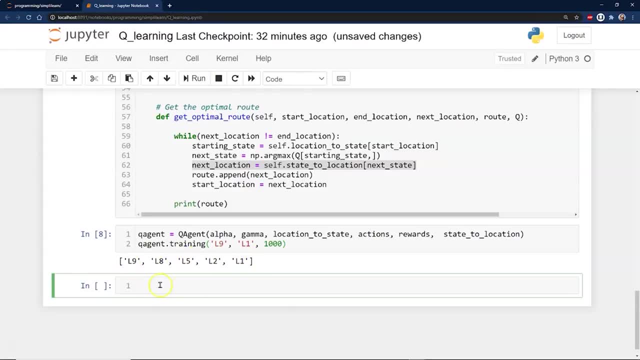 If you have a small amount of information coming in, You very quickly get an answer off of this, Even though we went through it a thousand times To train it And you'll see here we have L9,, 8,, 5,, 2, and 1.. 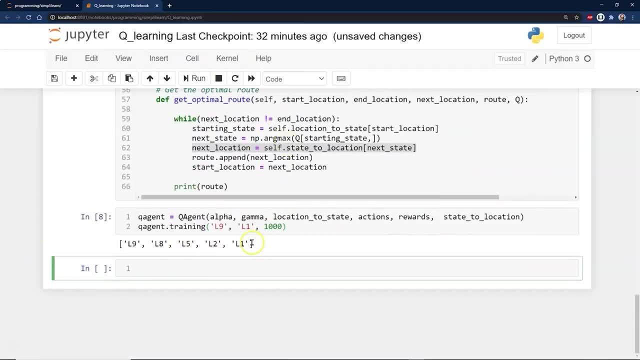 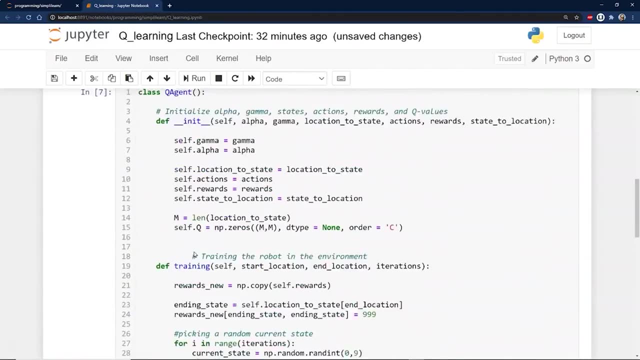 And that's based on our reward table we had set up on there And this is the shortest path Going between these different setups in here And if you remember on our reward table, You can see that if you start here You can go to here. 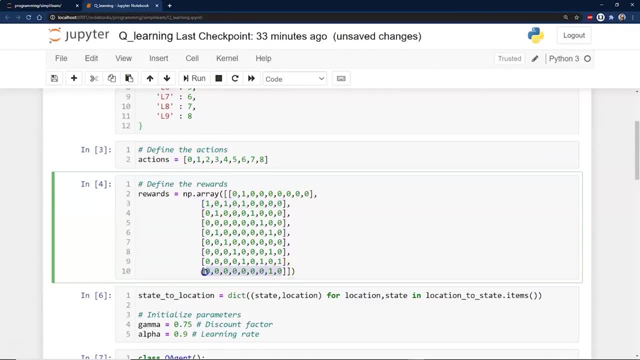 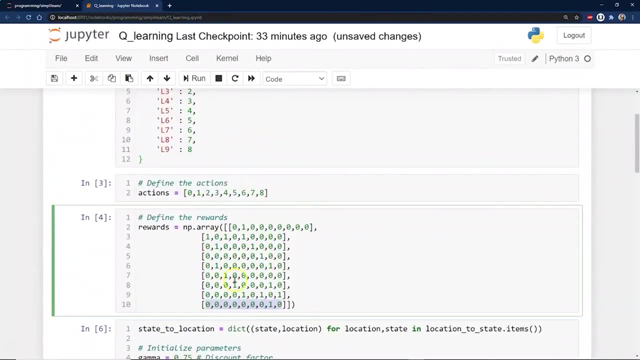 There's places you can't go. That's how this reward table was set up, So I can only go to certain places. So kind of a little maze setup in there And you can play with it. This is a really fun setup to play with. 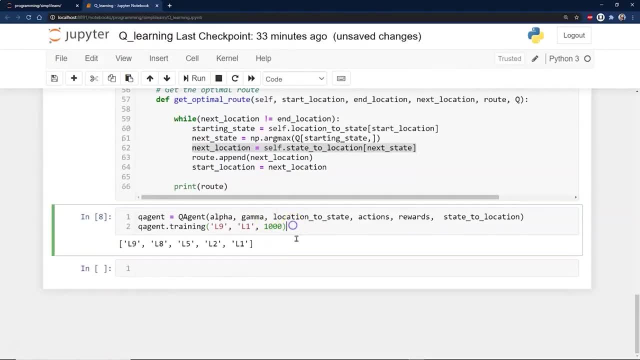 And you can see how you can take this whole code And you can, like I was saying earlier, You can embed it into another setup in model and predictions, Where you put things into buckets And you're trying to guess the best investment. 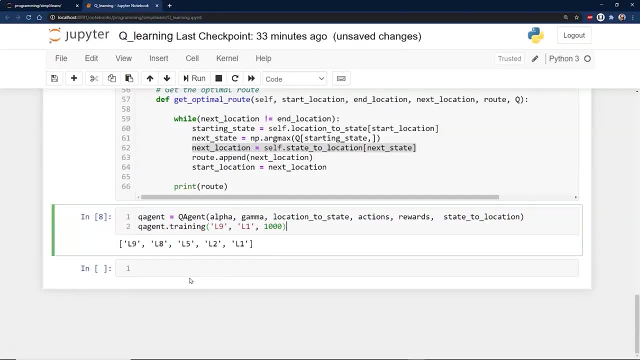 The best course of action, Long as you can take that course of action And reduce it down to a yes, no. Or, if you're using text, You can use a one hot encoder Which word is next. There's all kinds of things you can do with a cue table. 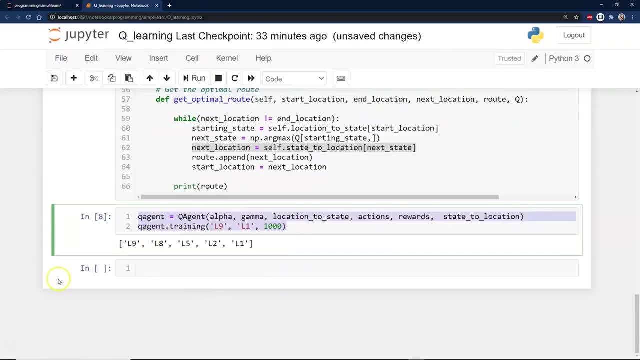 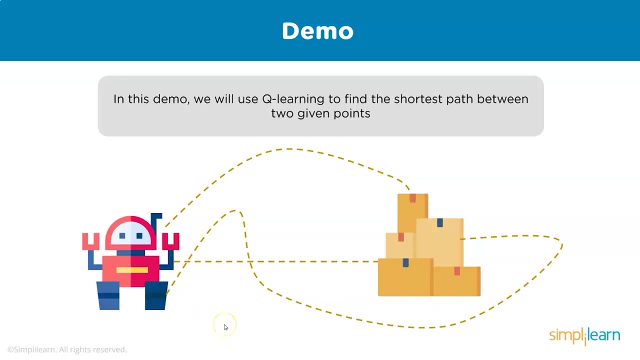 Depending on just how much information you're putting in there. So that wraps up our demo. In this demo we've found the shortest distance between two paths, Based on whatever rules or state rewards we have To get from point A to point B.